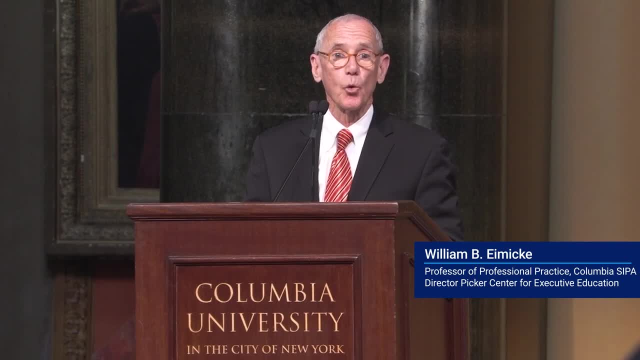 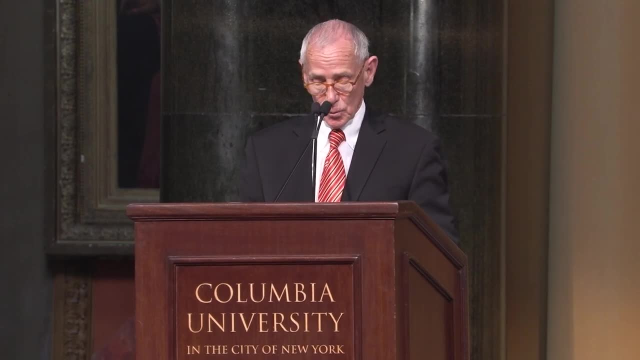 chance to hear about his most recent and, I think, important work. I'm speaking, of course, of Dr Stephen Cohen. He is the Vice Dean of the School of Professional Studies. He's also a professor of practice in the School of Public Affairs here at Columbia, SEPA as we know it, He's the director of the Masters of Public. 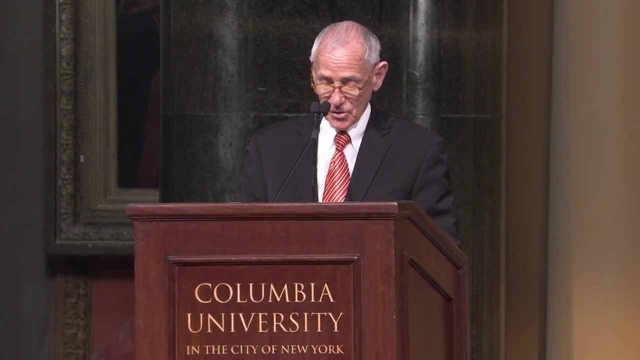 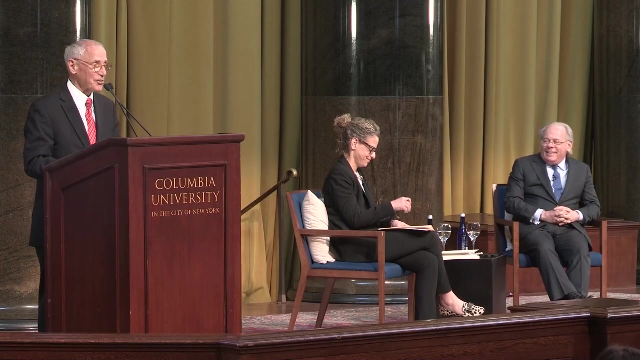 Administration in Environmental Science and Policy at SEPA, and he's also the director of the Master of Science in Sustainability Management in the School of Professional Studies. He also directs the Earth Institute's research program on sustainability policy and management. Just his title takes a full day's work and he actually does the work. 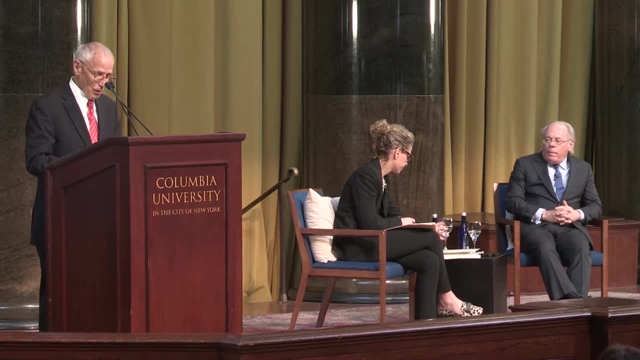 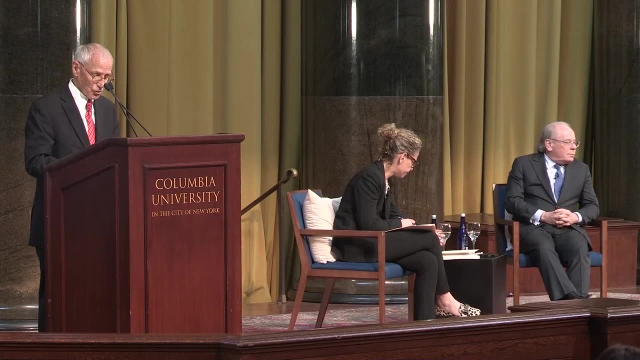 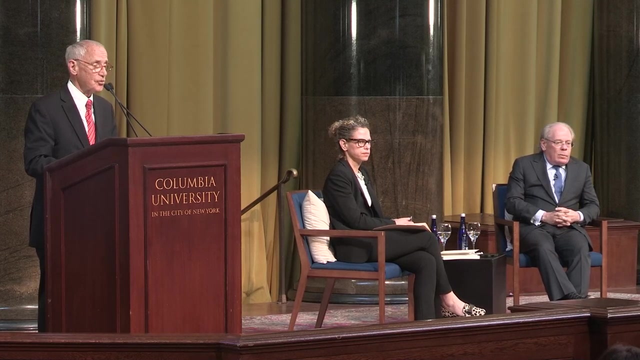 He of course has a PhD, as you well know, but you may not know that he was a Ford Foundation Fellow in Urban Environmental Policy. He was a Rockefeller Foundation Fellow in Public and Environmental Policy and Implementation. He previously served here at Columbia as the executive director of. 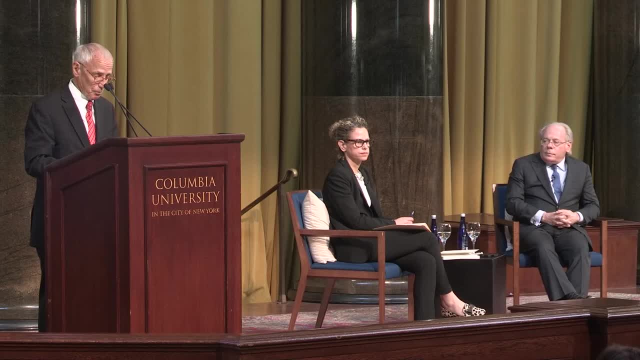 the Earth Institute and he's now a Senior Policy Advisor to the institute. He served as a policy analyst and consultant to the Environmental Protection Agency. He's also worked on numerous boards to this day, including the Pew Faculty Fellowship, the Executive Committee and accreditation community for the National Association of Schools of Public Affairs and the administration. 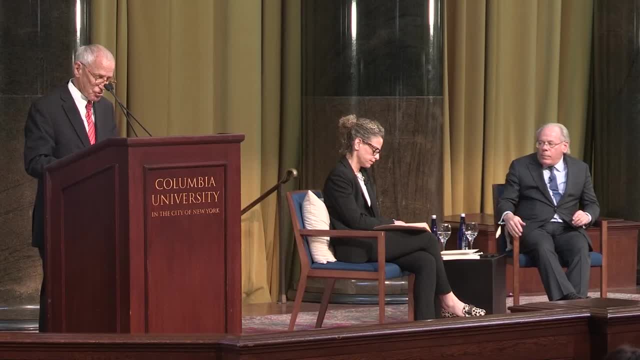 He served on the advisory board of the FEMA in grandpa's bay sign named Robert J beloved university. obwohl eroy eis pulses high school Newsama Sussamy emlogis Eng Ifauelo board of the EPA. he's currently on the board of directors of homes for the 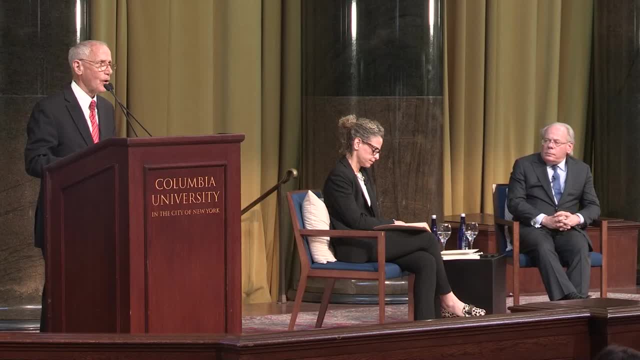 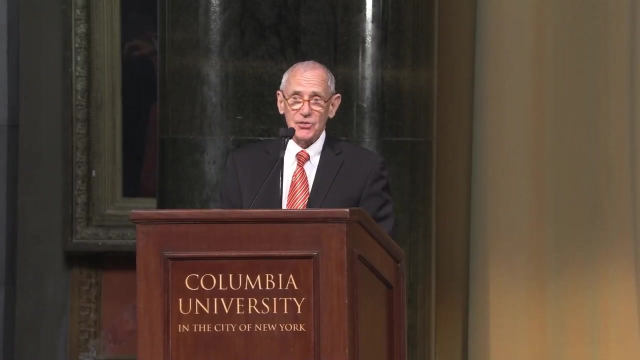 homeless and director of will Dan group, which is a large public corporation that does environmental sustainability issues. he is the author, depending on how you count, of a dozen to 18 books that he's either authored or co-authored, half of them on environmental policy and sustainability and the other half on 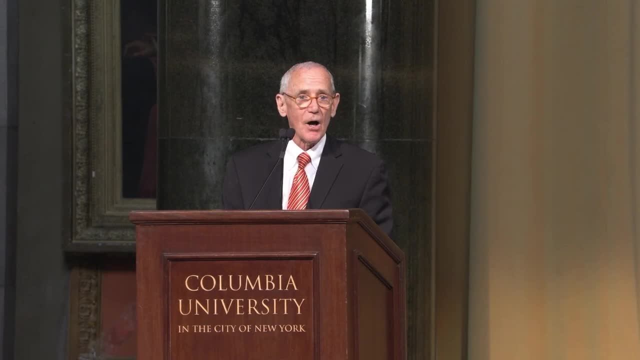 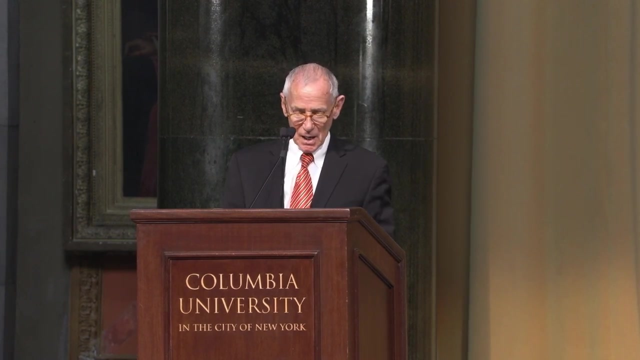 management, and he writes a weekly blog which is a can't-miss. I read it every Monday morning. you should too. it's really useful, and I think the most important thing I can say about Steve is I had the pleasure of reading this book already several times. he- not under, not only understands why we've got 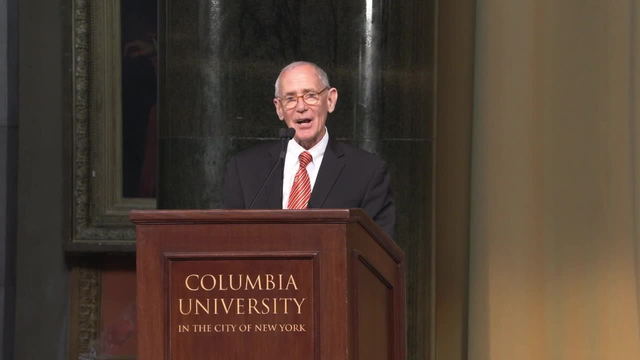 into the position that we're now in, but how to fix it, and how to fix it in a reasonable, responsible way. not that we all have to go back to candles and scratching for a living, that we can have all the benefits that we have in the world today just by doing things differently. and, I think, as importantly, 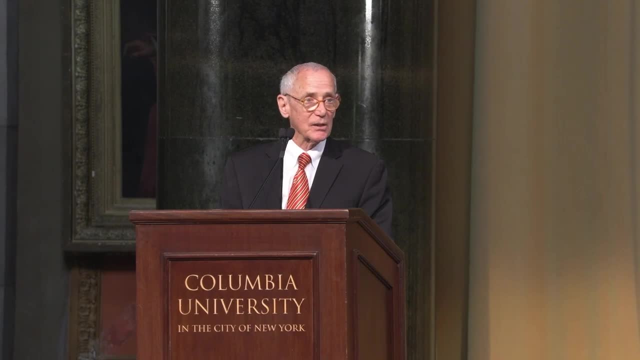 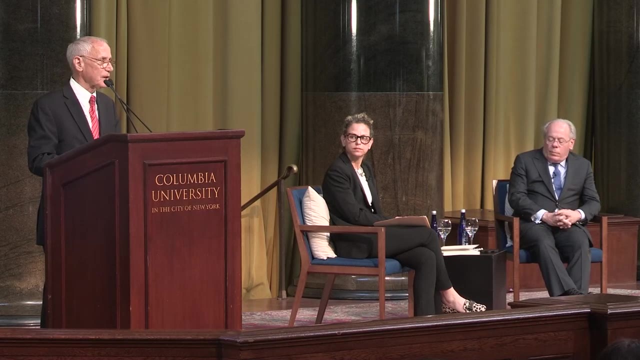 the solution to these issues is not government alone, it's not the private sector alone and it's not the nonprofit. it's all of the sectors working together. so this book is really fabulous, and I say that even though it sounds like I'm pandering. I'm not the first time I read. 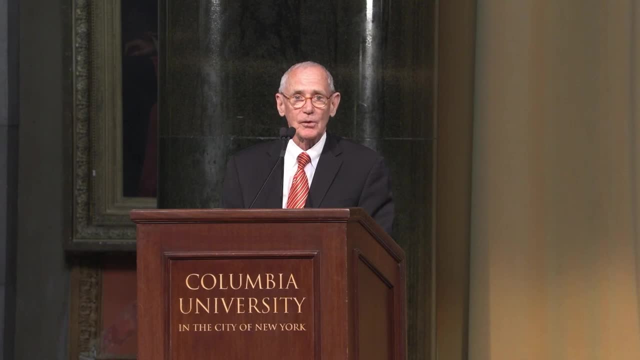 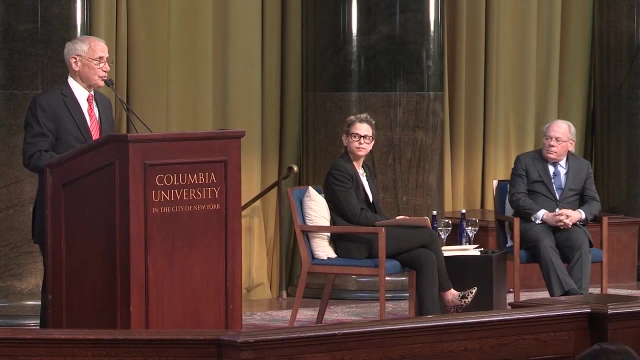 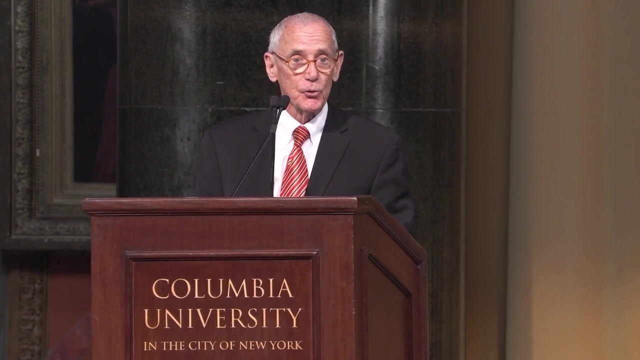 it I. I didn't put it down, I've read the book from cover to cover and I think you'll find it that exciting as well. he's going to be interviewed by Louise Rosen, so we're going to begin with a short film that will introduce you to the book, and then the two of them will go at it. so thank you again for. 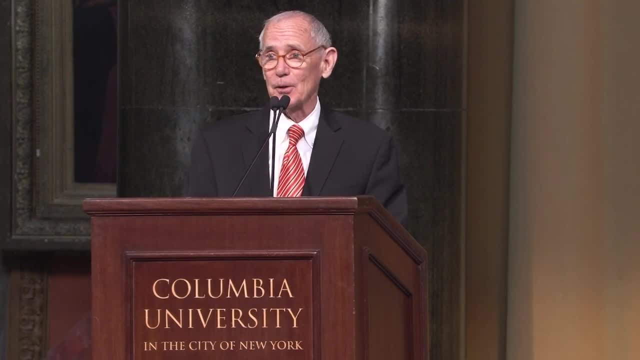 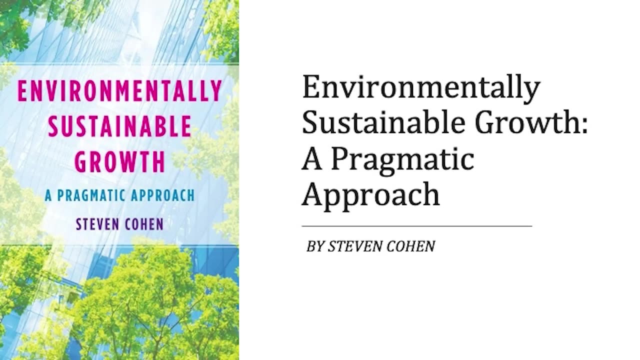 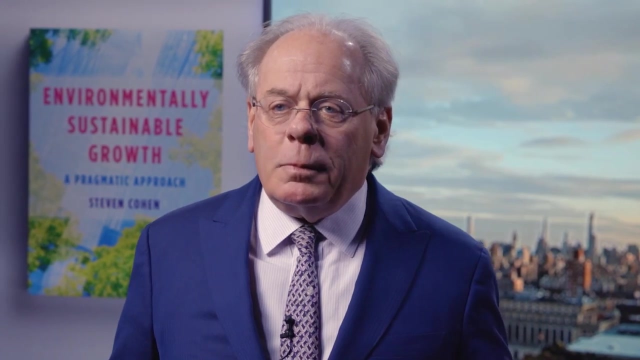 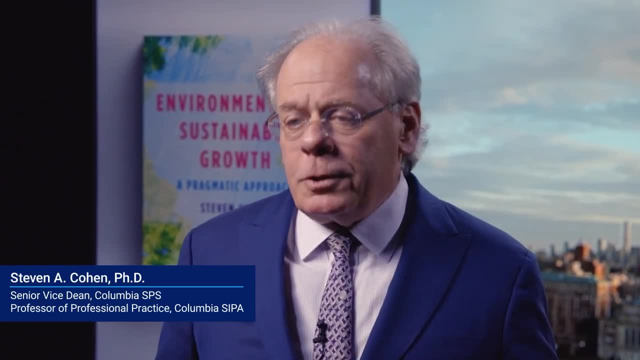 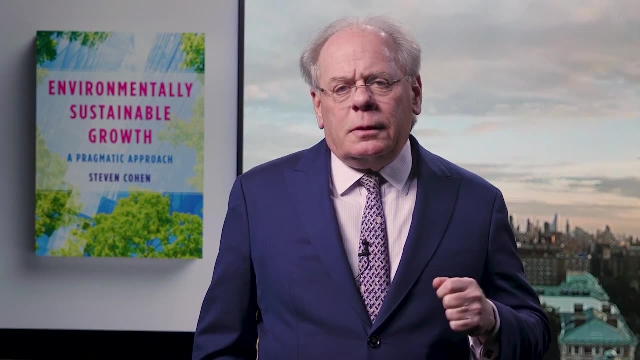 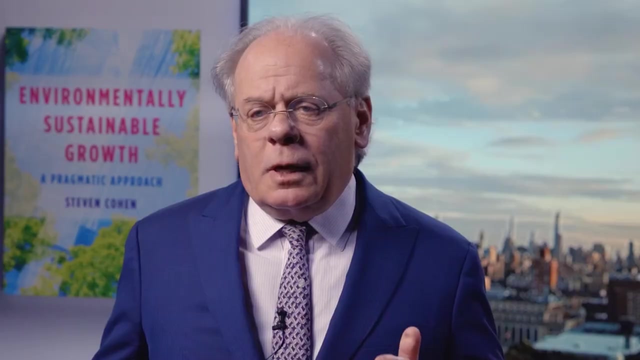 throw out all of our material possessions to what's called a circular economy, where every thing that goes in uh eventually comes back and gets reused. I want to, in a very straightforward way, explain how we got into the environmental and sustainability crisis we're in today. I start by looking at 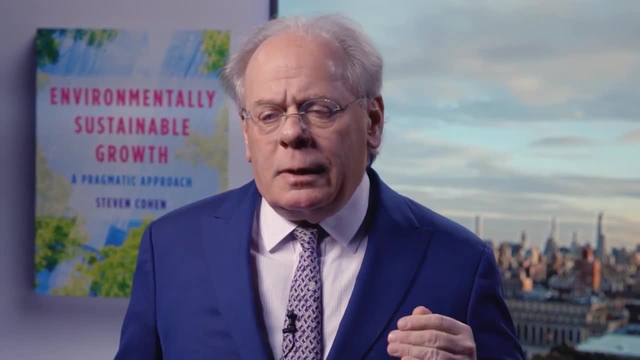 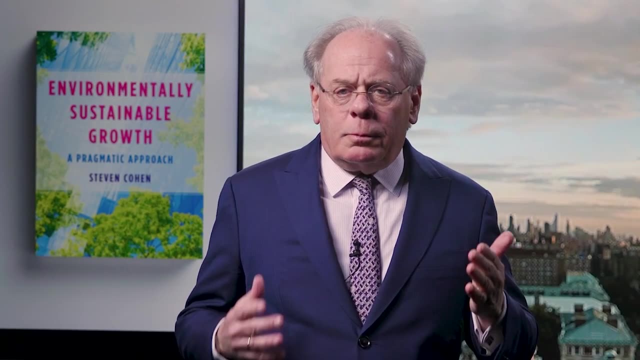 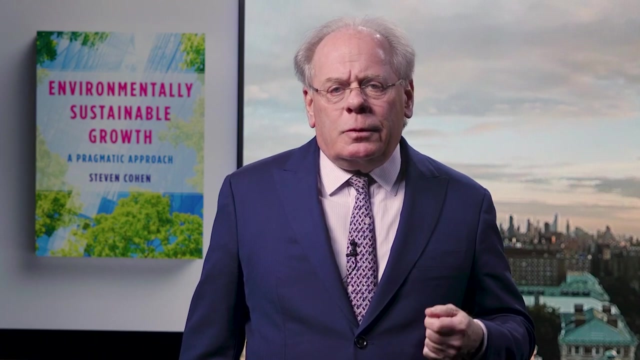 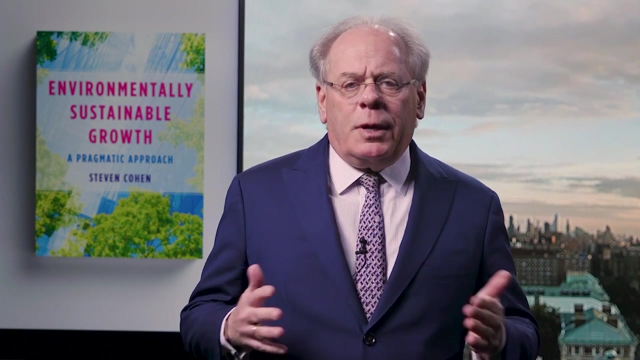 what are the forms of pollution that we have? what causes them? then I turned to a strategy for addressing those problems And I conclude with a discussion of the politics of environmental sustainability. Environmental activists want people to do without. They want to punish people rather than trying to figure out ways of creating positive incentives for moving from the way. 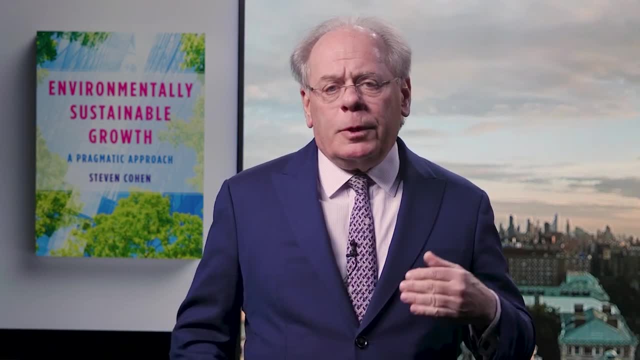 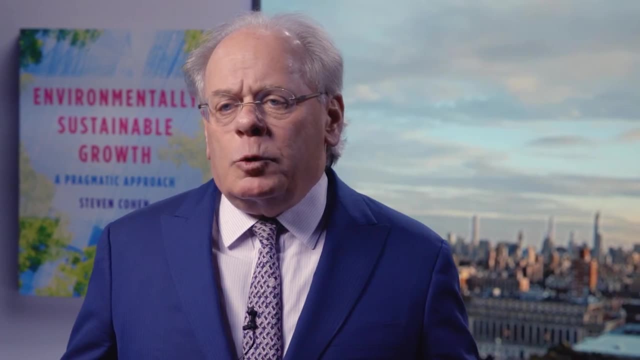 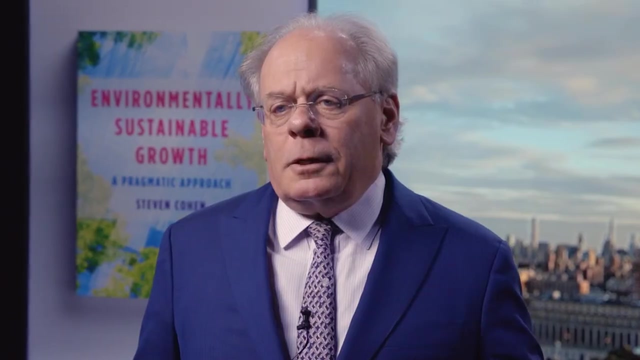 we live today to the way we need to live to be in greater harmony with the planet, And so I focus on what's better about having a renewable resource-based economy. Rather than focusing on just the issue of renewable energy, I like to focus on the issue of modernizing. 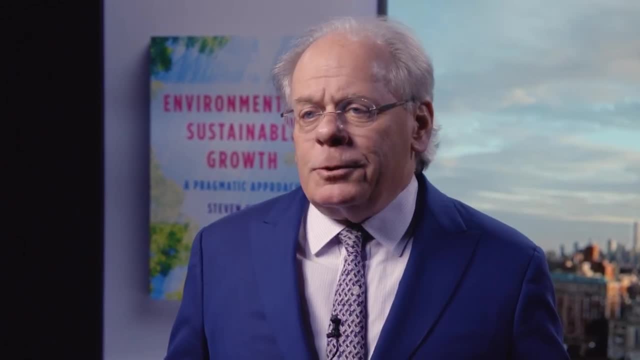 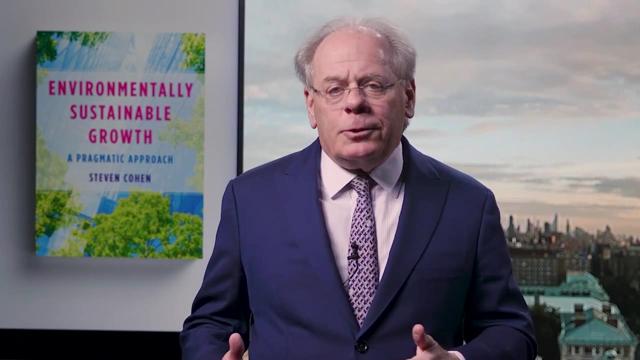 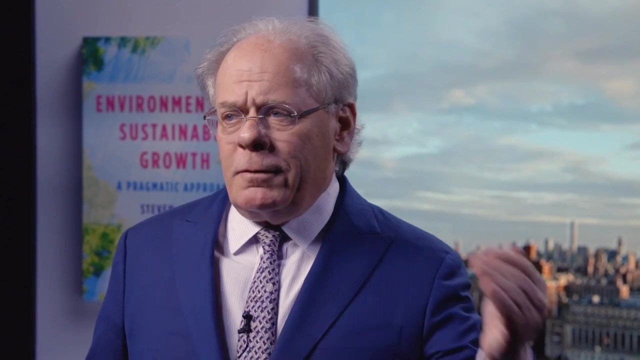 our energy system and trying to lower the price of energy, rather than figuring out ways of taxing people so they move from fossil fuels to renewable energy. Fossil fuels have to be dug out of the ground or pumped out of the ground. That pollutes, That costs money. Then they have to be shipped. That pollutes And that. 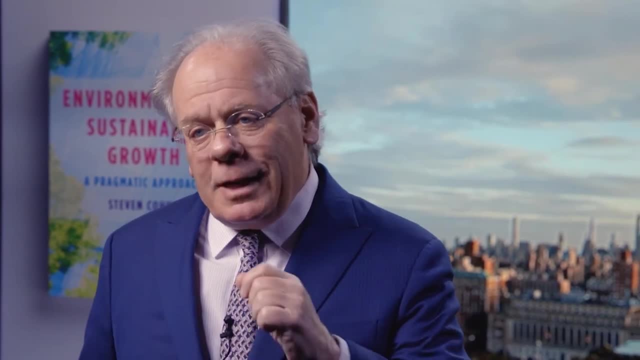 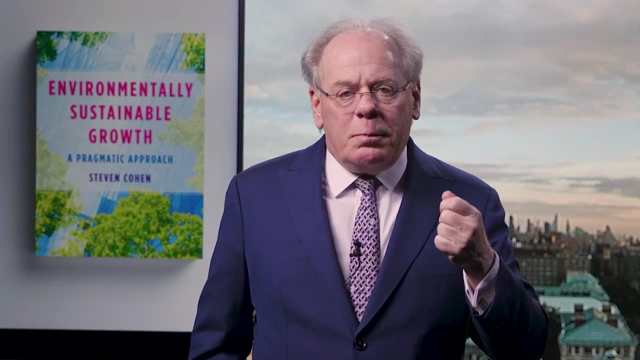 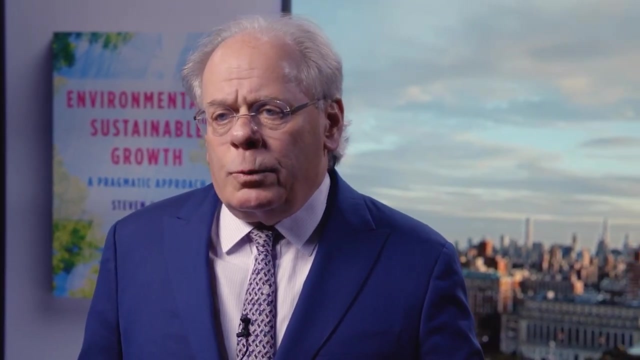 costs money And then they have to be burned. That pollutes And that costs money. Taking solar power and turning it into electricity is getting better and cheaper every year. We're going to see more and more use of renewable energy, And it's going to get to the point. 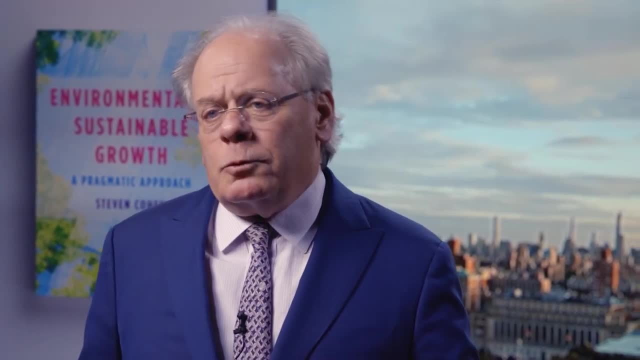 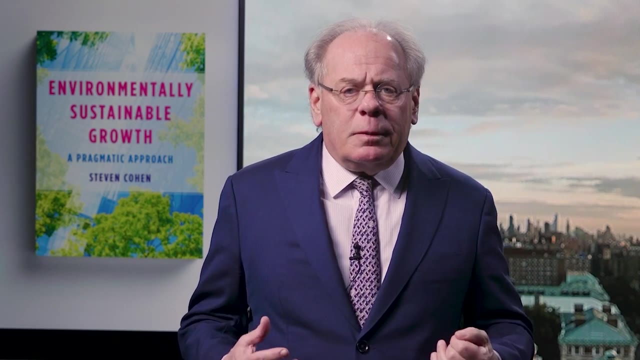 where it's so much cheaper than fossil fuels that fossil fuels will be literally driven from the marketplace. We need to. We need to deal with people where they are instead of trying to convince them that they have to do without in order to save the planet. And I think the other issue that I raise in 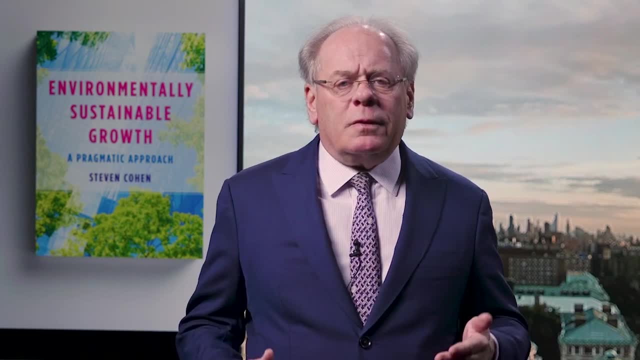 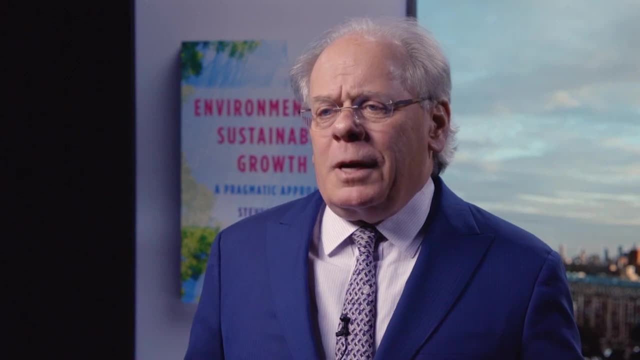 the book is the need to go back to the consensus politics of the 1970s, which is when all the great environmental bills were passed in the United States, And I think too much of our politics today is really about separating and polarization and showing how different 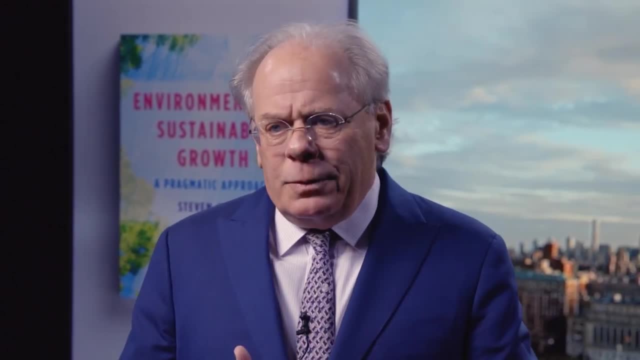 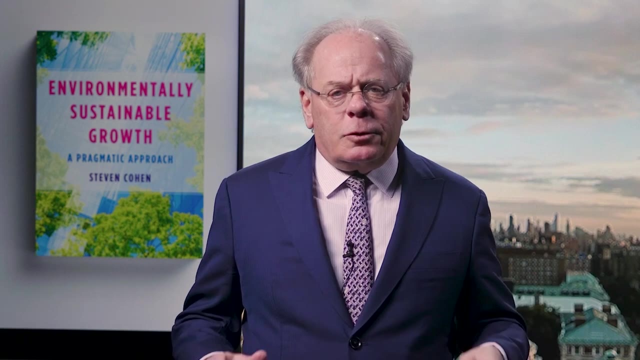 and better we are than other people, And I think we have to go back. We have to go back to a politics that talks about what we have in common. There's no reason to have the kind of ideological split we've had on regulation. Instead, we can develop. 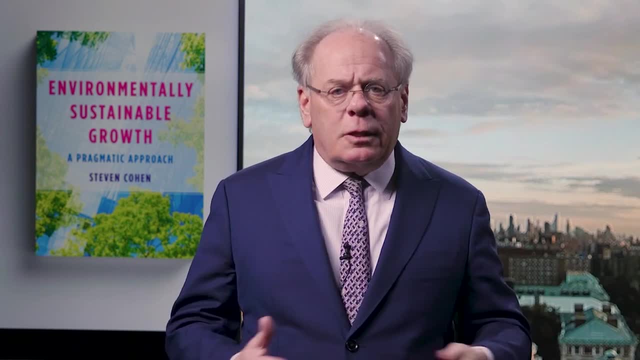 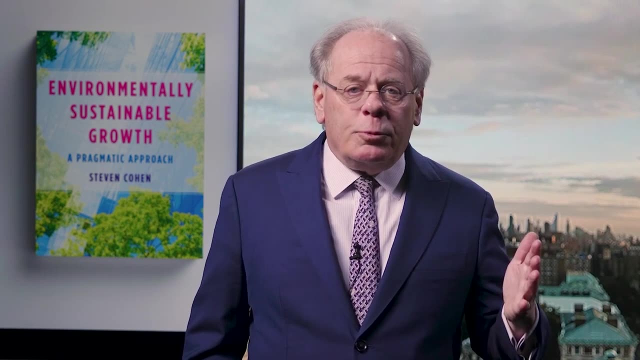 as we did at the beginning of the environmental era, a consensus politics. Now, some people consider that naive. I consider it essential, And the way I always put it is: we all like to breathe. It's one of those things we get used to And we need to build a politics around. 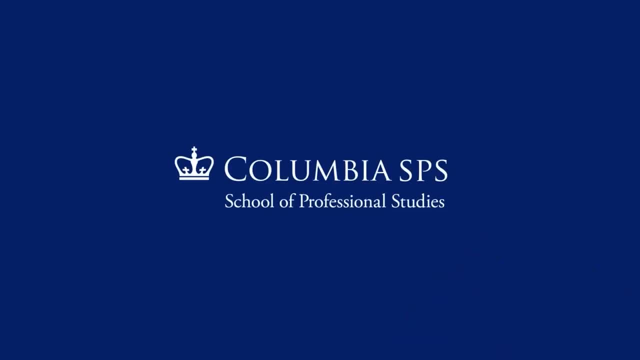 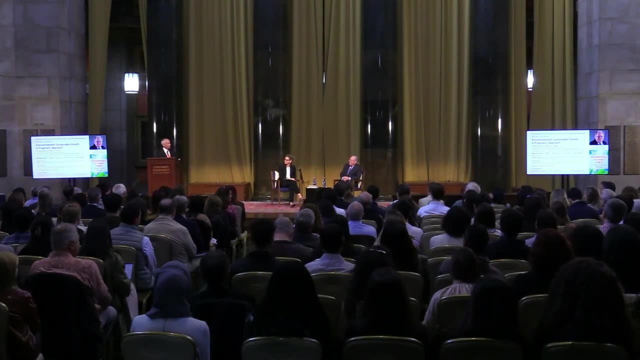 that common need that we all have. Now you get to hear directly from the man who made the video, Luis. I'll turn it over to you. Thank you, Bill. Steve, thank you for this opportunity to talk to you about this. 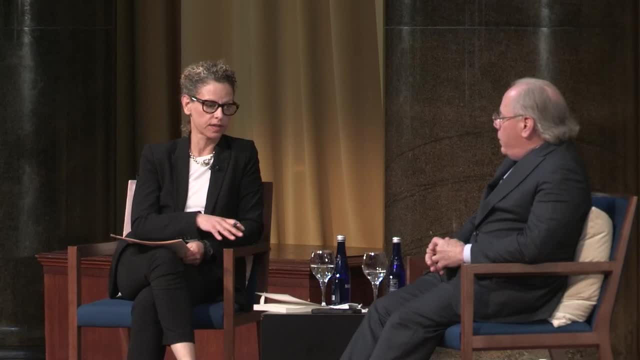 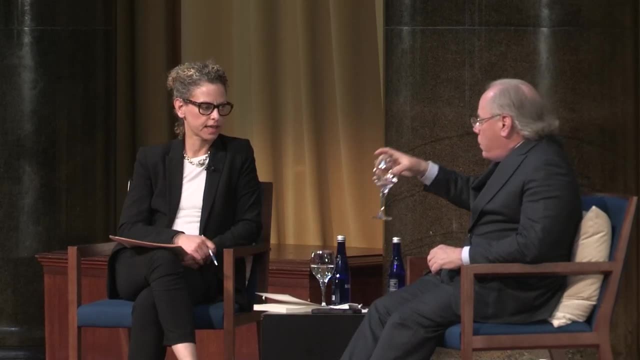 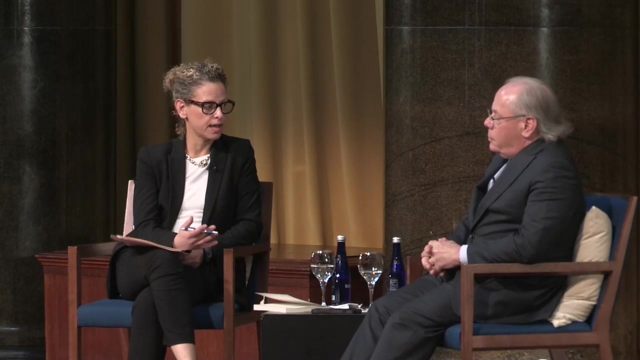 book. I think one of the things that grabbed me about this book, and that you mention in the video, is it's the can-do attitude and the optimism that carries from the first page end. so what inspired this optimism and what enabled you to write this book at? 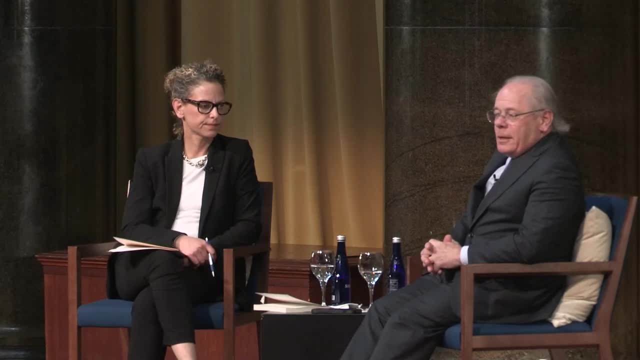 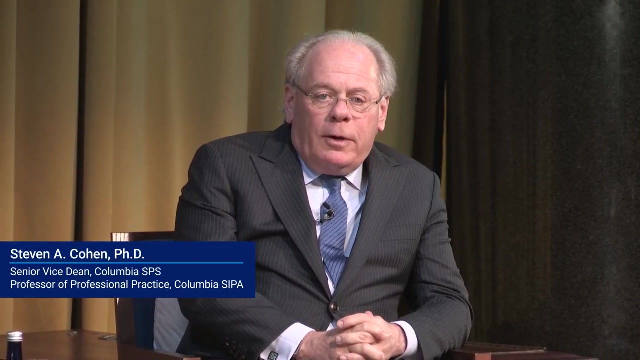 this moment in time. thanks. you see the extremes they went to have me not do a lecture. I think it really goes back to my first engagement with the environment. so it's the fall of 1975 and I wander into Les Milbrats environmental policy class and got interested in this, worked at EPA in the water and 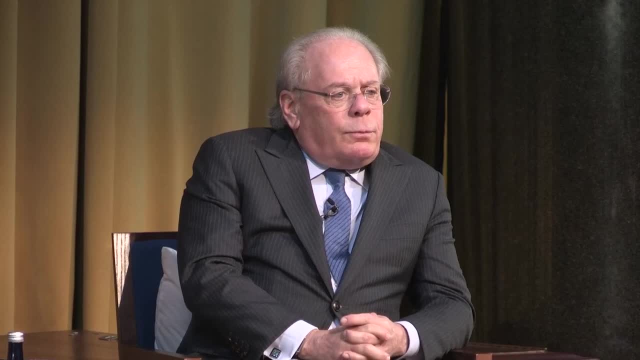 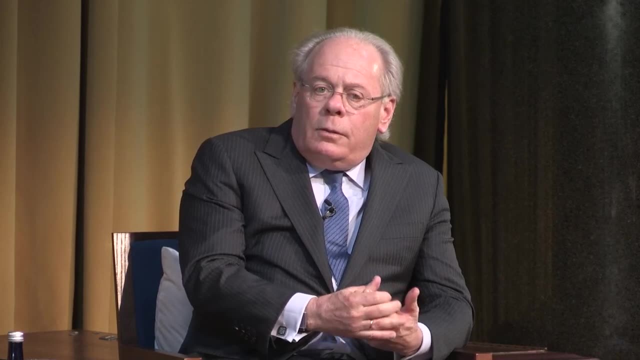 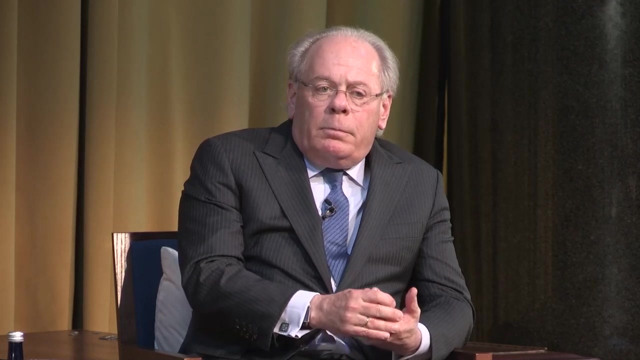 Superfund program in the late 70s. I realize that's four decades ago. and guess what? the air in America is cleaner today than it was in 1970. the water today is cleaner than it was in 1970. we got 40 million people out of pathways of. 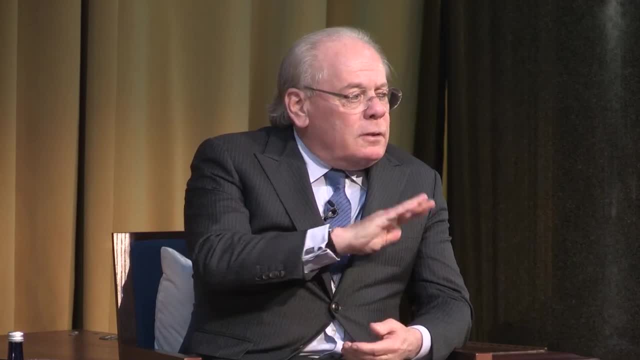 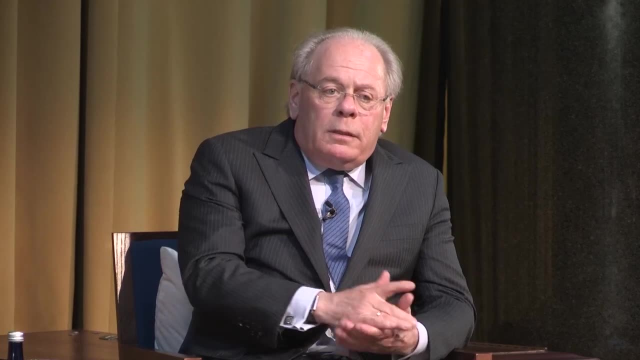 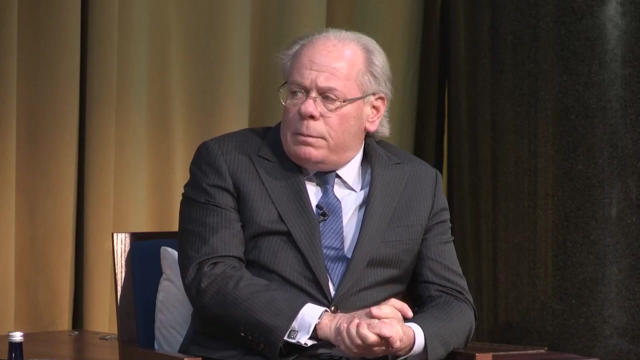 exposure to toxic waste. that didn't prevent East Palestine. it's not the world's perfect. public policy makes problems less bad and the environment is less bad than the environment is less bad than the environment is less bad today than it was in 1970. now we we have huge, important problems to address. 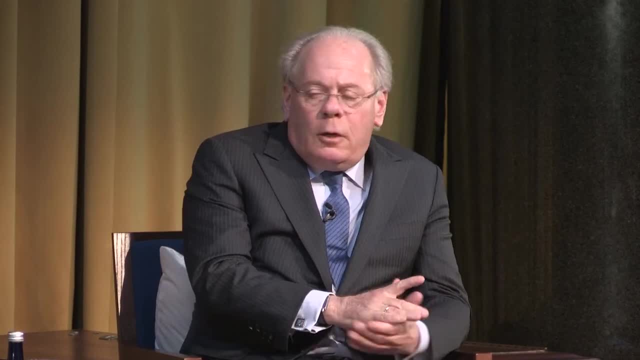 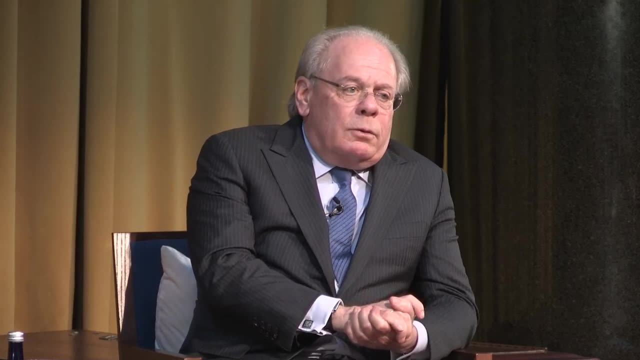 but the question is: what is it that we did in the past that helped us solve these problems, and then how do we apply those solutions to what's going forward? and so the reason I'm optimistic is that I really believe that we've made progress and that we're going to continue to make. 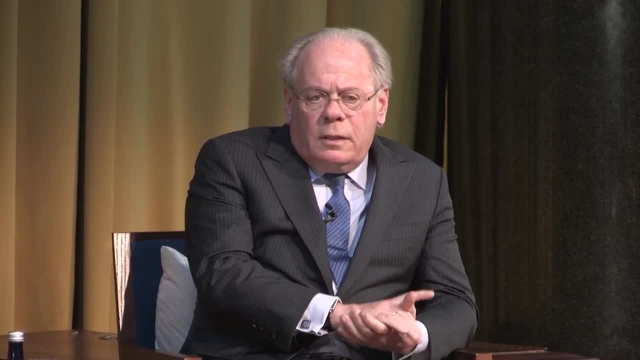 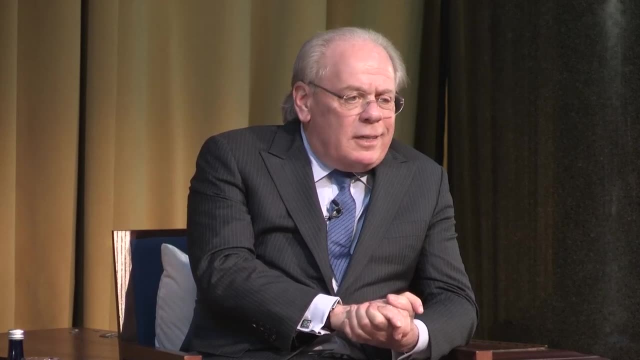 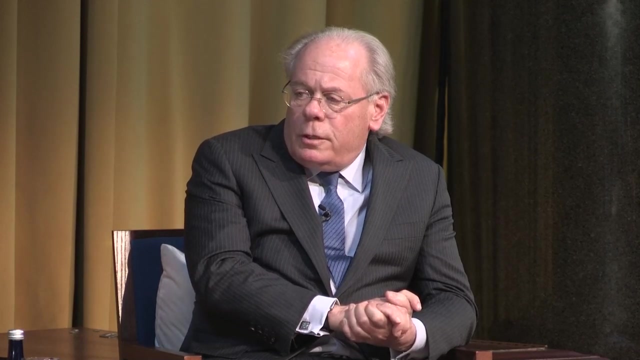 progress, and I think that one of the things that I say in the book is that I the transition to a renewable resource-based economy has begun And, like a lot of these transitions, when they start you don't notice them because you're still enmeshed. 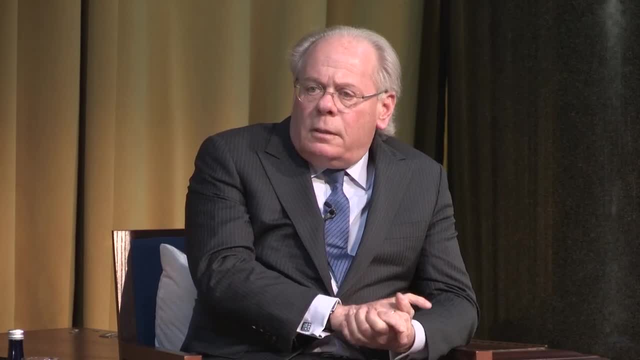 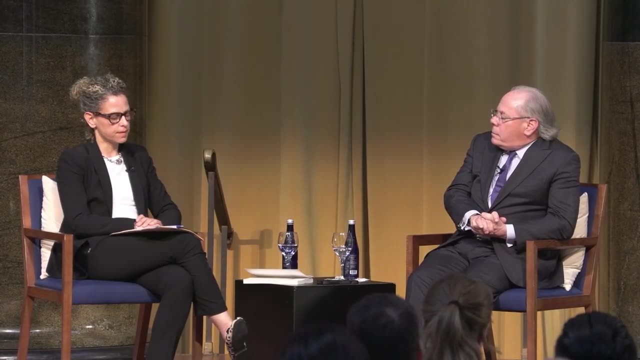 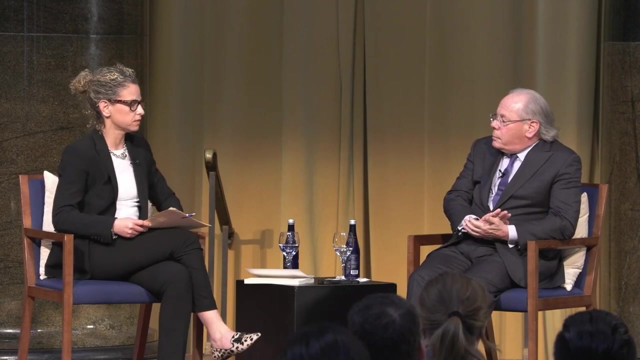 in the problems of the old era, And I think that's part of what I'd say is what keeps me optimistic about things. One of the things that you mention both in the book and that anybody who's reading the news at the moment can see that there's still degradation. 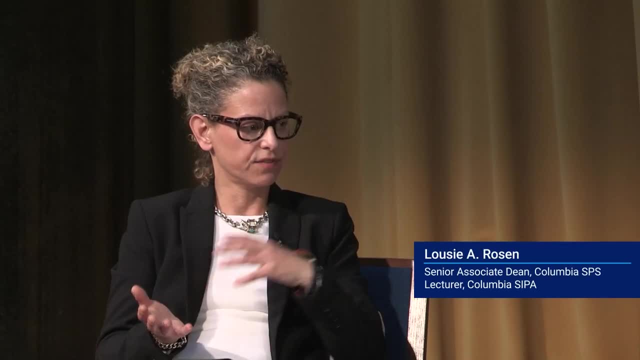 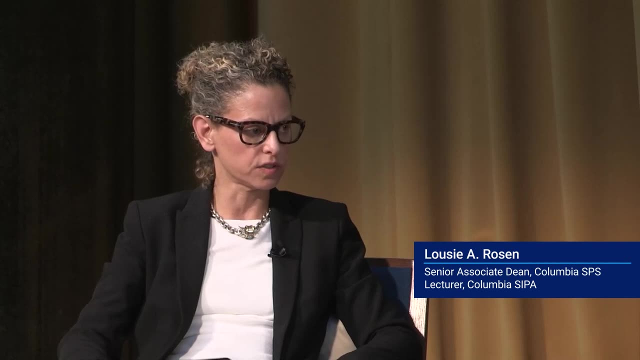 that's going on? Is the degradation that we're seeing today different to what we had seen previously? I mean, all of us were degrading with very little choice not to. So what's driving it today? What are the main causes of it today? 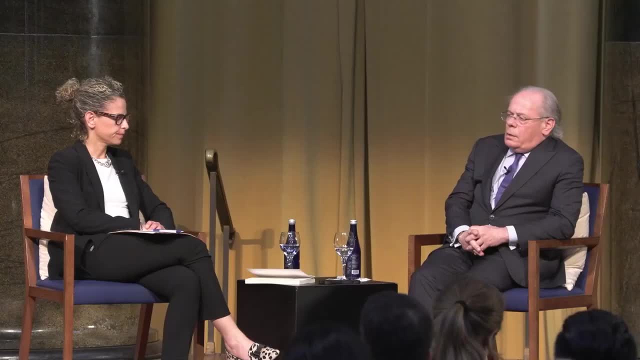 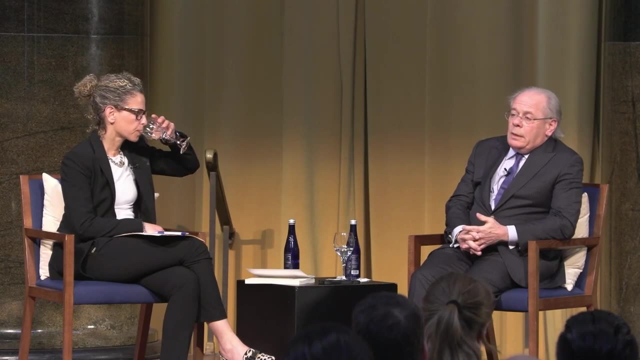 if there's so much possibility to eliminate it. Well, at the beginning of the environmental era in the 70s, we had a little bit more than four billion people on the planet. Now we have about eight billion people And the rate of consumption 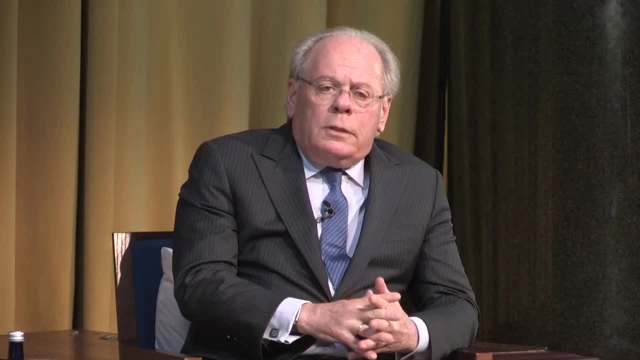 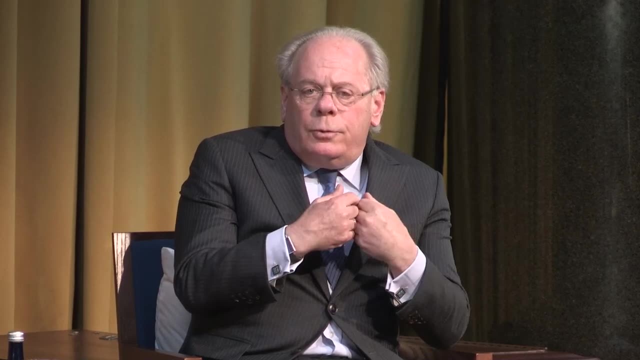 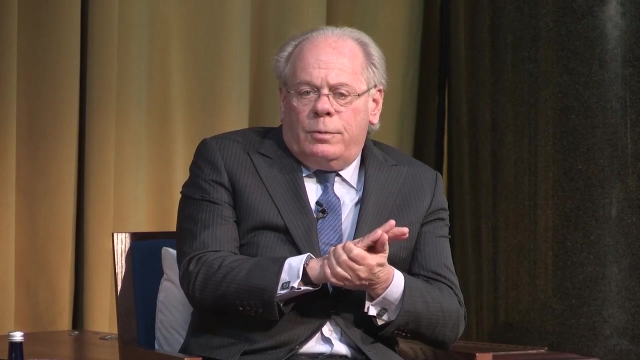 of material consumption has grown. So the question is really: how do you take that consumption and build it in such a way that, as you consume, you don't destroy the planet? And part of it is just good management. You know, I taught a case study in class the other day. about Cancer Alley, which is a terrible set of chemical plants, mostly in Louisiana, And the people running those plants should be ashamed of themselves, Because their management of those plants allows all sorts of toxics to escape unnecessarily. You don't have to poison the planet. 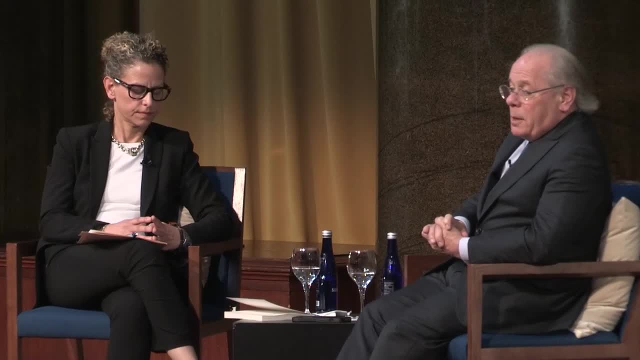 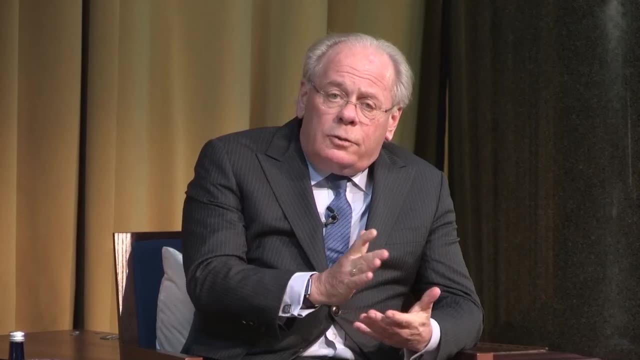 to make chemicals and plastic. It may be a little easier, it may be the way you know how to do it. but with a little bit of ingenuity, a little bit of ecosystem consciousness, you can actually fix it. And we have lots of examples of organizations. 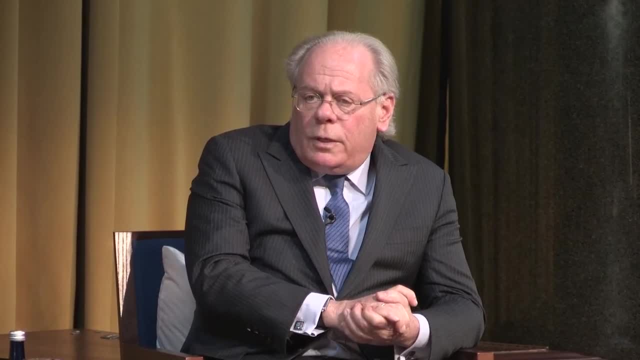 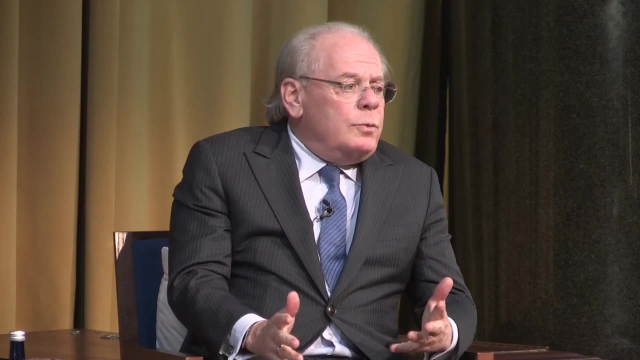 that have done that, And so I think that's really the. the question is: how do we become more mindful about our production and consumption so that, as we produce and consume, we don't destroy the planet? You, you know we're living in a time at the moment. 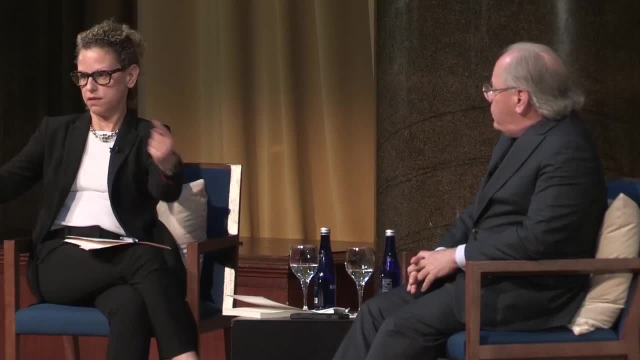 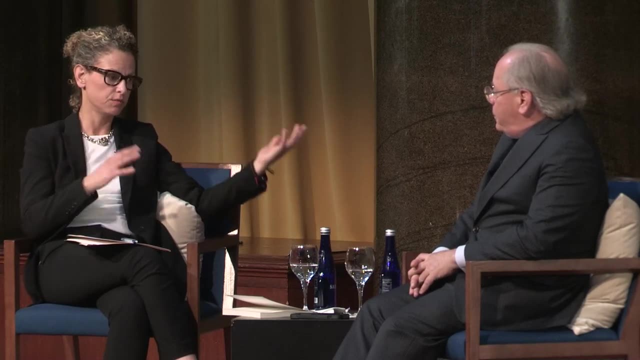 where there is just it seems very difficult to be able to see relationships being bridged across the divide. It also depending upon which publication you read or what radio station you listen to. government is evil, regulation is evil, And you're not saying that. 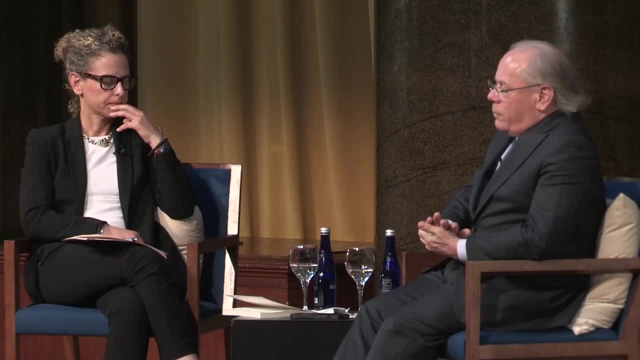 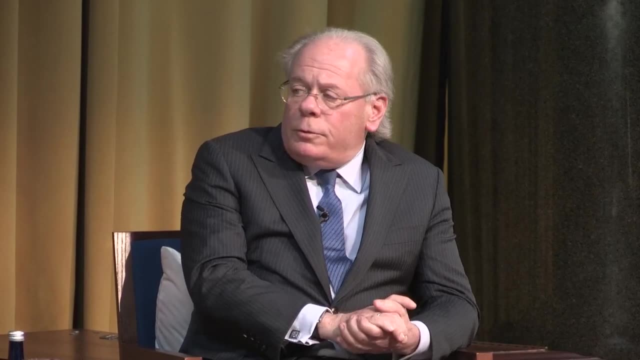 You're saying that in this book? Why? Well, first, unfortunately, our politics is a monetized difference. You know, because of the way people raise money for interest groups, you tend to paint your opponents as if they're evil and enemies. 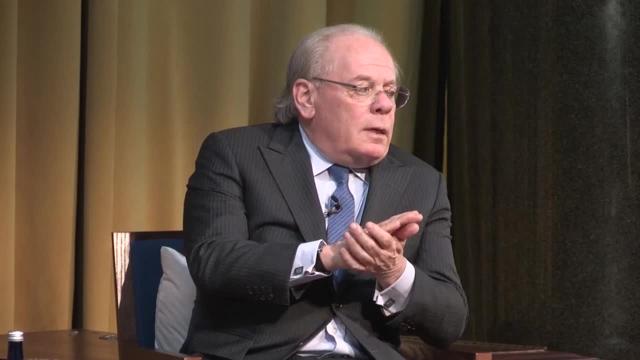 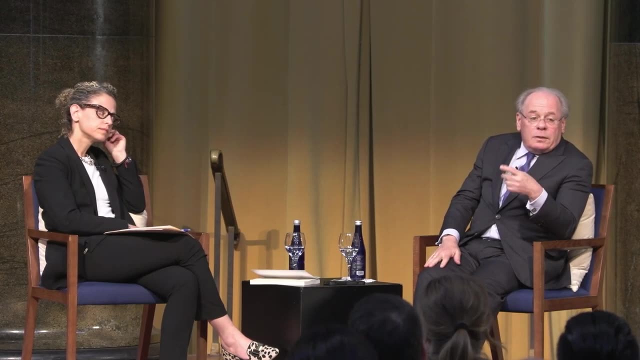 And so there's less of a drive to try to figure out what's common ground. And if you look at the beginnings of the environmental movements in the 70s, what's the largest environmental interest group in America To this day? it's the National Wildlife Federation. 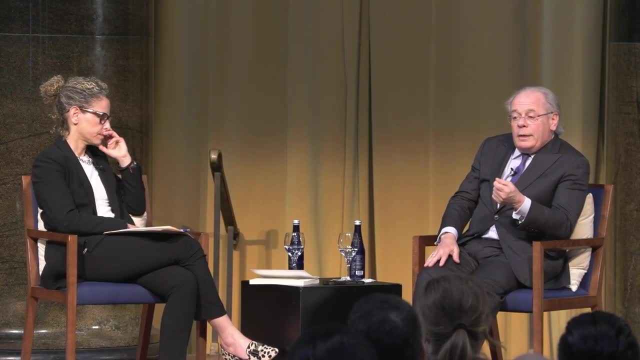 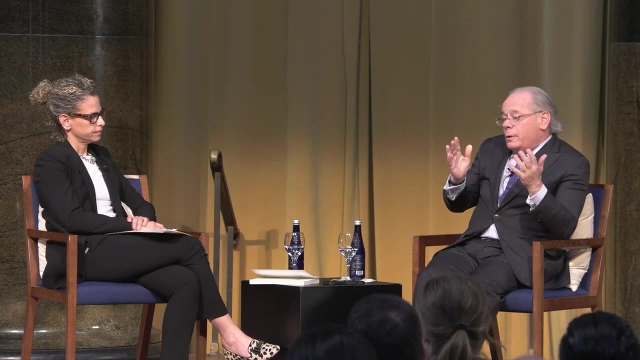 The National Wildlife Federation was formed by, and is still largely populated by hunters and anglers. Why do they care about the environment? Well, sort of like Teddy Roosevelt, when he and John Muir were were uh, trooping through the woods in California. 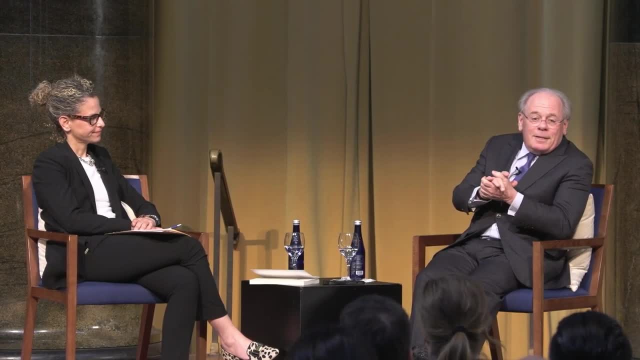 He liked to shoot things, He liked to shoot animals. That was his thing, And so hunting, uh, requires a certain amount of preservation. Okay, So what do they have in common with urban environmentalists who are vegans and are are? 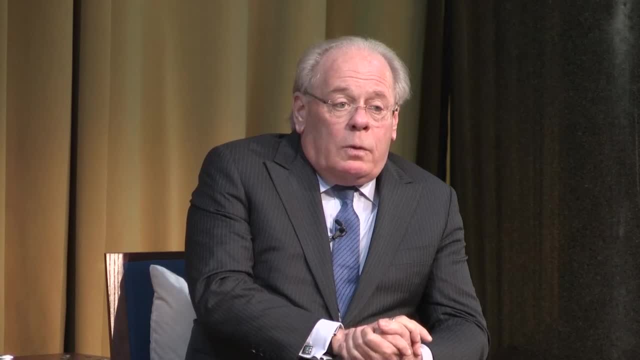 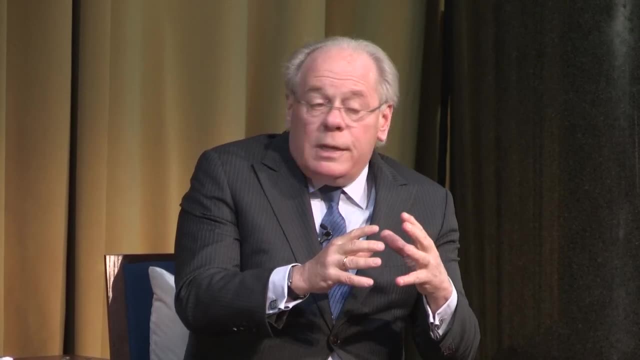 I can't believe people would wear fur or eat meat. Well, they all breathe and they all want clean water, And so there's actually a point that we can agree with each other, And so our politics has to go back to that kind of agreement. 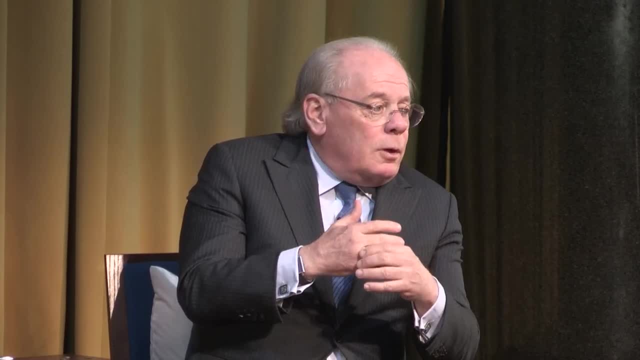 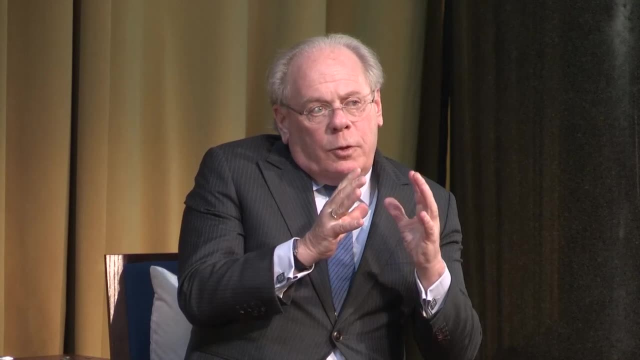 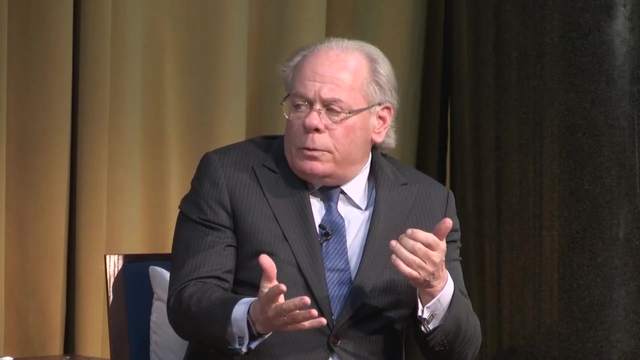 And climate change is the same way. Climate change- nobody wants to be underwater, Nobody wants to be in a planet with extreme weather all the time. So you know, there's been this effort to delegitimize the science And that's in part because the solutions being proposed are so extreme. 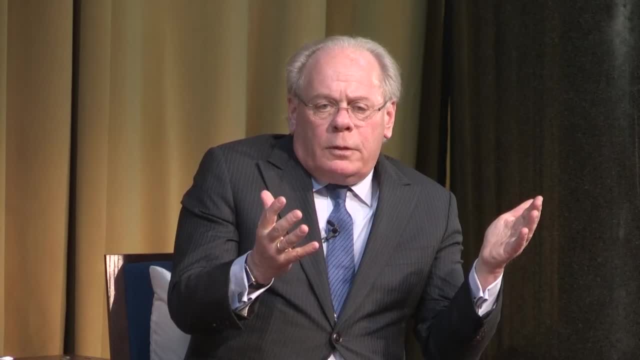 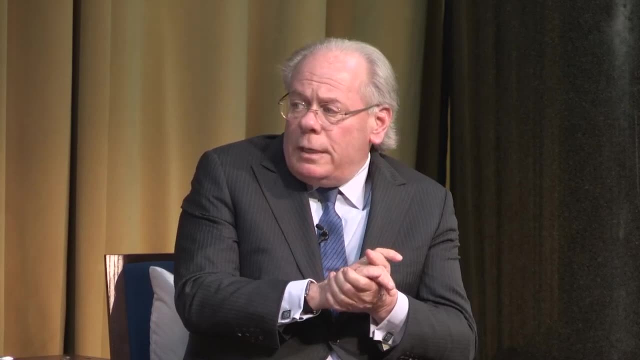 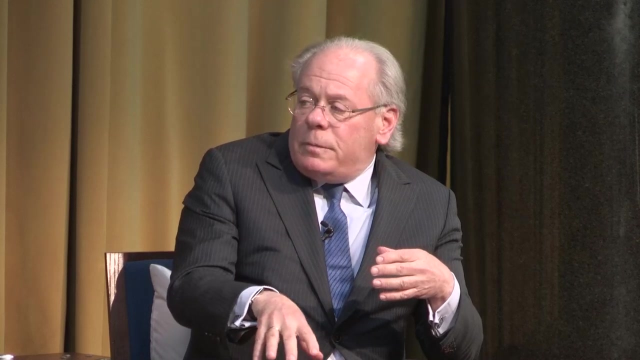 You know, the only way to solve the climate problem is for us to not fly and not drive and sit alone in the dark with a candle. Well, you know, good luck in selling that. What I would rather sell is an energy solution where I say we're going to modernize the energy system. 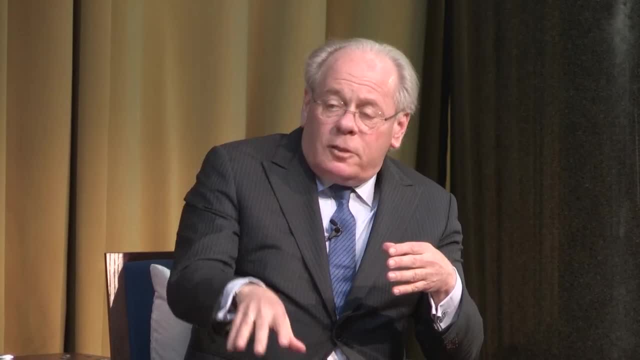 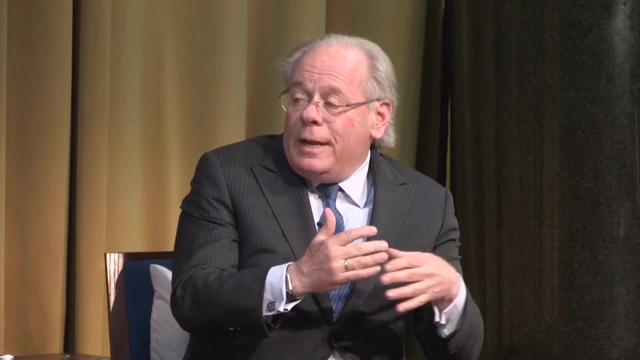 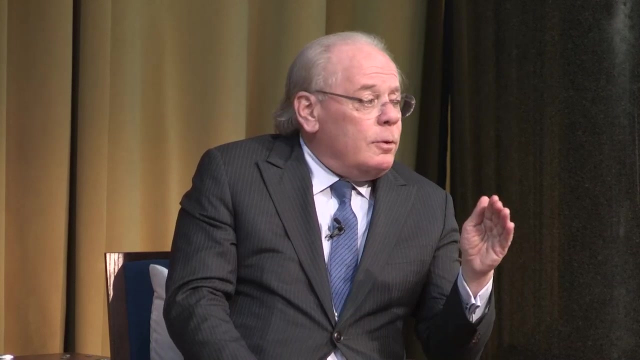 We're going to make energy less polluting, less expensive and more technologically superior and reliable, And that's exactly what's happening right now. That's what we're at the beginning of doing, So that solution works on greenhouse gases much more effectively than trying to convince people. 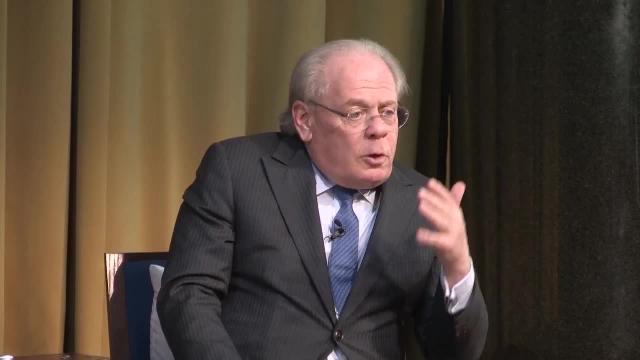 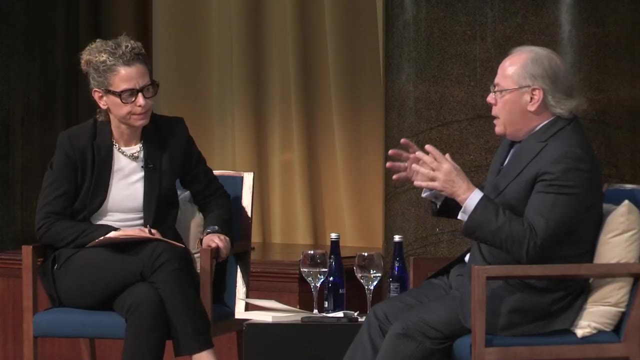 to give up their lifestyles, which they're not going to give up. So so much of environmental politics. is this position-taking and symbolic nonsense, as opposed to trying to figure out a way? how do we find out what's common so we can work on these problems and really solve them? 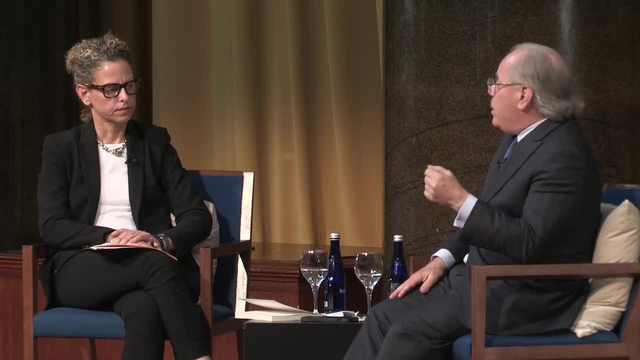 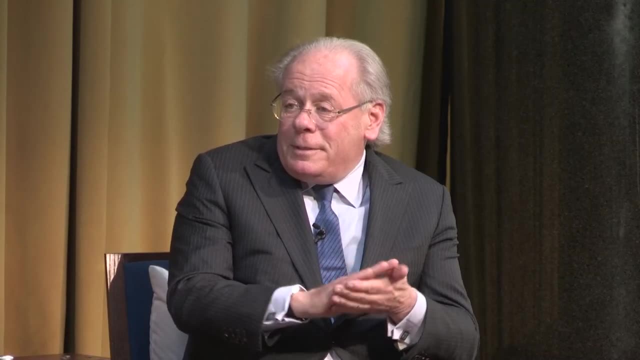 And in the past that's how we did it And that's what worked, And I would like to go back to that now. People tell me I'm naive and unrealistic, But, like I said, everybody wants to breathe. It's sort of one of those things we do get used to. 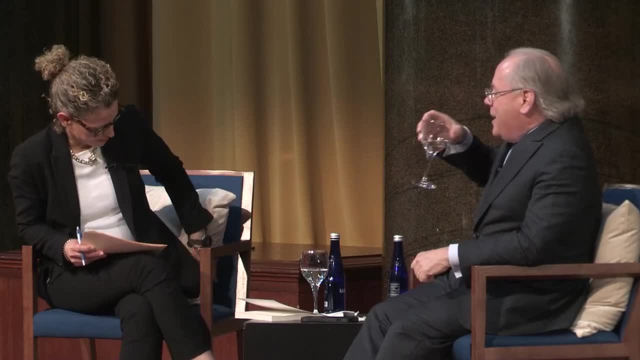 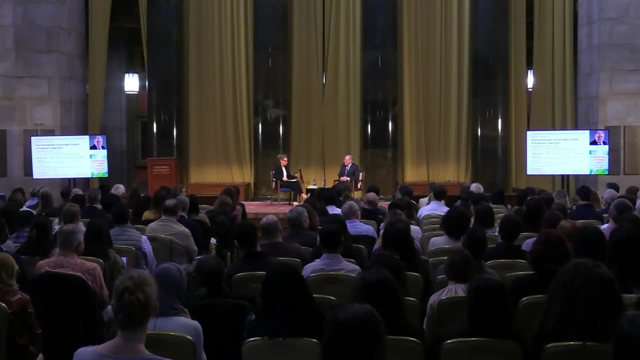 I would never say that you were naive or unrealistic. You're my boss. I would put it in a different way completely. But one of the things that is very compelling also is- and just to pick up on what you just said- you mentioned the role of hunters. 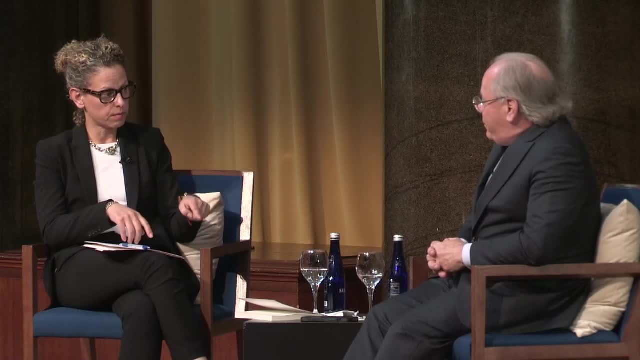 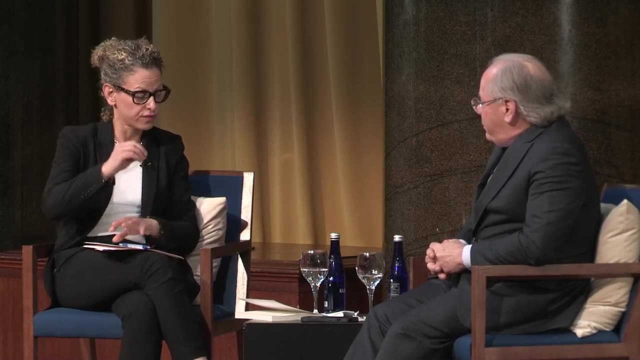 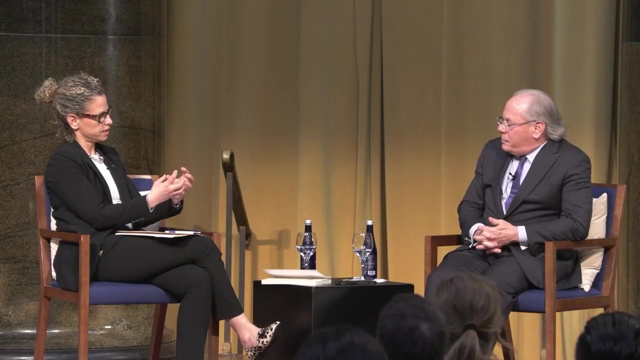 The role of anglers. You also, in the book, mention the need for organizations to take the lead- and take sorry for organizations to follow the lead of equity and environmental justice. So and this Genghis Khan-like approach of bringing the disparate tribes together. 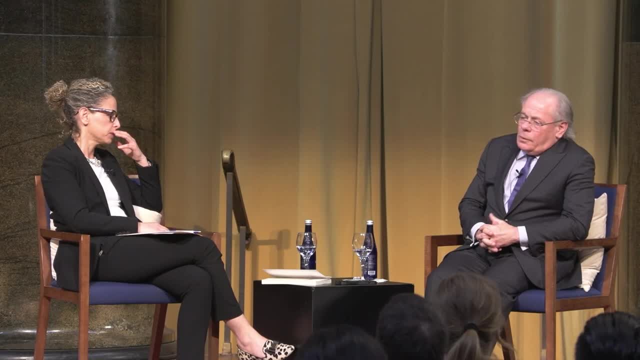 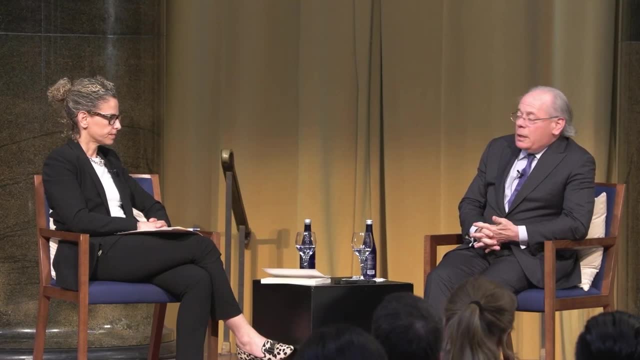 How does that happen And do you have any examples of that at the moment? Well, I looked at Mike Bloomberg when he was mayor of New York and he brought the real estate industry and environmental justice advocates into the same room And said: you know, what is it that we need together as a city? 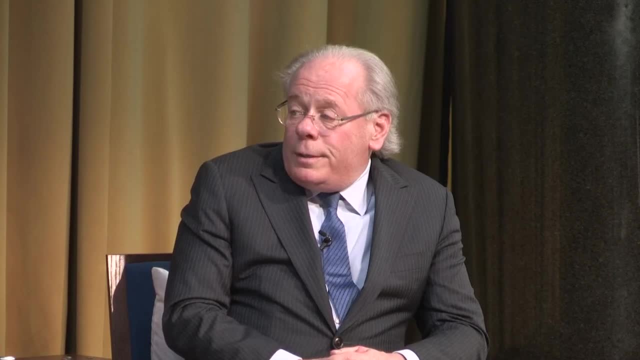 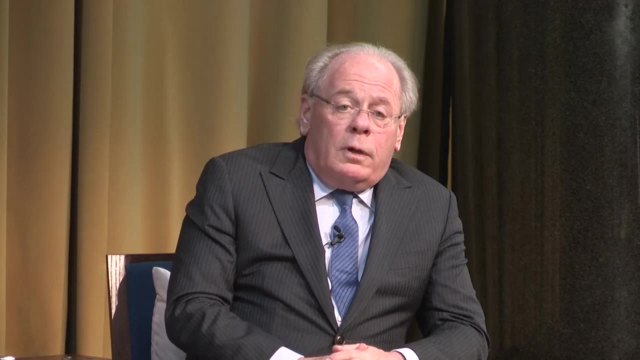 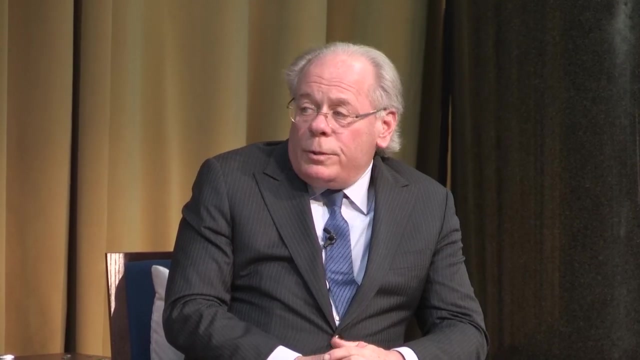 So goals, like everybody, should be within a 10-minute walk of a park. That when we build new developments, some proportion should be set aside for, you know, below market rents, That we need to modernize our water system in building the third water tunnel. 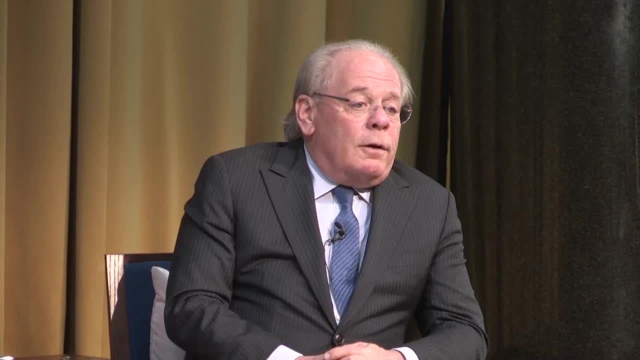 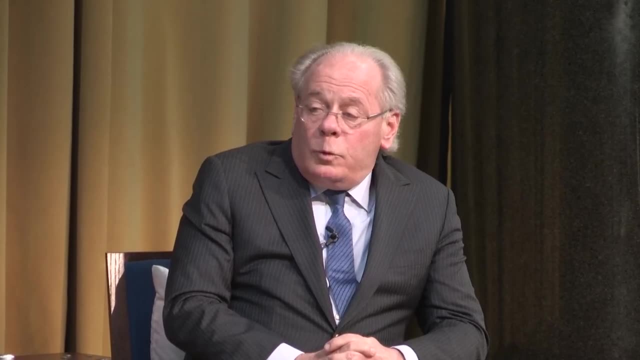 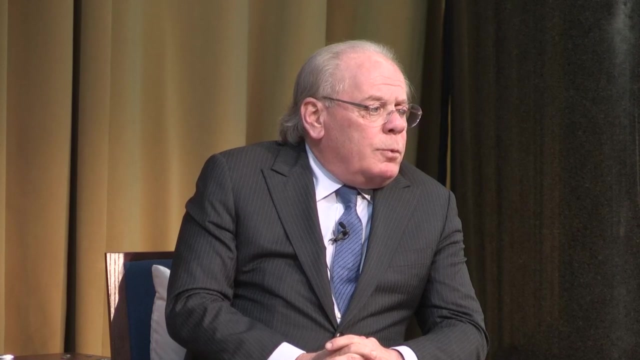 That we need to come up with congestion pricing and other ways of funding mass transit, And it was early days, But I think since then he's been focusing a lot on renewable energy and advancing those technologies, But directing the benefits as much as possible to people who are suffering the most from environmental degradation. 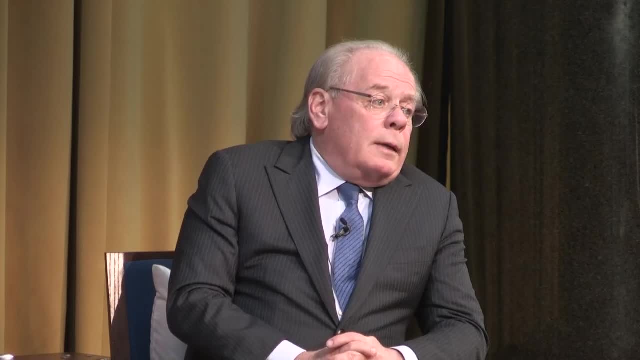 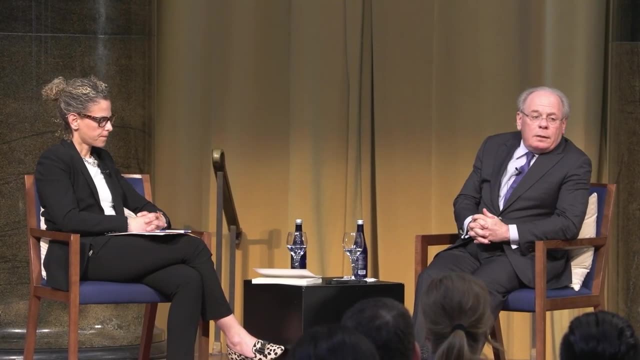 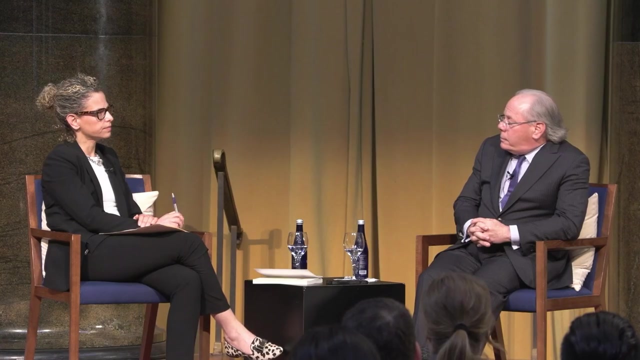 And those are largely communities of color and poor people, And so we have this opportunity to rebuild the energy system. We could, at the same time, use that opportunity to also fulfill some of the goals of the environmental justice movement. Do you think the government is better than at prohibiting pollution or fostering innovation? 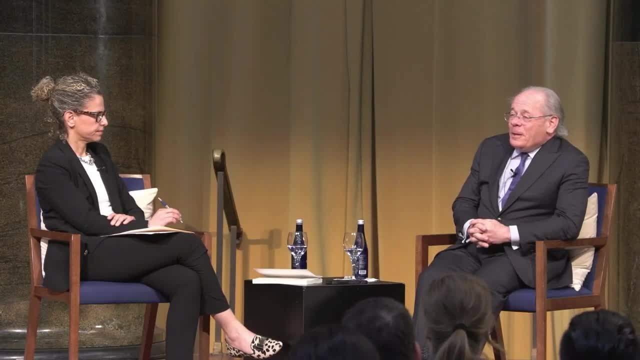 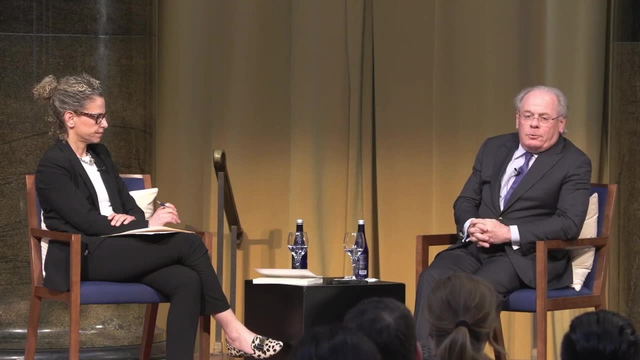 Well, interestingly enough- I mean, this was actually part of my blog this morning- It turns out that regulation inspires innovation. Now, I know that that's the opposite of the rhetoric. you know, job-killing regulation, But I use the automobile as the example. 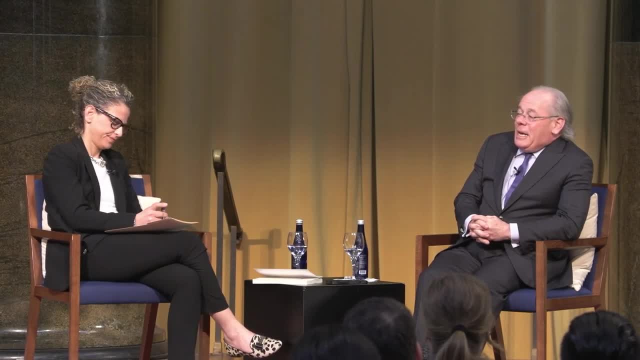 So Ralph Nader writes: unsafe at any speed And the automobile company says: you've got to put us out of business by making us have seatbelts. The same thing they said when we said you need catalytic converters and airbags and all the rest. 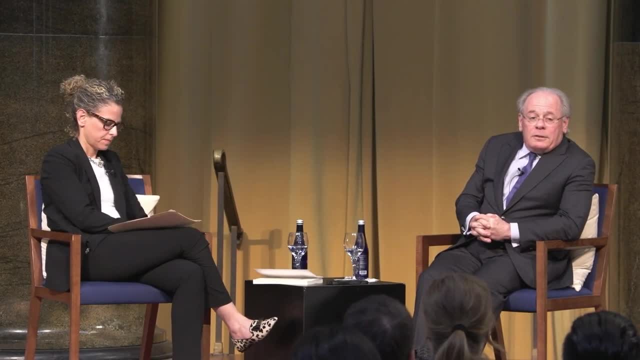 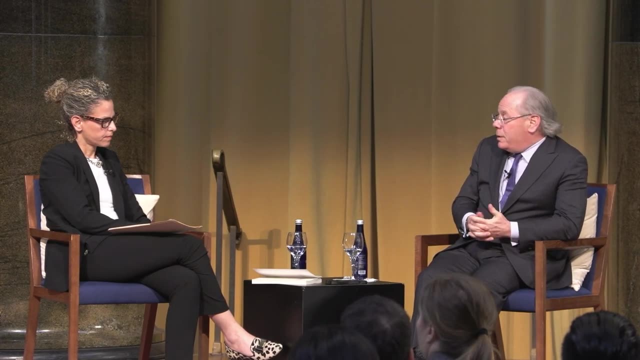 So now what happens? Family goes to the showroom and the salesperson says: this is a really safe car. It's worth the extra thousand bucks. And guess what? How much is my family's life worth to me? I think a thousand bucks would cover it right. 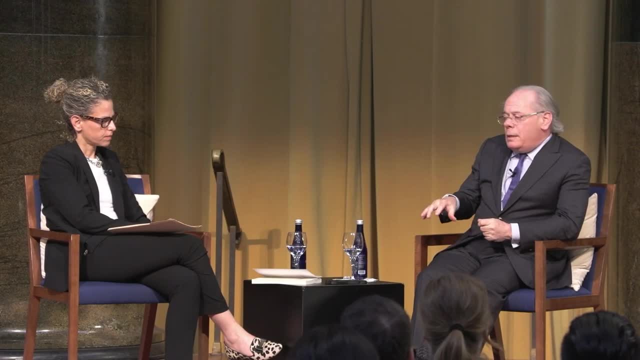 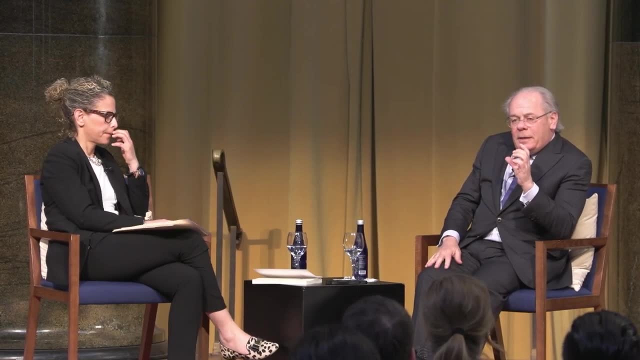 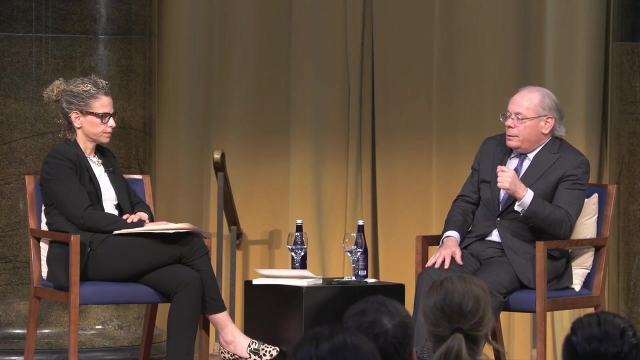 So the point is that we've made environmental protection a kind of product, And that requires innovation. You know, I think about energy efficiency as probably the best. You buy a modern air conditioner and it uses 25% of the air conditioners from 20 years ago. What happened? Well, the people that designed the air conditioner, the engineers, made energy efficiency a design parameter. Before they did that, it wasn't considered a design parameter. So they just- you know who cares? It's just energy. 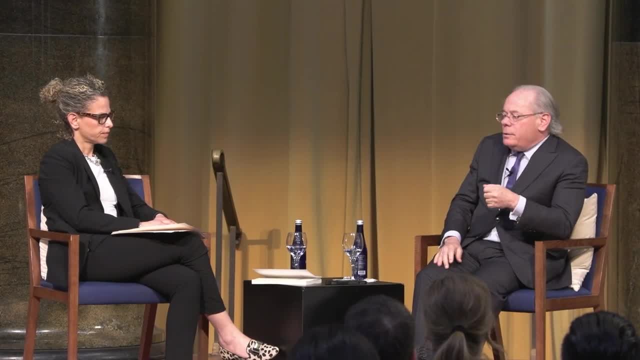 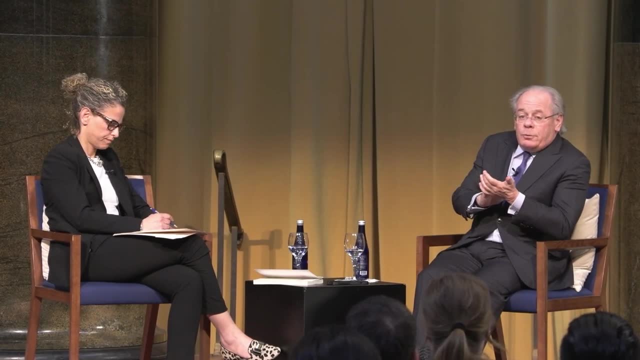 And so, by using human ingenuity, it inspires technology to make advances, And what happened with the automobile is a great example. After the engineers got finished with the energy efficiency that they needed for mileage and pollution, they started to turn to other things. 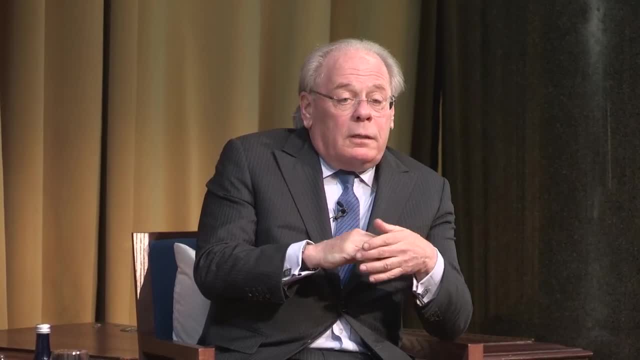 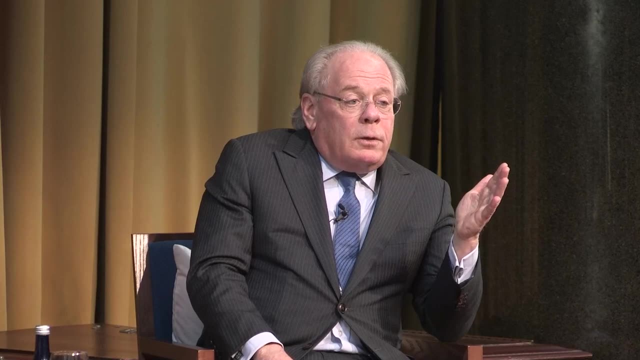 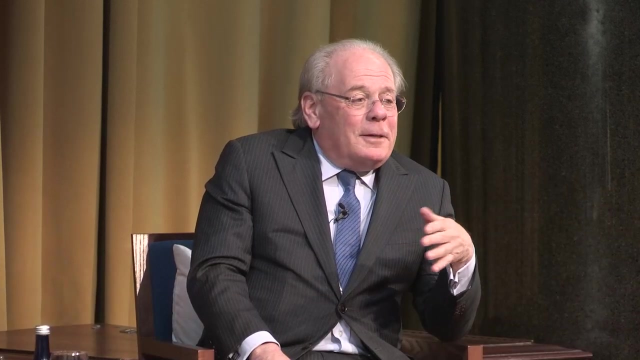 So now the motor vehicle is a mobile computer. There's many fewer mechanical parts And now we're on the dawn of the era of the electric vehicle, which is a. you know when the EPA last week proposed new air regulations And the answer was: there's no cost. 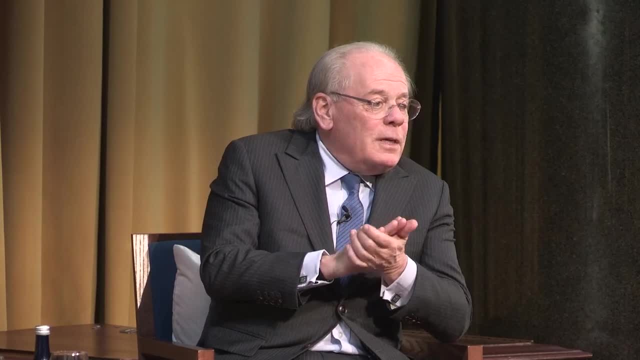 And hence the carbon emissions, And they have a lot of time to think about what that'll cost. So if you know the story of the big car, the carbon emissions from the motor vehicles, Tesla automatically qualifies because there's no emissions from their motor vehicles. So I think the point is the ideology of antiregulation which Ronald Reagan popularized. the idea that all regulation is bad for business is simply not the empirical reality. Regulation can actually be good for business. Now there's lots of bad regulations that are administered poorly and badly thought through. 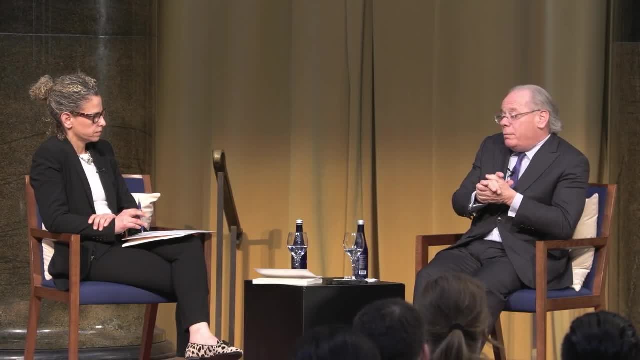 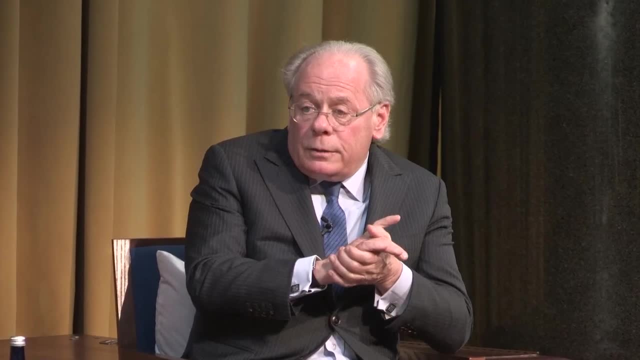 And those are bad for everybody. So One of the things I argue for is a more tailored, focused approach, so that you can work with companies so they can get to compliance without being destroyed. I'd like to pick up on something you just mentioned. 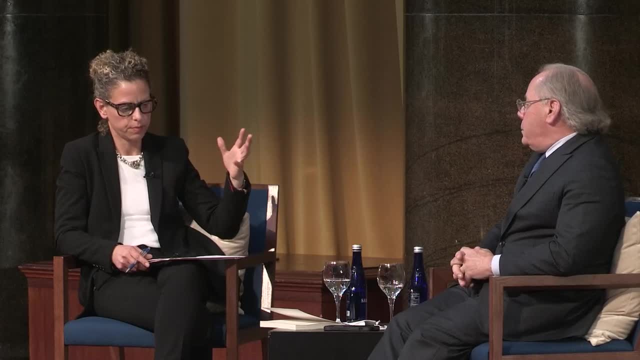 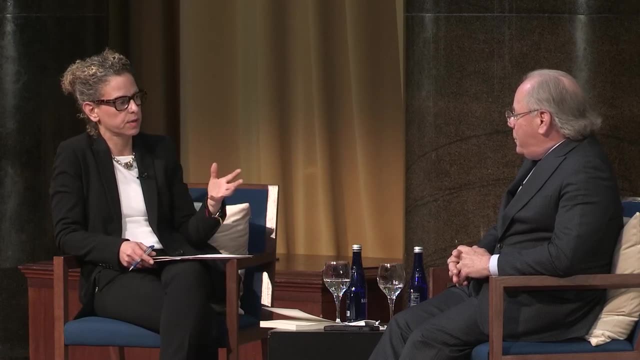 from the point of view of the products that are created and how they're more efficient, But a byproduct of what's created is something that you talk about an awful lot and a topic that you're an expert on, which is waste And you talk a lot about. 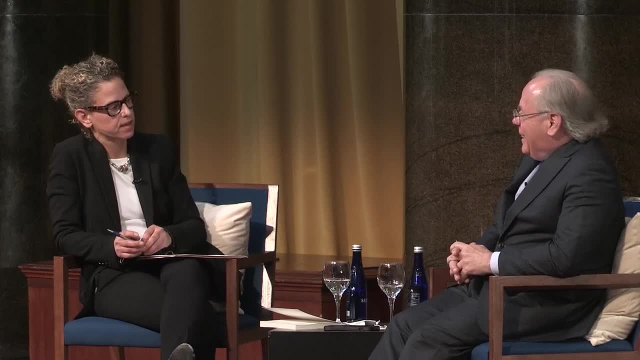 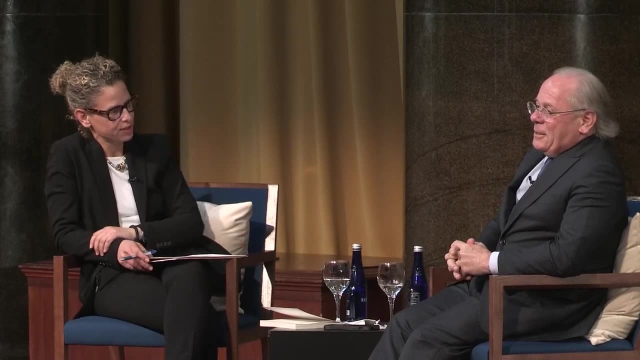 I'm heavily into garbage. You're heavily into garbage. I wanted to be respectful. We're recording this. So you're optimistic and you're heavily into garbage. What's changed over the time that you've been swimming in those topics? Well, I think we're heading toward the point. 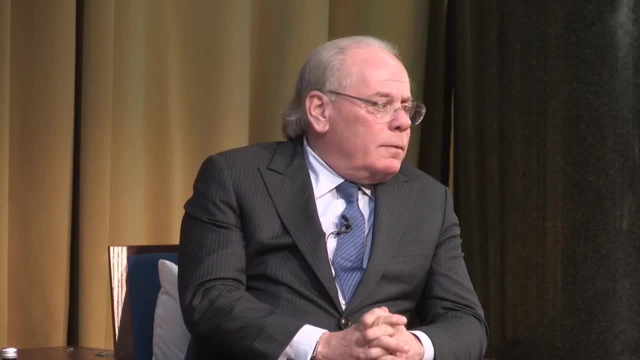 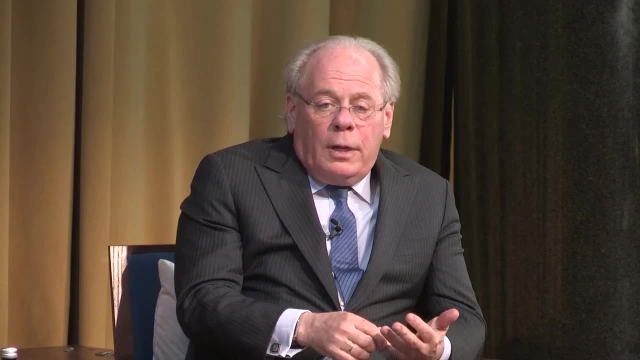 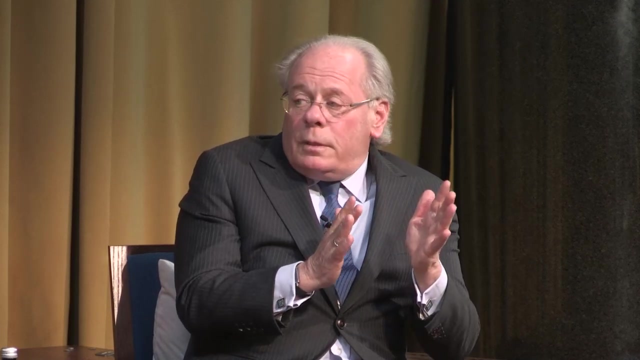 that mining from our garbage will be less expensive than mining the planet. Now that is a new way of thinking about this, But there are actually people working on applying robotics and artificial intelligence to waste management. And to get to that point, we have to admit some of our failures. 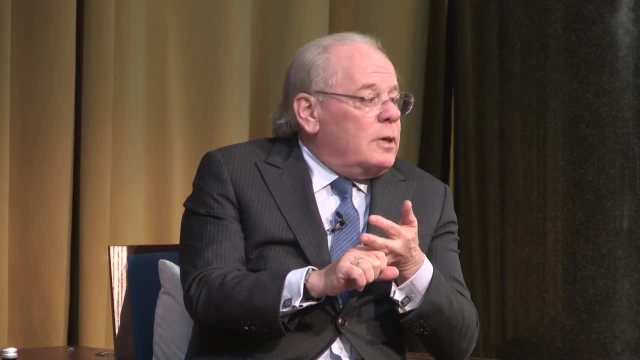 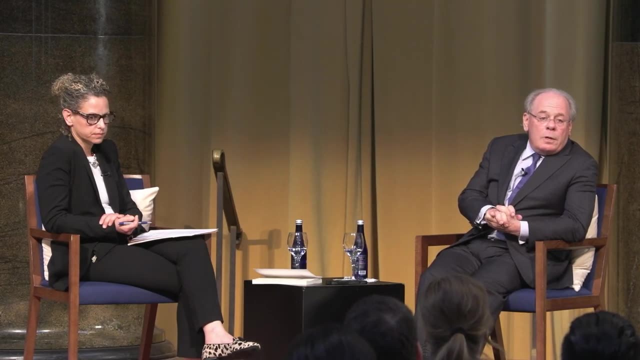 So recycling has largely been a failure. Admonishing people to separate their garbage and then developing individual markets for every product that comes out of the waste stream has not worked particularly well. Part of it is it's very expensive, Part of it is that the waste stream 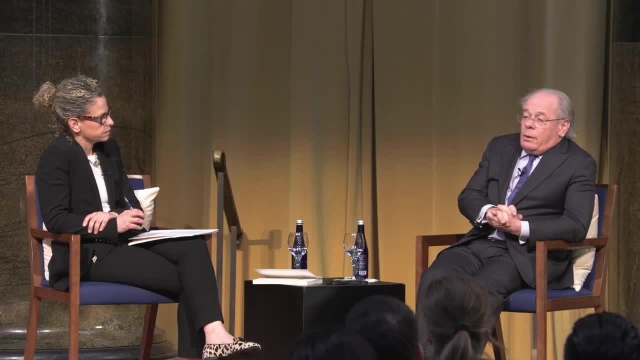 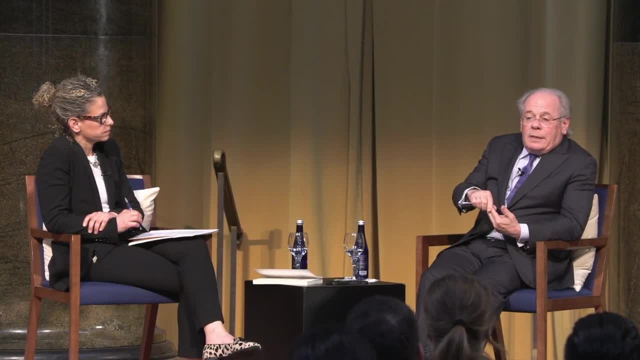 And that's a new way of thinking about it. And that's a new way of thinking about it using robotics and artificial intelligence. And you know, we all know that one of the transformative technologies of this part of the 21st century. 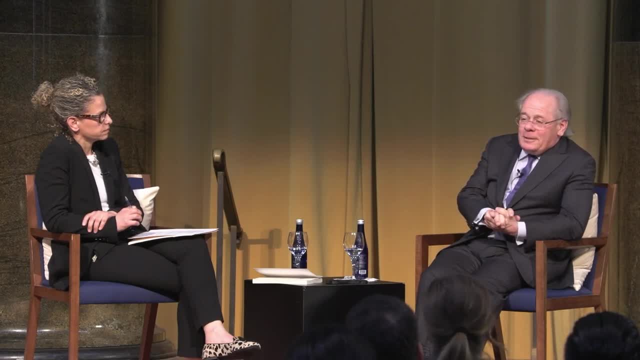 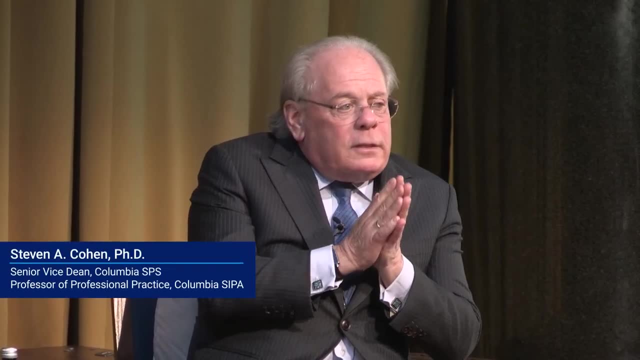 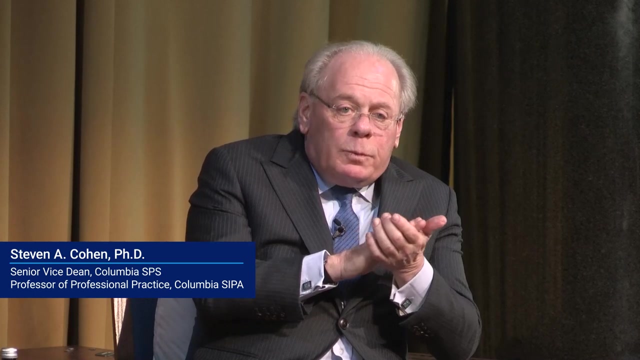 is going to be artificial intelligence. If you watched 60 Minutes last night, you saw some scary versions of it, But the idea here is that the planet itself is the main place we now get our minerals from. But what if our garbage became the place? 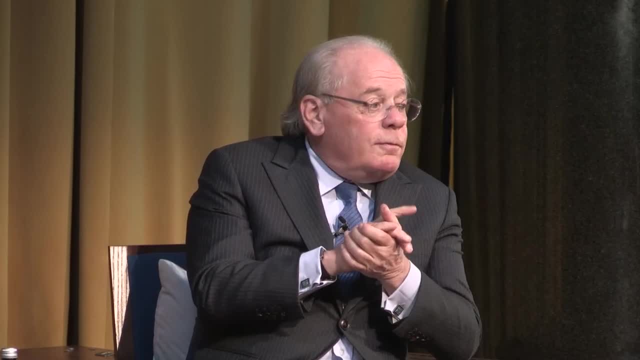 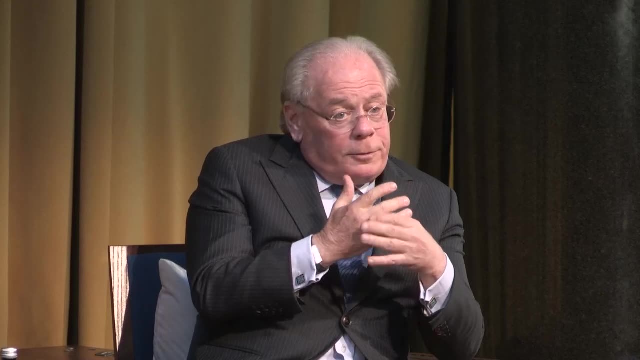 we got our minerals and raw materials from. We already know that. We already know how to do it with food and with fertilizer. What about plastics, metals and other raw materials? It's not going to be here next week, but in the next 10 or 20 years we're going to see. that as commonplace? What if New York City spends $2 billion a year on collecting its garbage and sending it someplace to either burn or dump in a hole in the ground? What if a billion of that came back to us because we were able to sell the materials? 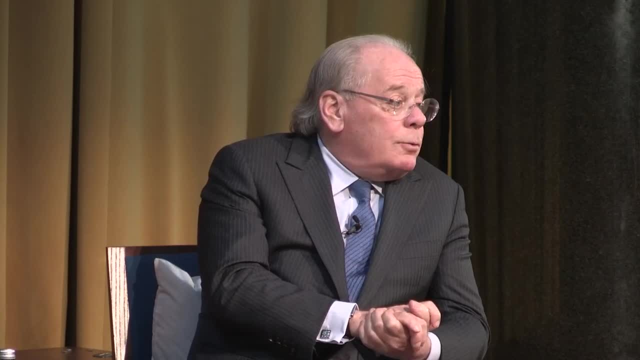 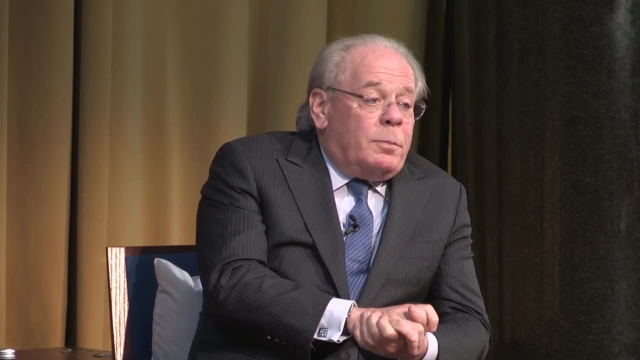 that we mined from our waste stream. That might make for a pretty interesting change in the economics of waste, and New York City has the scale to do it. Now, of course, the politics of citing these technologies is something that will be challenging. 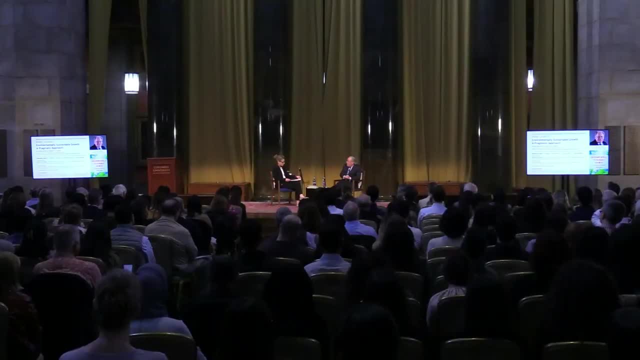 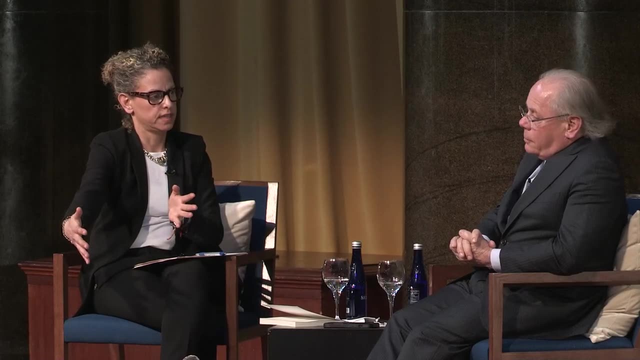 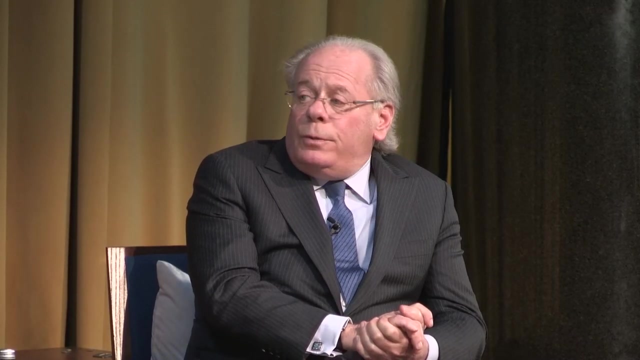 but I think it's feasible. You give a lot of examples of things that are possible. What's needed in order for us to realize that What's missing now? I think what's missing now is a little bit of confidence. Yeah, I think there's a lot of confidence that we can do this. 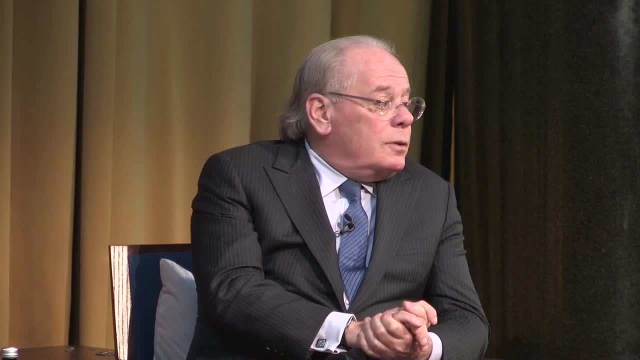 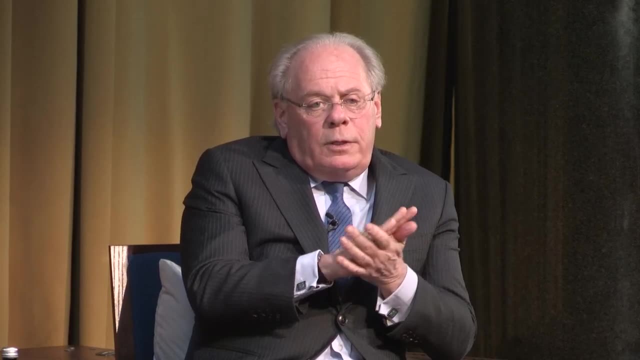 Young people worry that the planet's coming to an end, climate change is going to destroy us, that we've destroyed our planet and all the rest of that, And part of it is. I think you need to look back at history, at how economic transitions 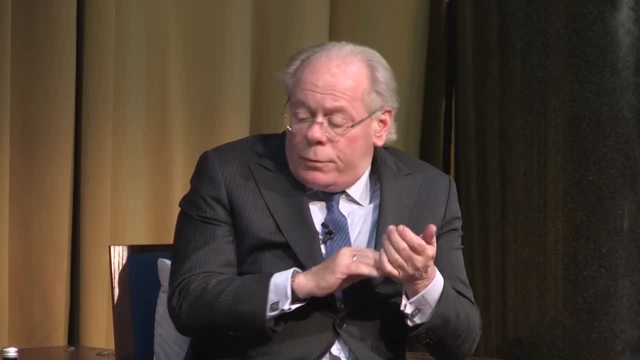 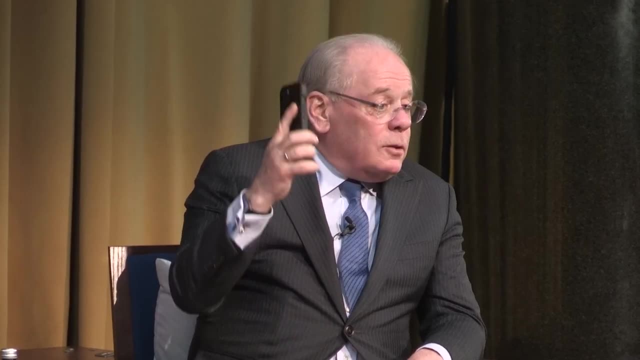 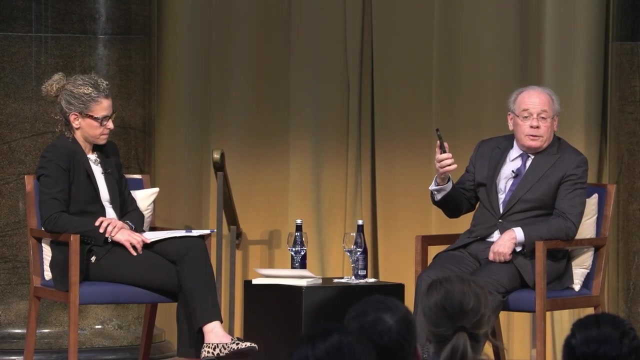 and technological transitions take place. How many of you knew that we're around 20 years ago, that we would have to carry computers with us wherever we went? I think this is actually more important than our wallets or anything else. Think about what happens when you lose your phone. 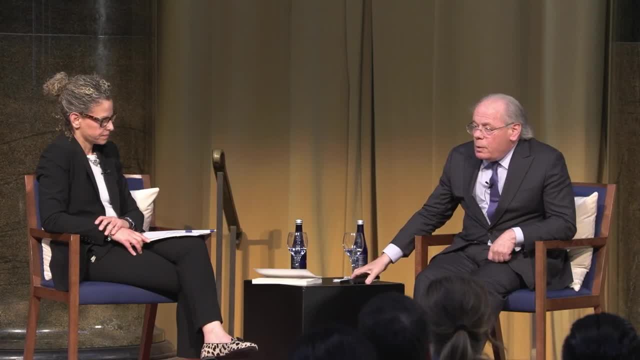 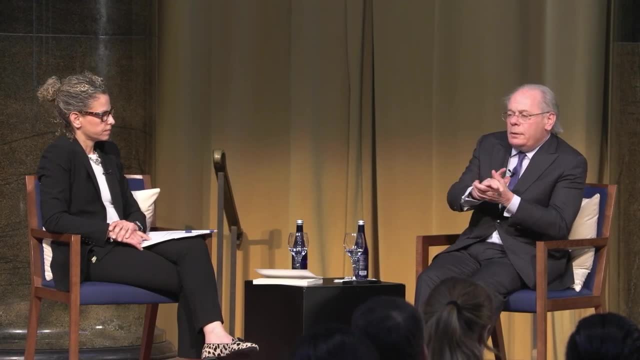 It's like something horrible has happened to you. So we've been in the midst of this technological transition. New York City is what I – I usually use the physical dimensions of New York City as an example. New York City starts as a trading city. We traded furs and agricultural products from the surrounding countryside. There's a lot of trade. They're all in the United States and we sent it to Europe. So we were a trading city at first. In fact, we got so good at it. we built the Erie Canal. 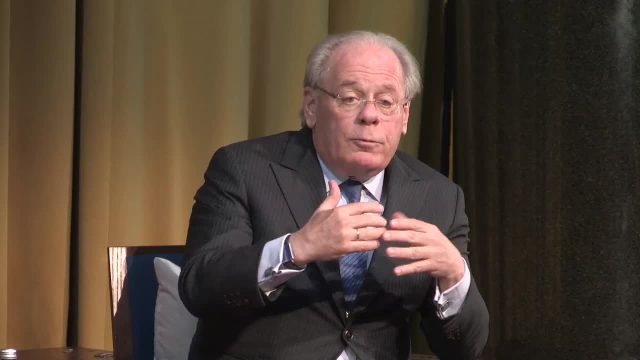 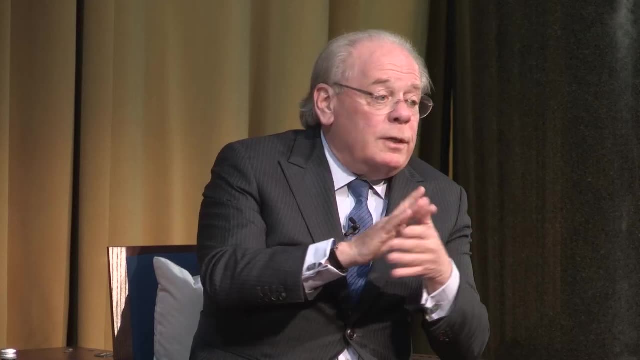 and were able to get the entire Midwest to come through the Port of New York instead of New Orleans, which would have been the natural place for stuff to come out of the Mississippi. We came through New York, So we were a trading city. Then in the 19th century we became a manufacturing city. 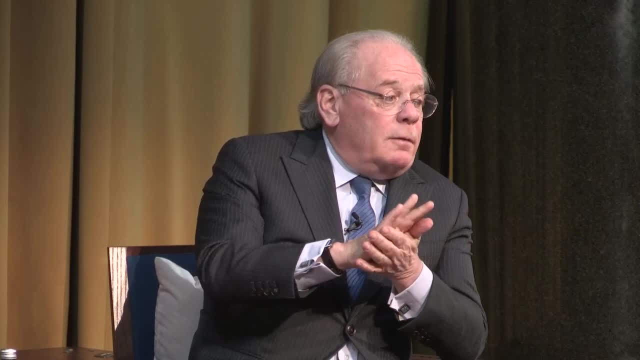 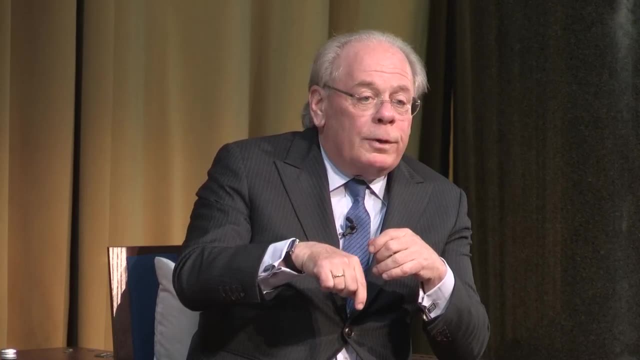 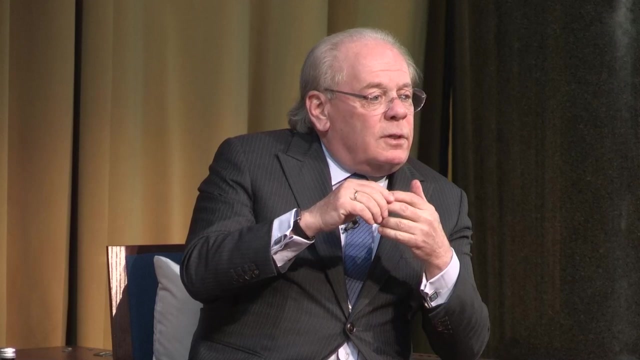 particularly toward the end of it. In fact, at its peak in 1950,, New York City's clothing manufacturers made 95% of the garments worn in the United States of America. okay, We had half a million garment workers. Today we have 150,000 people working. 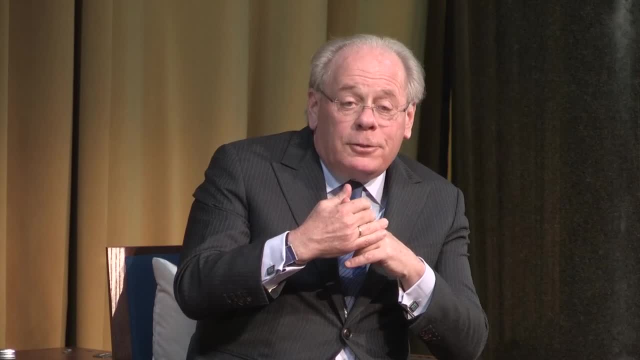 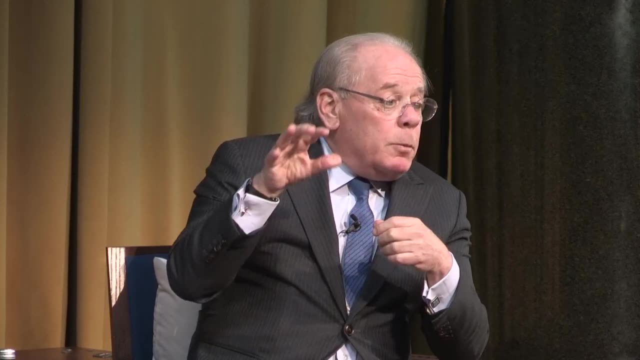 in the garment industry. We now call it the fashion industry in New York. We make almost no clothing here except for samples, but we design it and sell it and we make much more money doing that than manufacturing 95% of America's clothing. 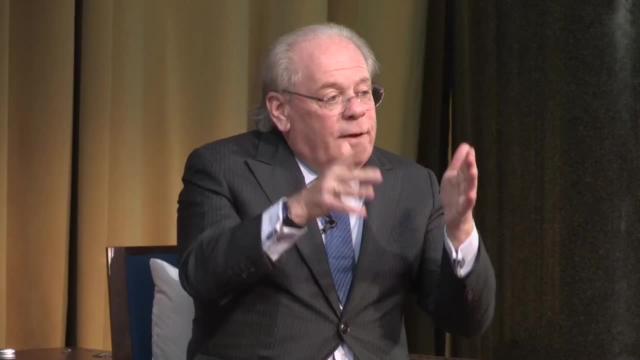 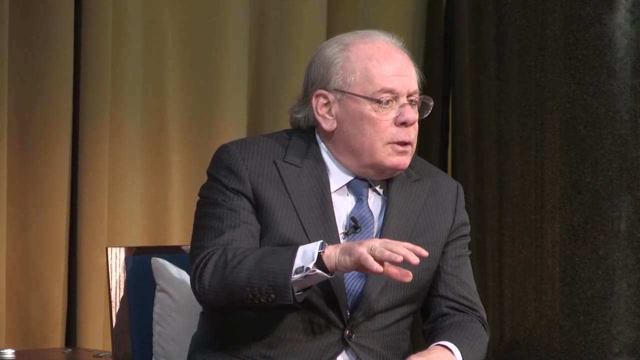 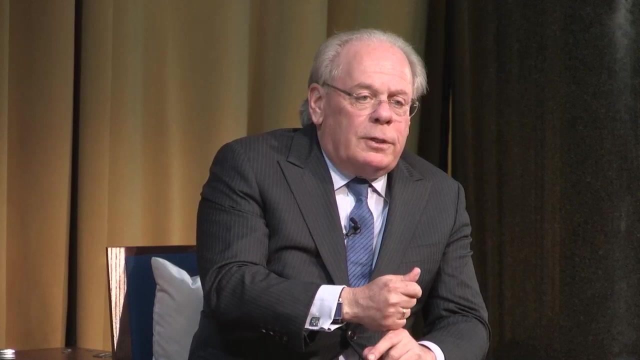 So we have transitioned from manufacturing to manufacturing and manufacturing to manufacturing. We're now at the beginning of the transition from a service city to a renewable resource-based city. And what's the evidence of that? The local laws have been put in effect to try to change our energy use. 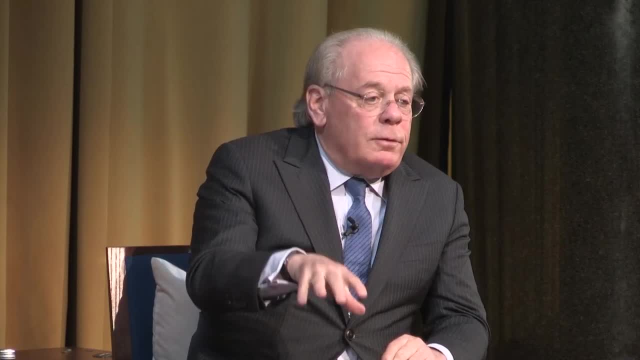 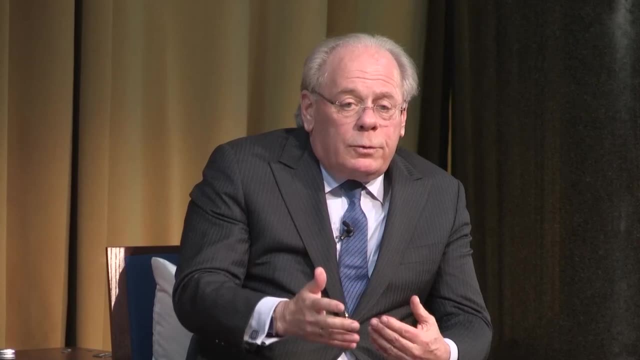 what's going on to try to make us more energy efficient, The kinds of very slow transitions we're seeing in the energy sector and the renewable resource sector. it's not going to happen next week. This is a generation-long transition, but we're at the beginning of it. 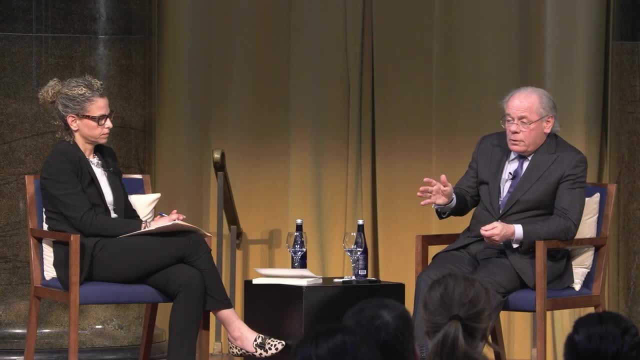 I can tell you, in the middle of the transition from manufacturing to services, everybody thought the city was going to come to an end. We lost a million jobs. People thought that was the end of New York And somehow we reinvented ourselves as a service-oriented city with education, entertainment. 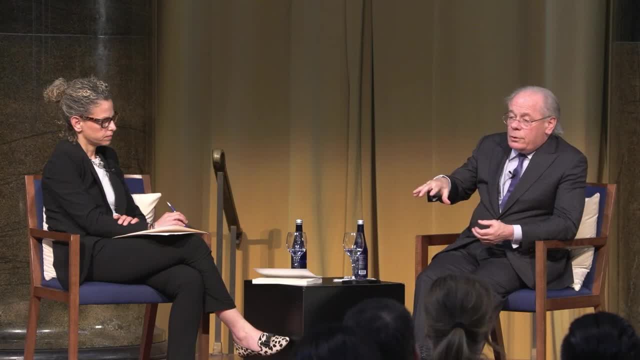 healthcare and the rest. Now we're at the beginning of the transition to a renewable resource-based city and country, and I provide some examples at the end of the book of places that are doing that. Who's responsible for fueling that? Is that coming from the technology? 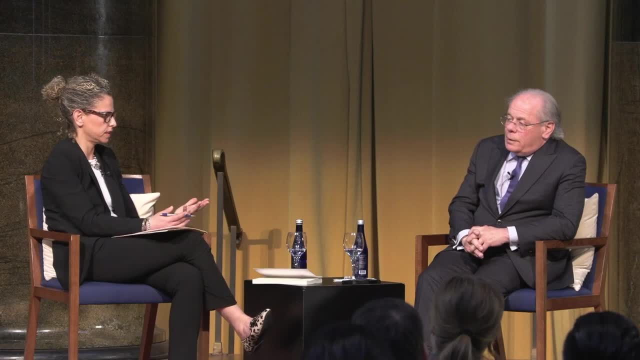 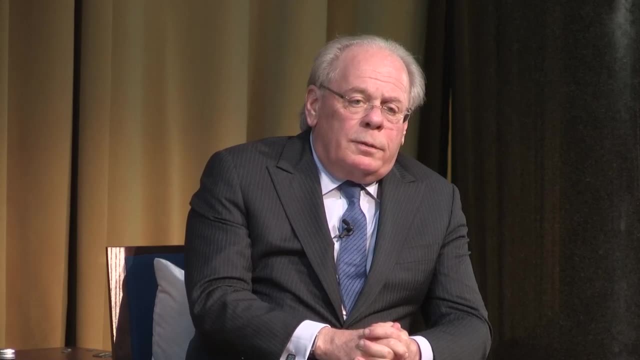 from the private sector. Is that government Who's investing in this new future? I think there's a bunch of things going on. Some of it's public policy, pushing it through state and local governments, and then we see the Biden administration getting into it. 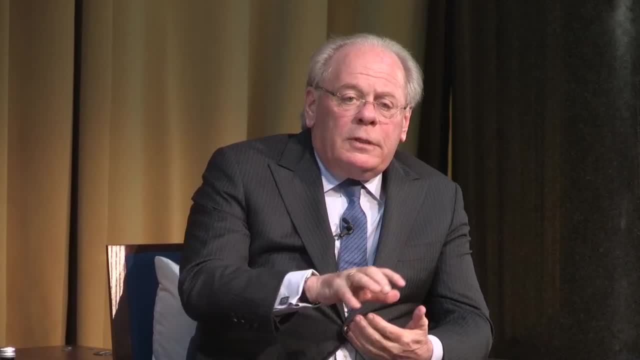 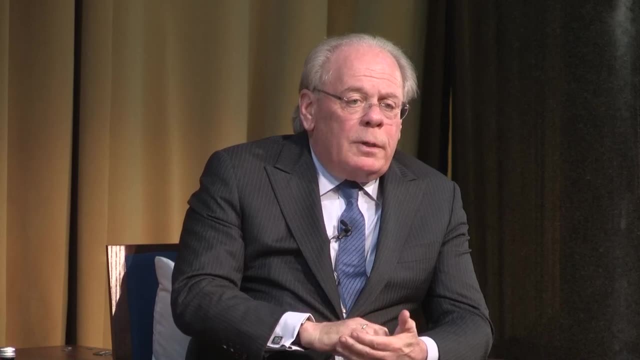 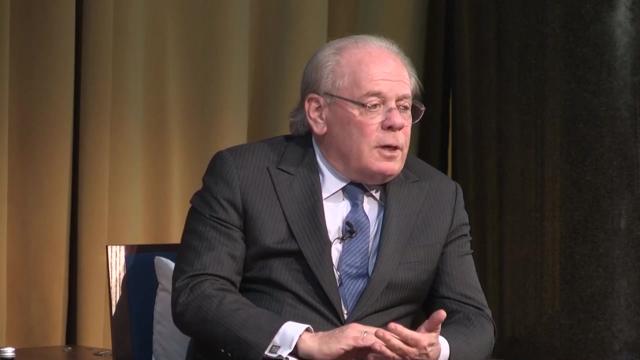 We see particularly businesses starting to understand that they need to account for the risks associated with environment. So I think the most important change that's about to happen. if you read the Wall Street Journal today, you would see that the SEC is coming close to finally issuing its carbon and climate risk disclosure. 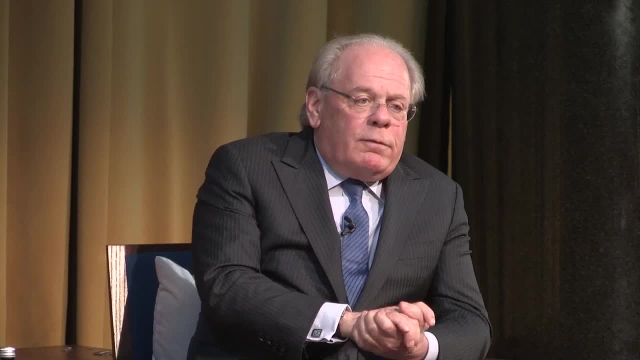 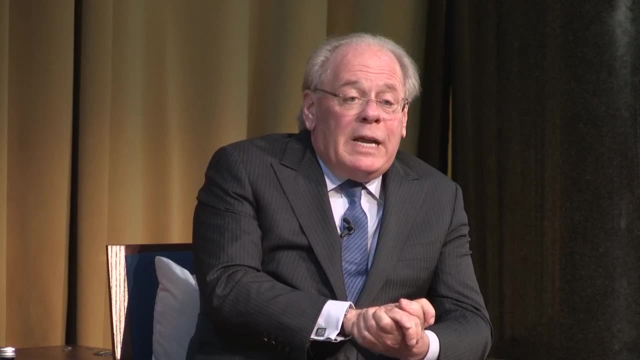 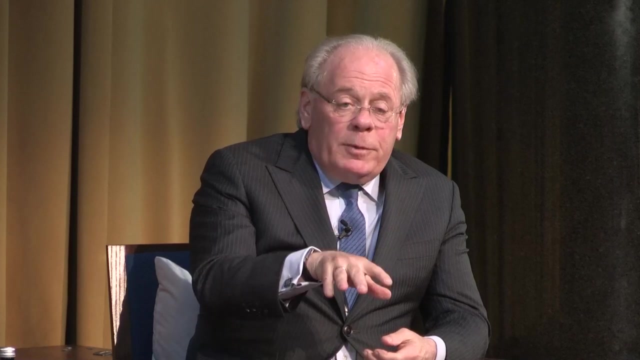 This single regulation is gonna have a massive impact on American corporations who, many of whom, have been reporting voluntarily on ESG issues, but now we're gonna have to do it very specifically according to government rules. Now those rules are gonna be very preliminary. 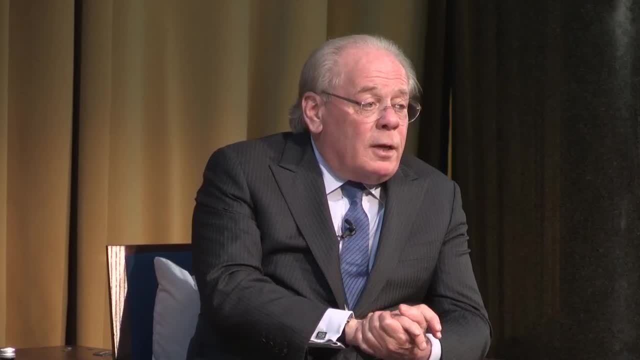 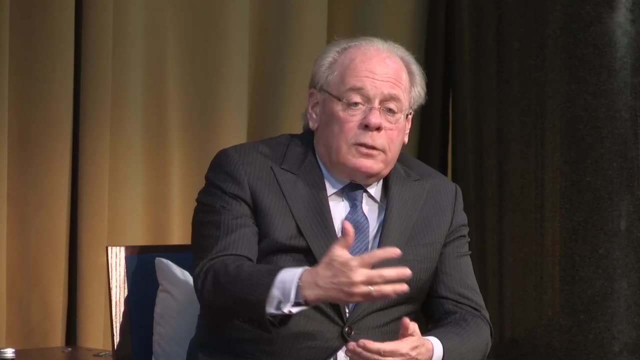 They're gonna be challenged in court. They're gonna change, but it's a lot like accounting in 1930s, When we created generally accepted accounting practices to get access to the public stock market, we created the profession of accounting and chief financial officers. 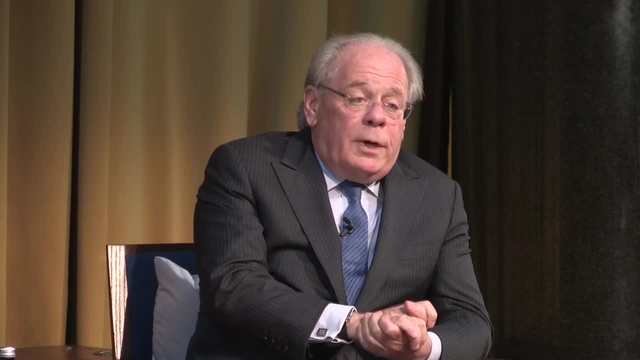 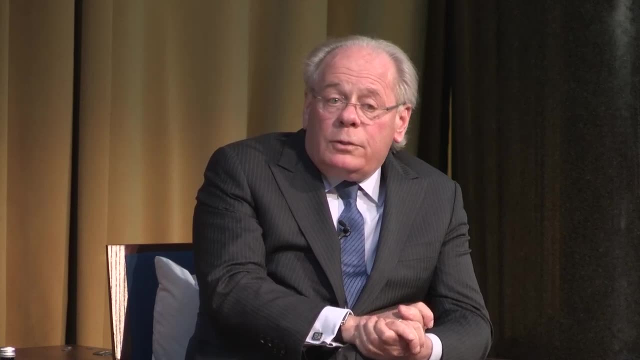 There were very few of those in the 1920s. So now we're gonna be creating the position and we have it in the federal government. It's starting in local governments, starting in many businesses of chief sustainability officers. That's being fueled by market forces. 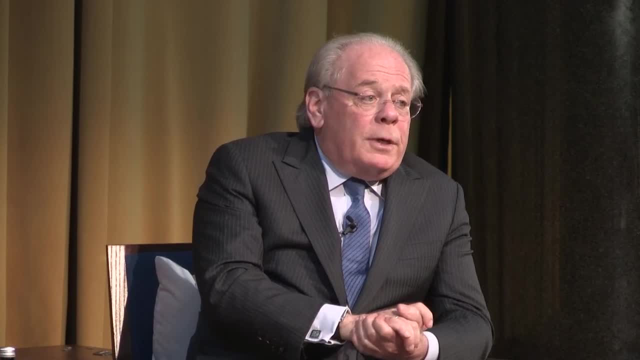 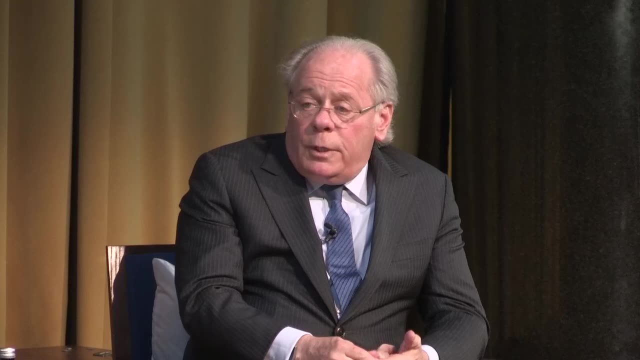 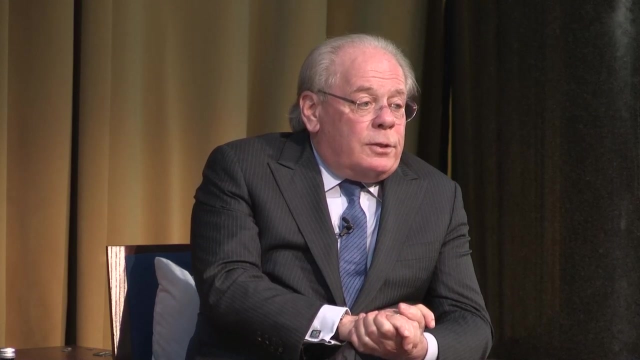 It's being fueled by public policy. In fact, it's being fueled by young people who are coming into organizations and asking questions about environmental impact, diversity, equity, inclusion and governance issues, and it's changing the world. Now, sometimes this gets criticized. 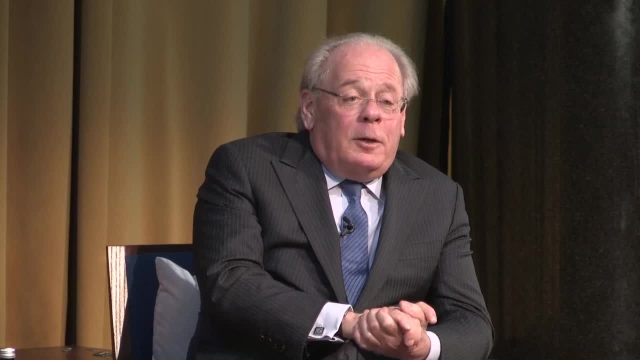 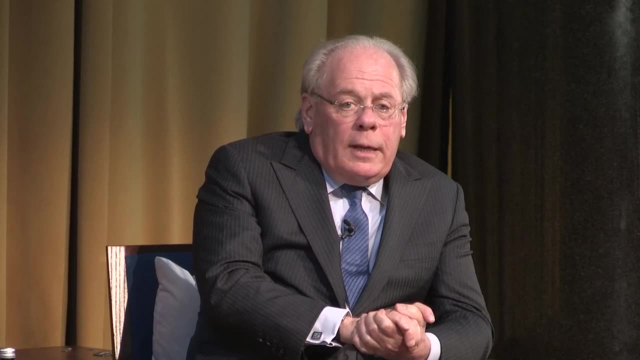 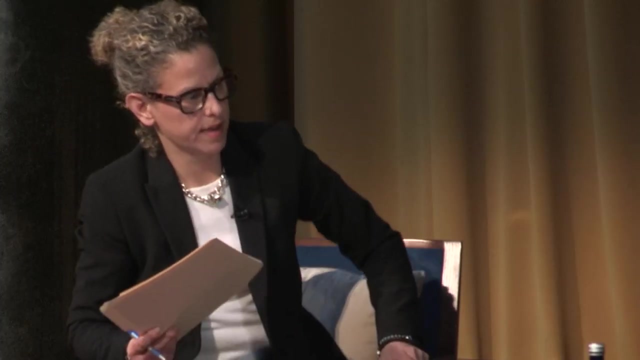 as somehow being woke. Well, I think woke is better than being asleep and I think these organizations are aware of their environment and that's making a sea change in corporate governance. You speak about Etsy in the book. You cover Apple, You cover Walmart. 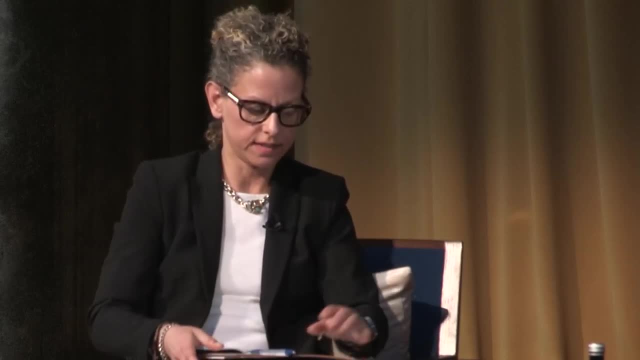 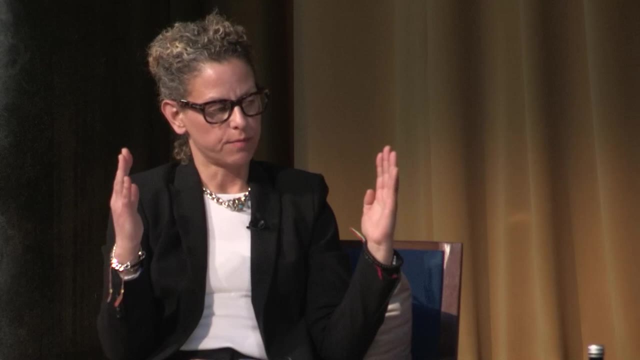 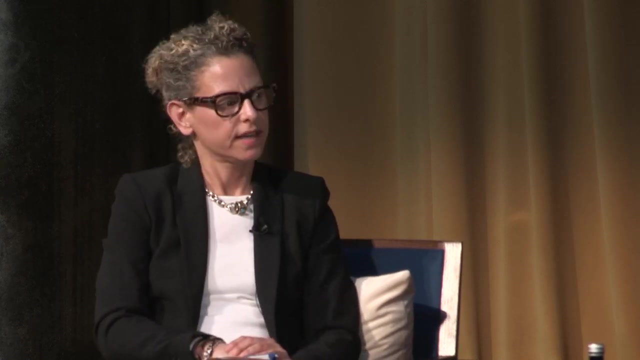 Just I think I mentioned this to you earlier The weekend- this conversation, your book, your work in particular struck me as my eco-conservation team from Mattel arrived in my Walmart box. For those of you who don't know, it's a chief sustainability officer, Barbie. 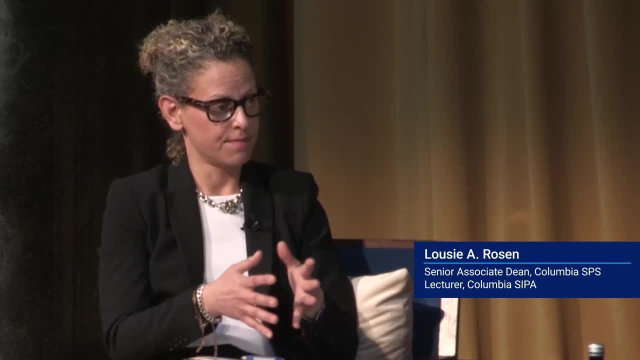 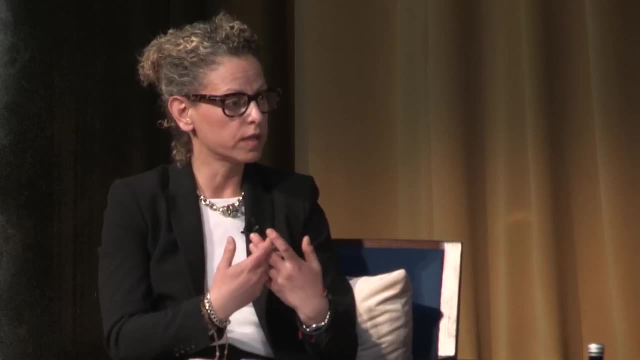 and that made me think of how far we've come. So you see a very strong role for the private sector and you see the Walmarts of the world playing a role in the sustainability of our resources, and you call for a need for there to be a shift. 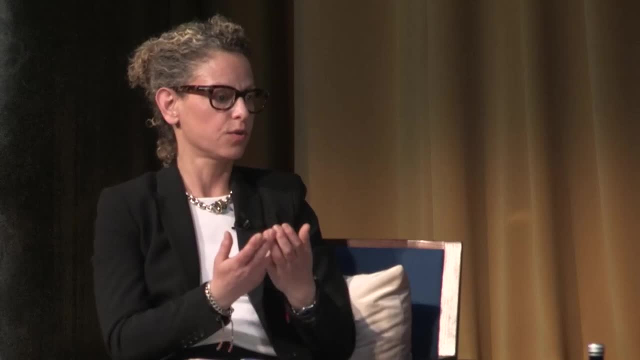 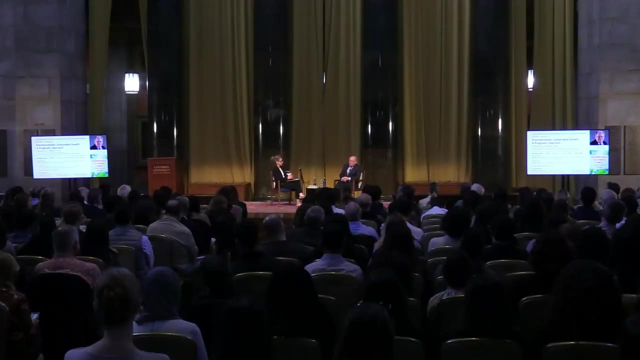 in how we talk about business. we, as environmentalists, talk about business. Can you talk about that a little bit, about how things have changed so much that they're now our stewards? Well, Walmart is the fastest, the fastest adopter of solar power. 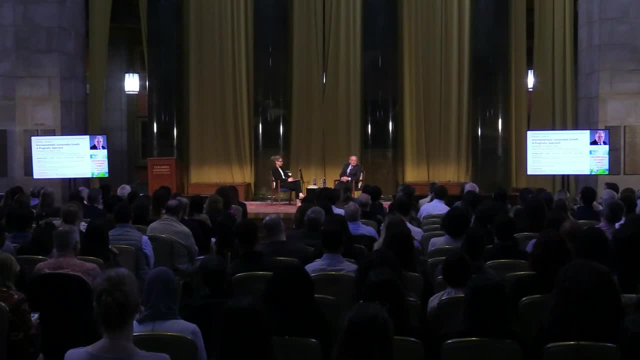 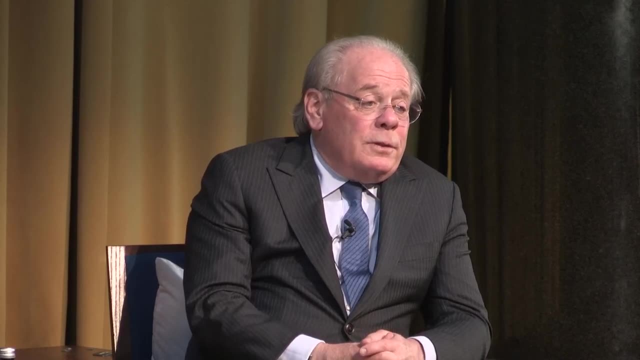 of any corporation in the United States. Why are they doing it? They're an Arkansas-based firm. Their clientele is not that concerned about climate issues, So they got into it because they saw the profit in it: Solar power. they have a lot of flat roofs. 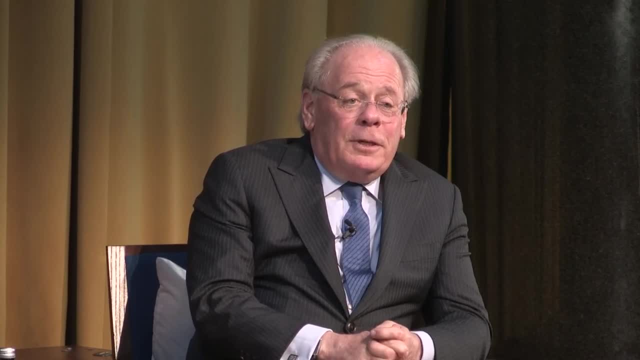 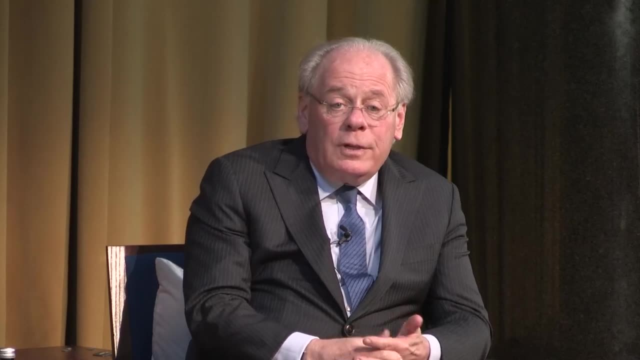 on their buildings- you've probably seen these- And so they figured this is a good place to put solar arrays. and they're so rich they'll recover the capital quickly and have cheaper energy, And they use a lot of energy in their stores. They also announced a couple of weeks ago that they're gonna put charging stations in their parking lots and gas stations. And why they do that? Well, while you're charging, you're going inside Walmart to buy some laundry detergent. you know, Concentrated laundry detergent, by the way. because they won't sell any other kind, because that makes them more money and less space. The point here is that the idea that a renewable resource-based economy is bad for business is empirically untrue, And businesses that are getting into this area are seeing it, and that's what I think's going on. 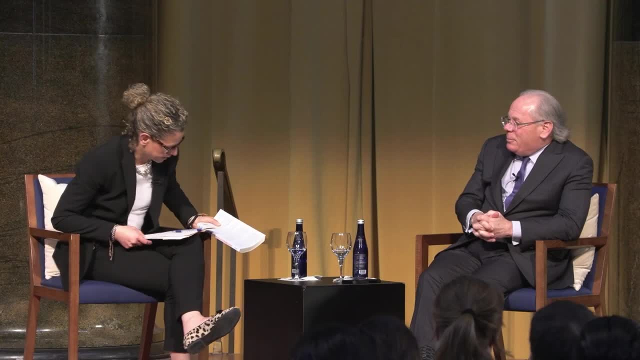 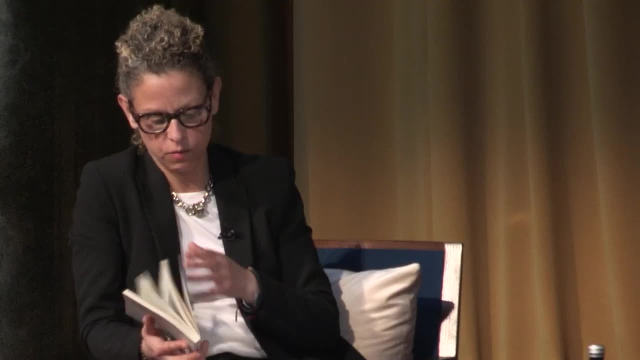 I'm conscious of the fact that you and I could kibitz on this stage all night about this, and I have to give our audience time, but I have one more question I wanted to ask you, And so I want to end our conversation. 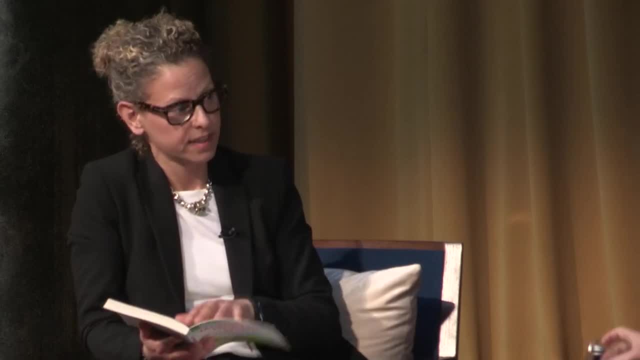 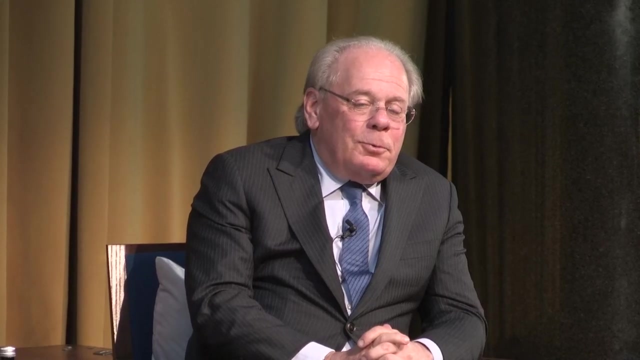 with the beginning of the book that you donate, you dedicate to your granddaughters. So what does the world look like when your granddaughters become fresh women in college? Well, that will be 15 to 20 years from now, I guess. 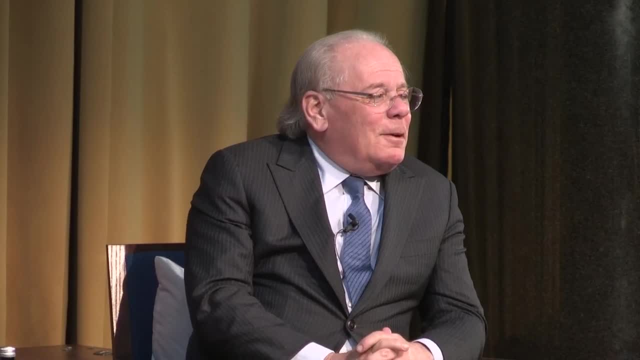 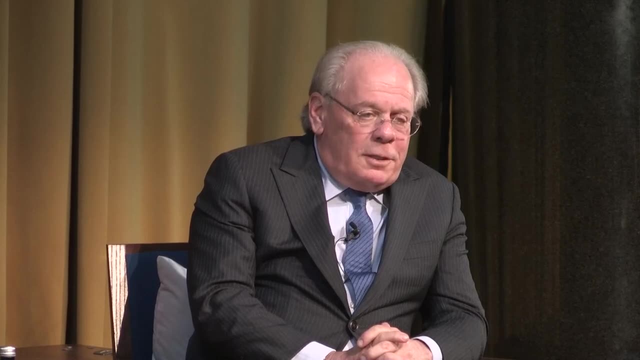 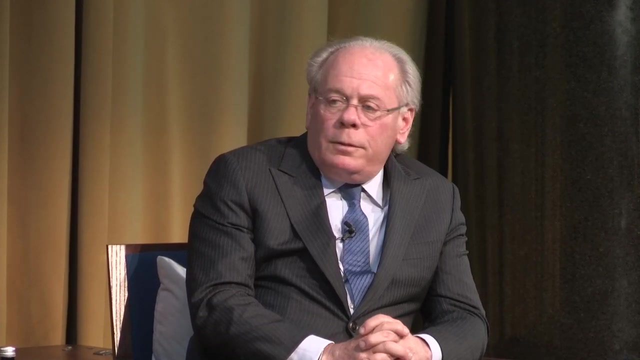 maybe 13 to 18 years from now, something like that, and I think this transition will be well underway. I think that I did dedicate it to them because I think that Robert Hallburner wrote a postscript to his book An Inquiry to the Human. 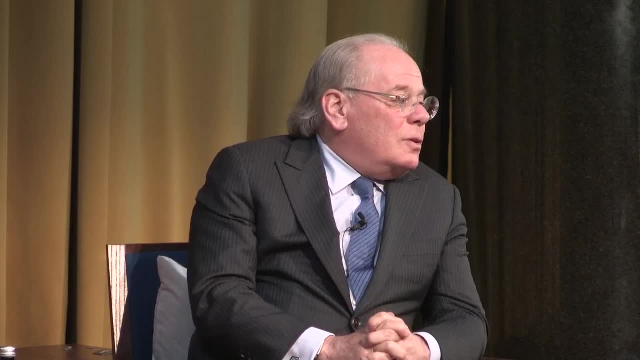 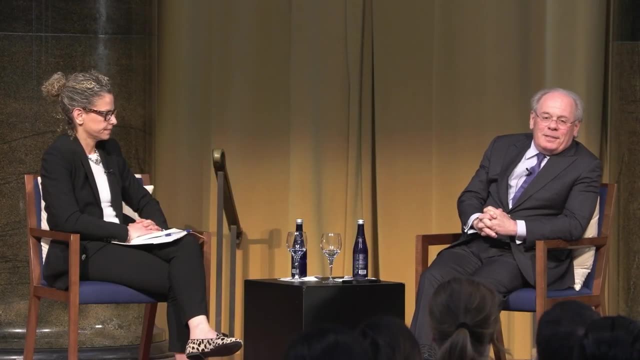 prospect. what has posterity ever done for me? so, in pure economics term, in pure economic terms, the future doesn't matter, but it does matter. it matters to all of us because you know, we care about what's coming next and what then the world, our children and grandchildren will inherit, and so 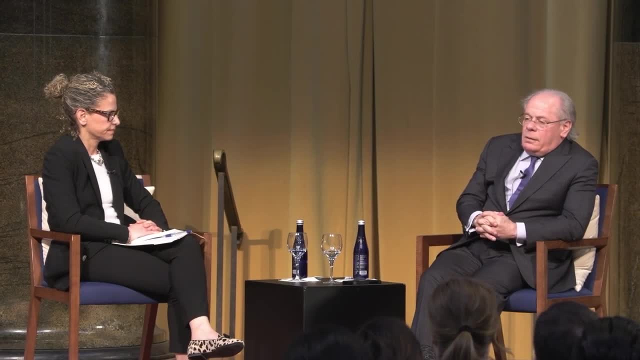 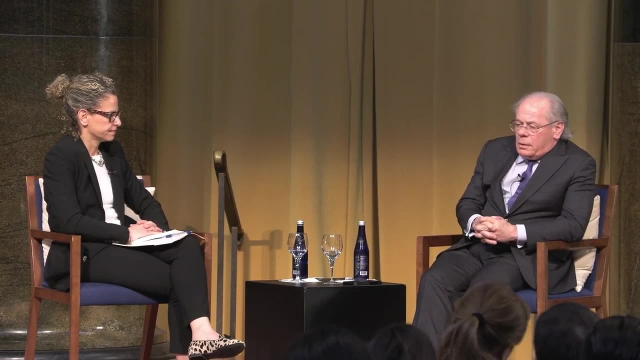 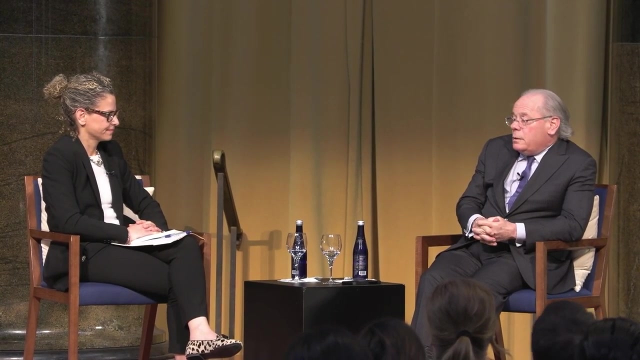 I think that we owe them, we owe these next generations, enthusiasm, optimism and a can-do spirit. that's how America got to where it is today and that's really what gets us to the next place. and I think this pessimism and this polarization, and particularly the symbolic politics, at one 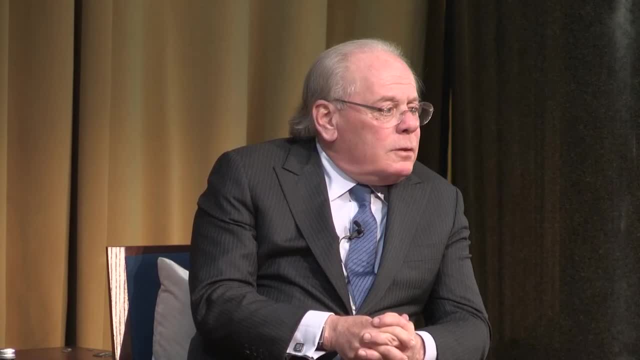 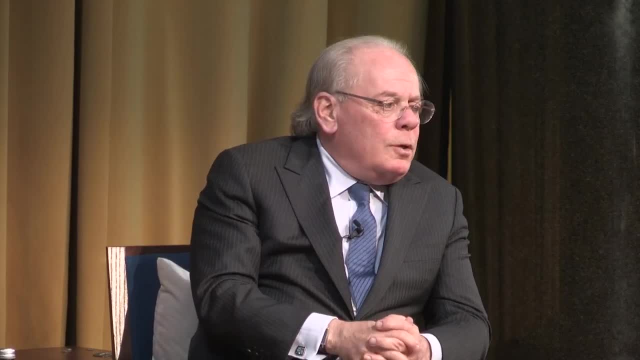 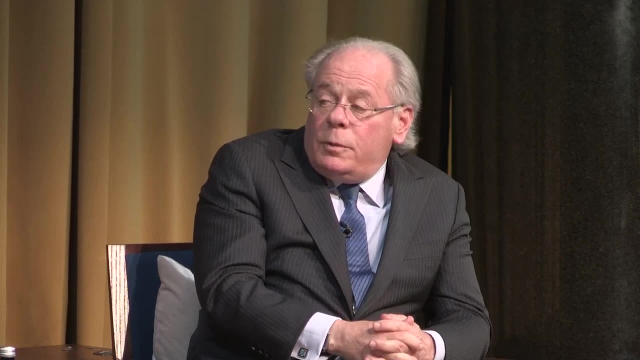 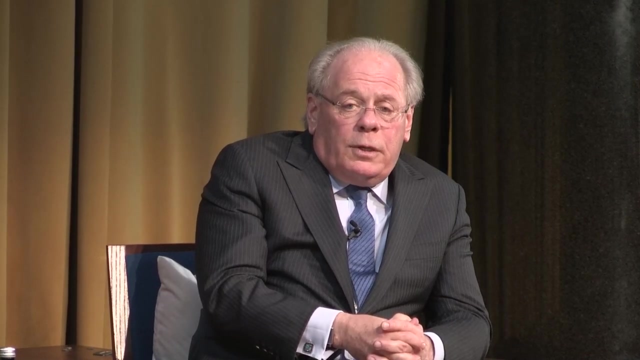 this goal by 2030, this goal by 2040? well, I want to look at what we're doing today and see how much better we can do next year, rather than going for some aspirational target that may or may not be real. and I want to do it because I want my grandkids, by the time they're adults, to be in a 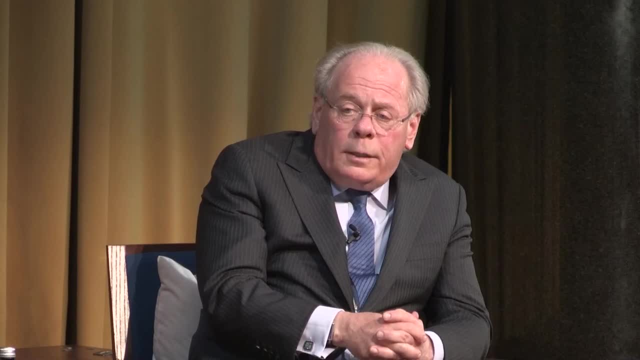 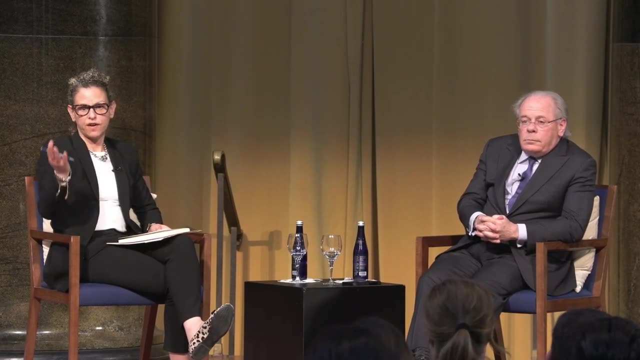 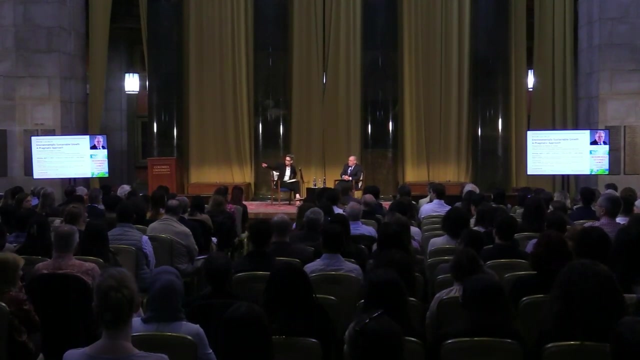 planet where this pessimism has been wide, widely displaced by a more optimistic outlook. thank you, Steve. I'd now like to invite members of the audience to ask questions. so if you do have a question, please raise your hand and one of our colleagues will bring a microphone to you. and I ask also that you ask questions, not give speeches. so who would 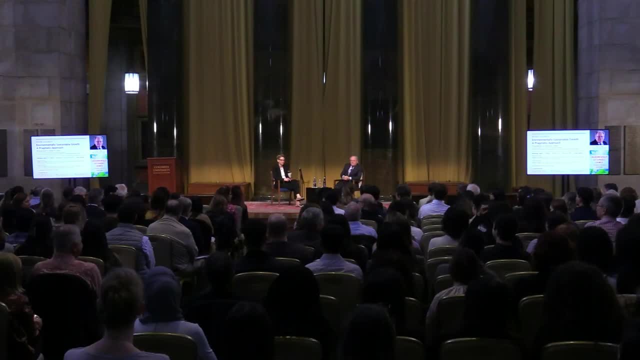 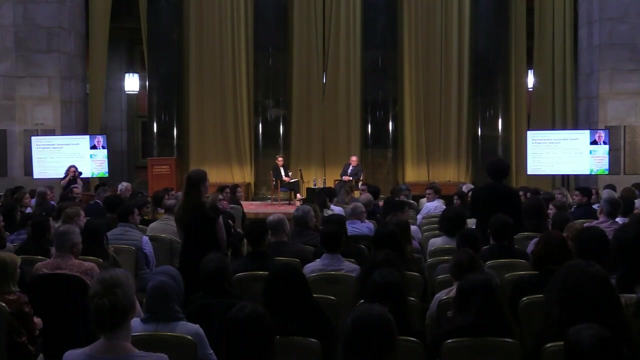 like to. who wants to raise their hand for the first? throw the first one out, somebody over here, please. thank you, uh. hi, I'm Cheyenne Jody. I'm an undergrad student studying environmental science, public policy, data science. I'm interested, uh, because, as a young person myself, there's a lot 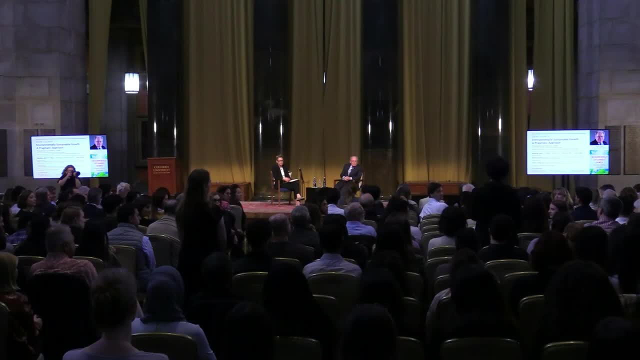 of talk about. you know, as we transition towards a greener future, greener transition- how that is going to shape. a lot of the predictions that have been made about rising sea level or rising temperatures, like: is there a big impact that we will see as a result of us switching over to solar? 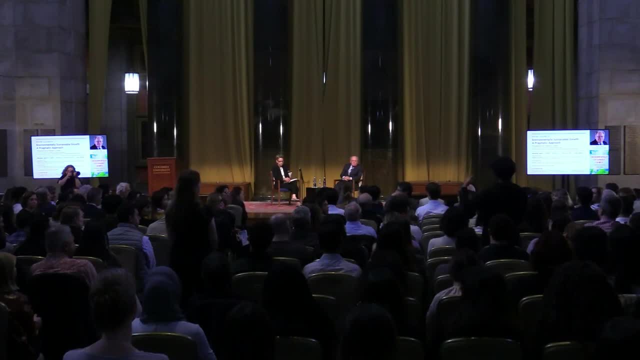 panel or wind farms here in New York, like, if we have a transition, like of the NYCHA houses, to using solar panels, is it going to have a large impact on on, uh like parts of Queens flooding or parts of Manhattan, like some of the coastlines? thank you, well, one of the issues with climate change and this is why. 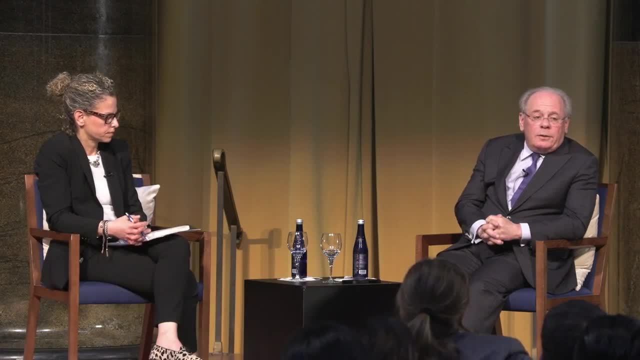 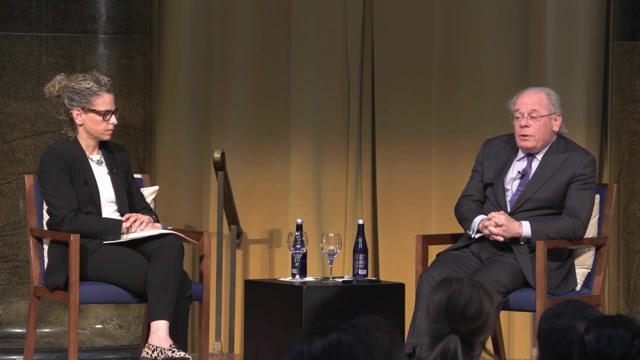 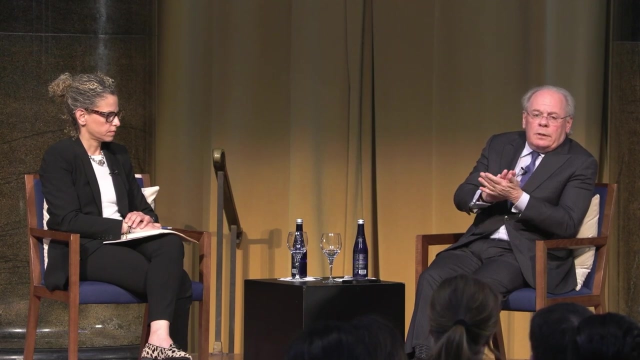 its politics was so difficult is it's created everywhere and its impact, at least up until now, was largely in the future. now, fortunately, our models 20 years ago did predict exactly what's going on, so we do know this is. this is happening. I think that what we're going to see and what we've 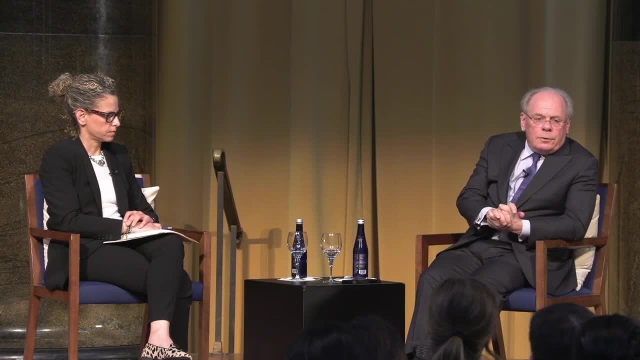 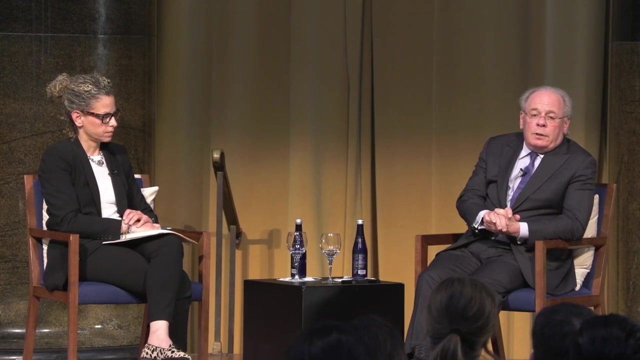 started to see is the beginnings of this technological transition which will have an impact all over the world, but it's going to take a while before we see it. we're going to have another 20 years of increasing heat and increasing extreme weather, more sea level rise, and so the immediate priority is going to be on. 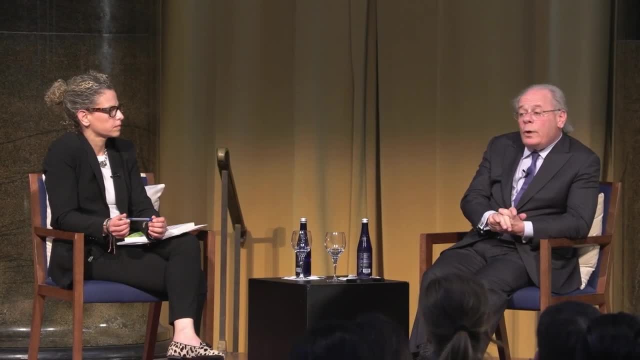 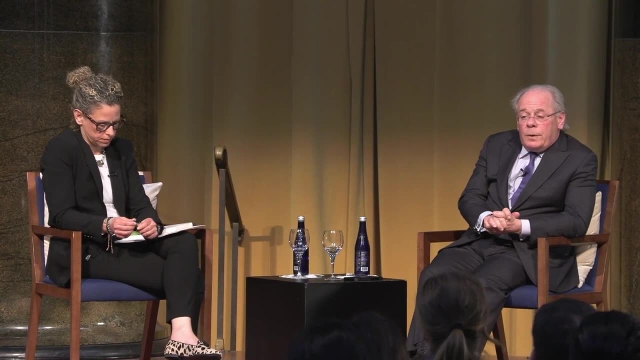 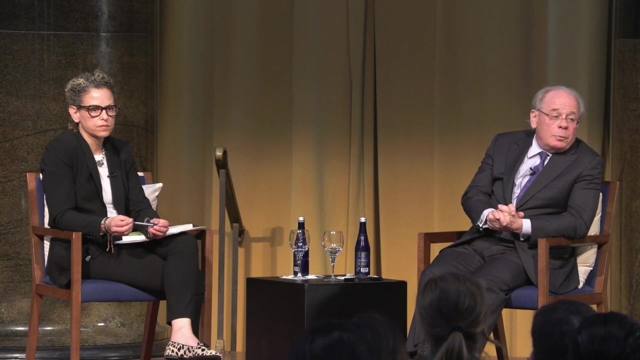 adaptation, making sure that we create more resilient cities. now. New York has spent billions of dollars already to do that. con Edison, you know, the plant that once was underwater during Hurricane Sandy is now pretty weatherproof. most developers in New York are not putting their new utility rooms in the basement, they're putting it. 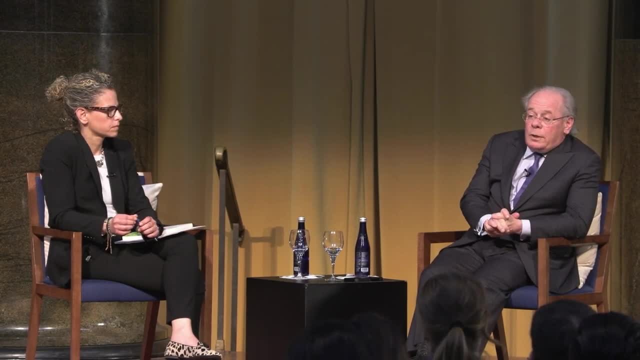 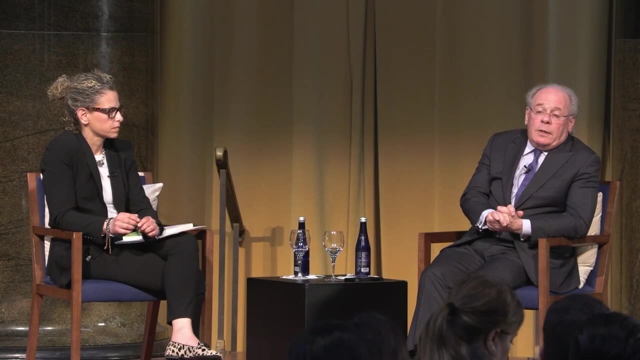 up on the third floor and lots of people that live close to the shoreline have raised their houses on stilts, knowing that the waters are going to come. so we're- we're going to have to get better at this, but then some of the impacts, like you know, after either the five inches of rain in one hour that. 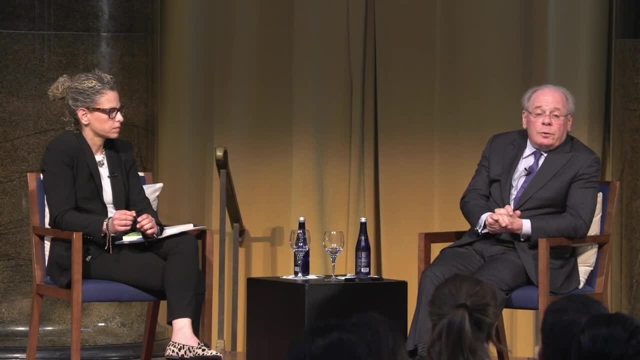 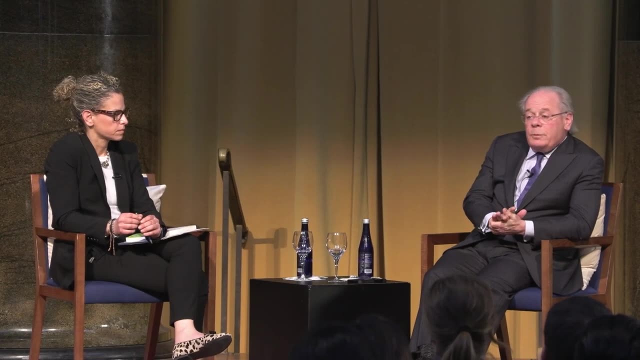 that flooded people's basements. that's going to take different kinds of solutions. the good news in New York City is you don't have to convince people. people know there's a problem and they're willing to get together to try to help solve it again. it's not perfect. I. 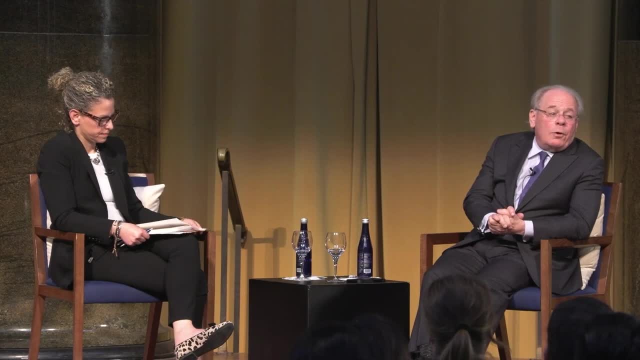 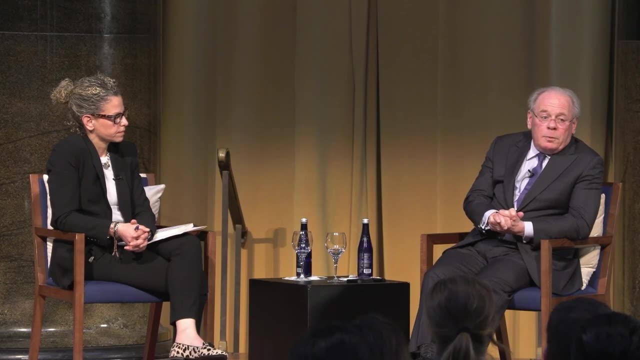 shouldn't. I don't want to give the impression that everything is easy and everything's perfect. this stuff is hard and, like I said, public policy is about making problems less bad. we're not going to solve these problems, but we're going to make them less bad, and I think one of the reasons that's 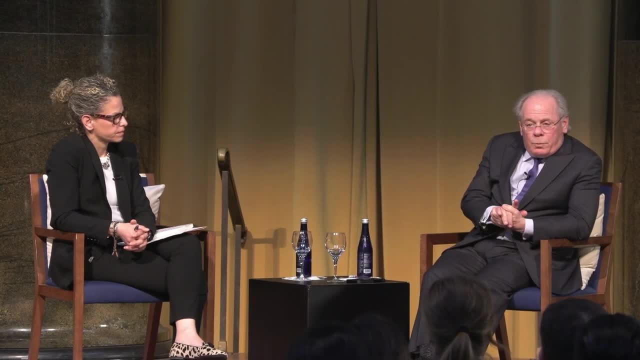 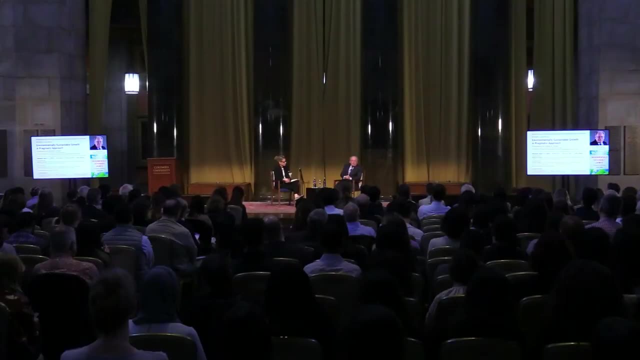 going to happen is that these transitions are underway. I mean the one that I point to, that, I think, is really picking up steam, if you will: electric vehicle. the electric vehicle is coming and it's coming very, very fast, much faster than people thought it was going to, and part of that subsidies and part of that is the business. 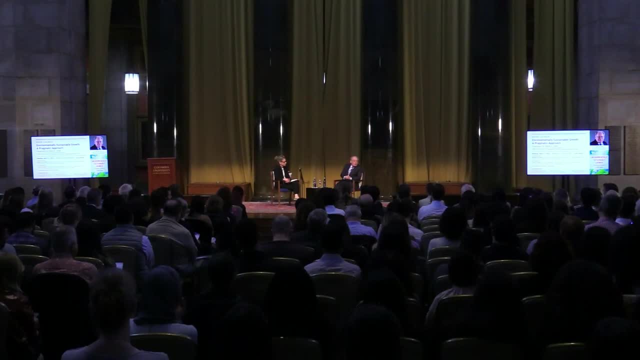 community has put billions of dollars into it, seeing the handwriting on the wall. so that is going to be another thing we're going to see. and the other thing I hope we see in New York City is that we finally get congestion pricing and we improve the subways so that people want to ride. 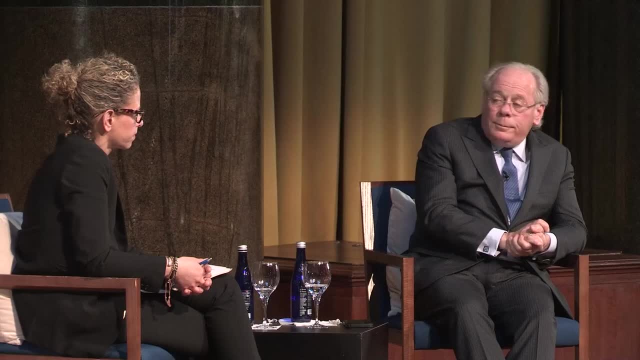 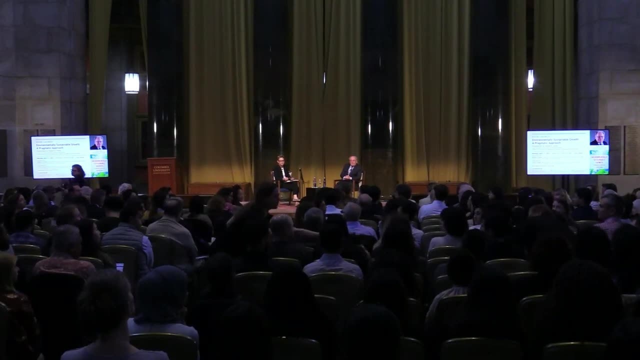 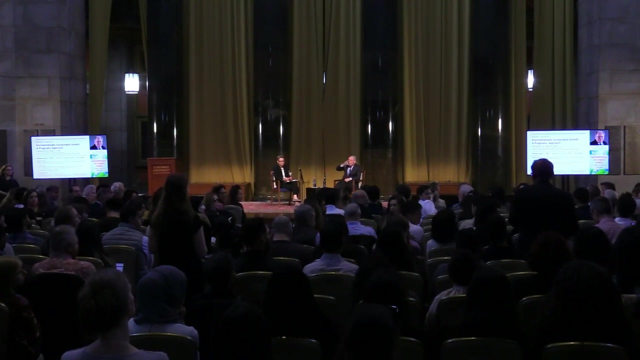 on them and that they're more convenient and come more often, thank you. thank you very much and it's wonderful- uh book it sounds like, and I would like to read it. I had one quick question: that would atomic energy and uh? would that have a place in the way you are thinking? 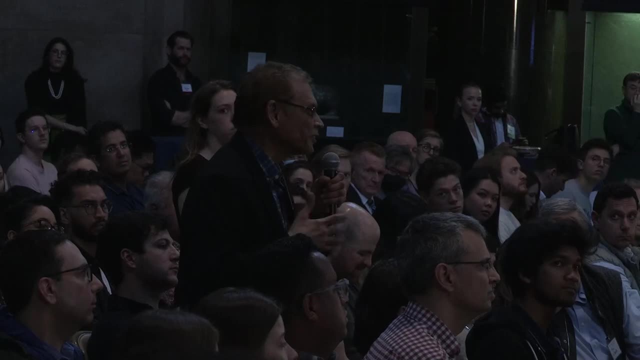 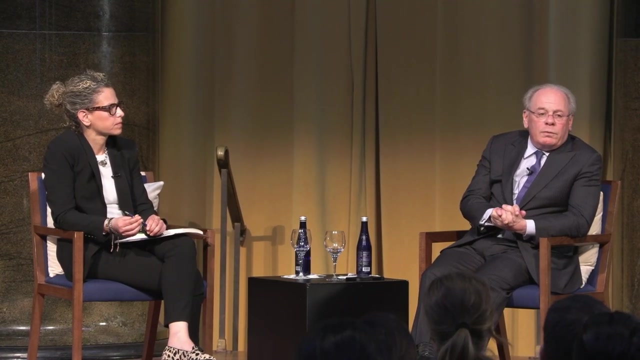 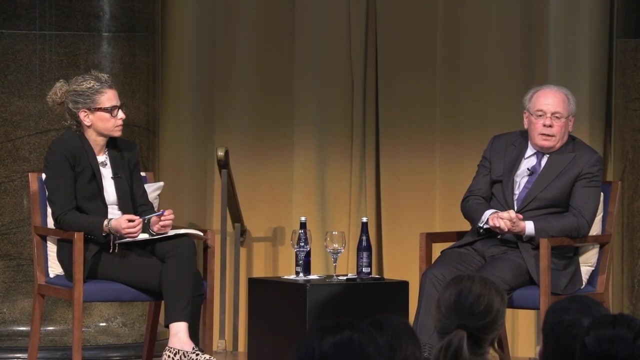 about it and how would it fit- because it may be another way to think about all of this, sure, um, yeah, the unfortunate history of nuclear power is we took the wrong form of it. uh, and it really goes back to Ike as Adamus for peace. we don't want a nuclear power that can contaminate and create. 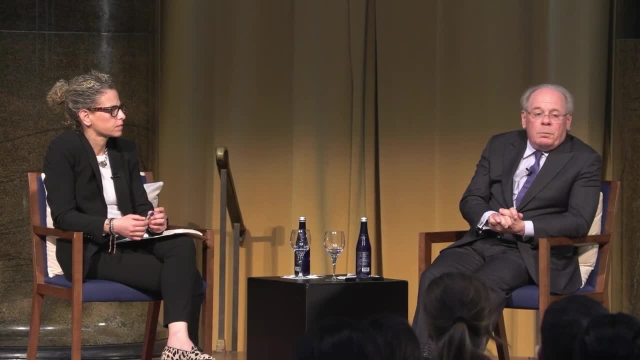 bombs, and that's what fission is. had we put the money into Fusion or other forms of nuclear power would be much further along. I do think that nuclear is a long-term solution, but in the short term I would quote Barry commoner who said: nuclear power, it's a hell of a complicated way to boil. 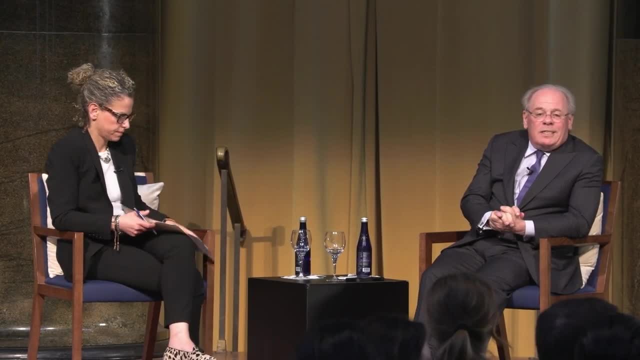 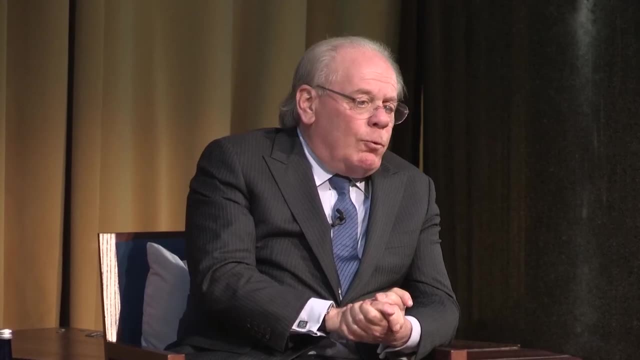 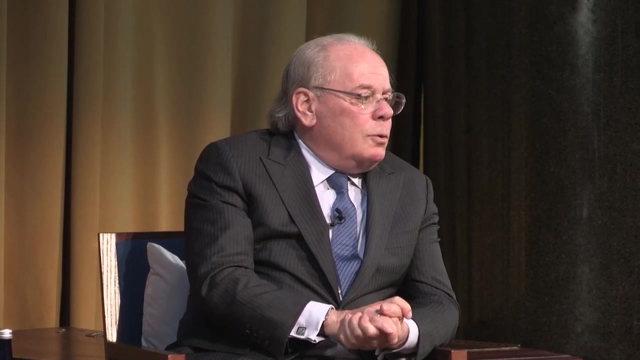 water, and so I think that that the technology of using, uh, some form of nuclear power, yes, the form we have, no. and all of the people that talk about that, I mean: look at what's going on right now in Ukraine. do you really want to have the possibility of a nuclear plant bombed and melting down? 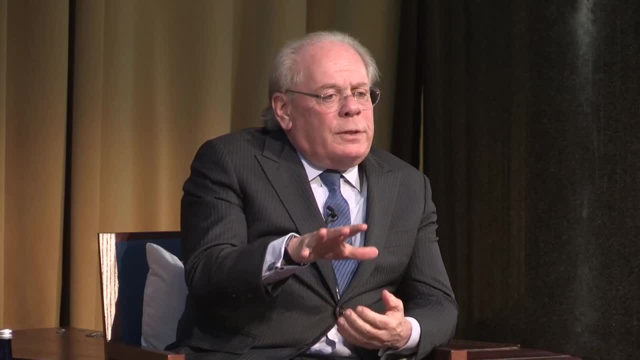 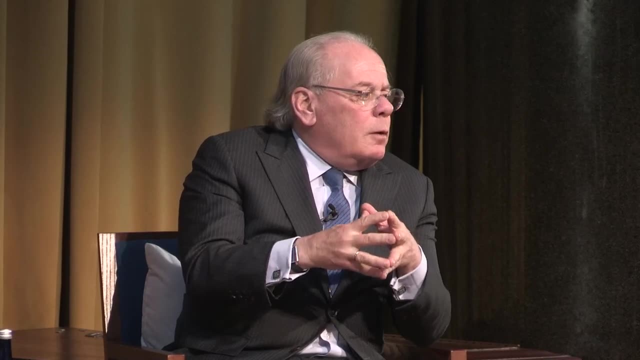 uh, or terrorists taking over. you know, one of the points that I make in the book, which I I should have made here, is that One of the reasons we need economic development is that political stability requires it, And so if the extreme poor people of the world 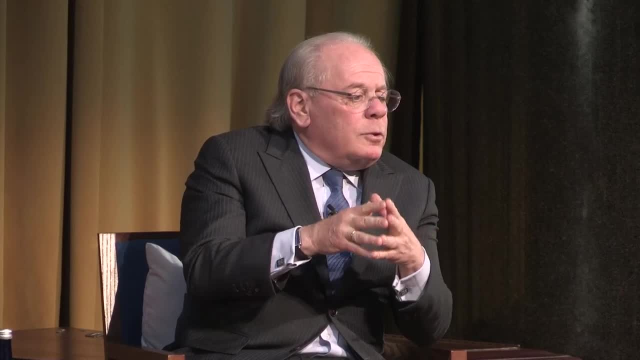 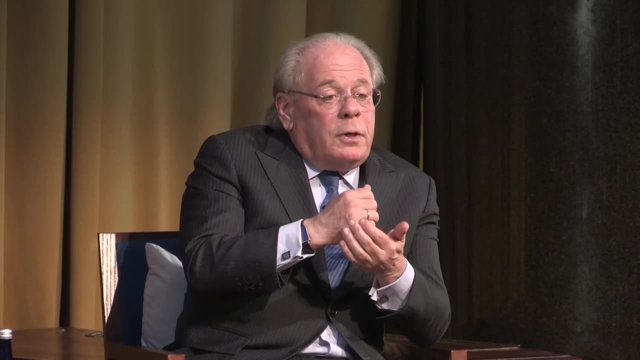 don't see hope, and if the people living prosperous lives think that they're going to lose it, then you have political instability. If you have political instability, you have terrorism. Today, with the technology of destruction, the trade-off is a little sea level rise. 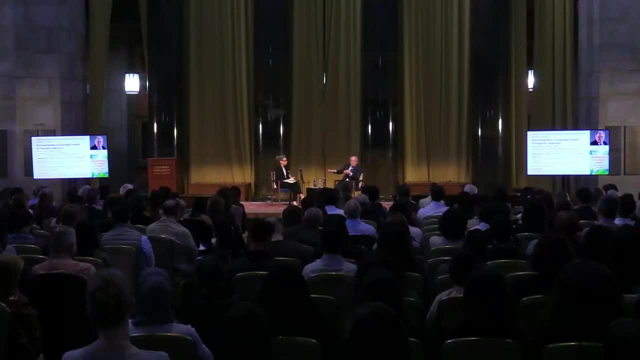 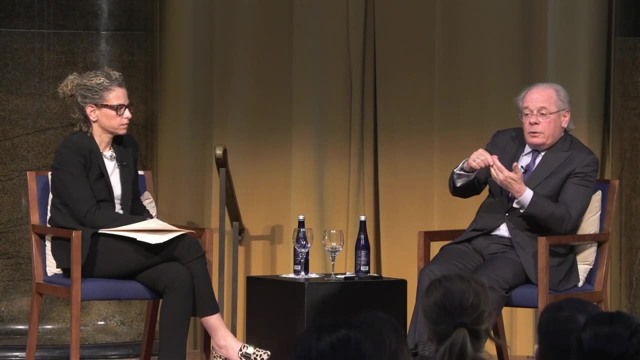 or a dirty bomb in Times Square. I'll take the sea level rise Now. in the long run I don't want either of them, But I think we need to understand the connection between economics and politics and environment. This is one system. 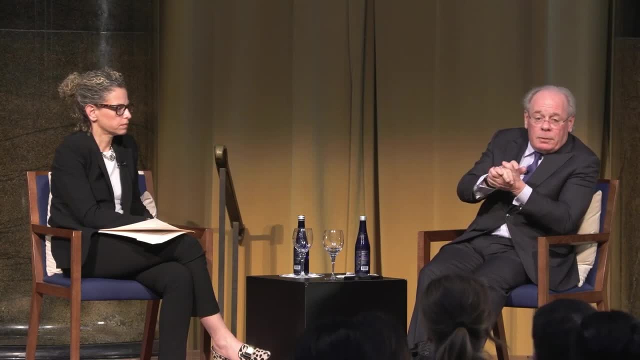 And the idea that you could pull something out and say: let's shut down the economy so there's no greenhouse gases is a dangerous idea and one that's been rejected by politics for good reason. Thank you. Next question: We have someone back on the right side this time. 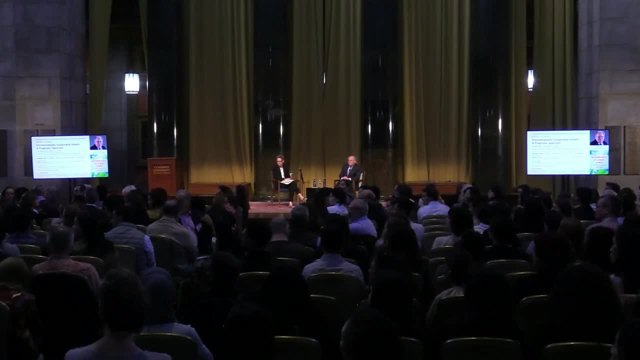 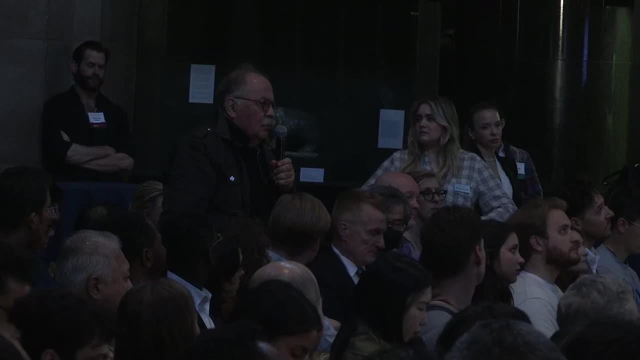 Thank you very much for your efforts. Looking at the electric vehicle, there's a major problem which I'd like you to address: the fact that there's several billion petroleum-based engines in the more than 190 countries of the world, most of which do not produce these vehicles. 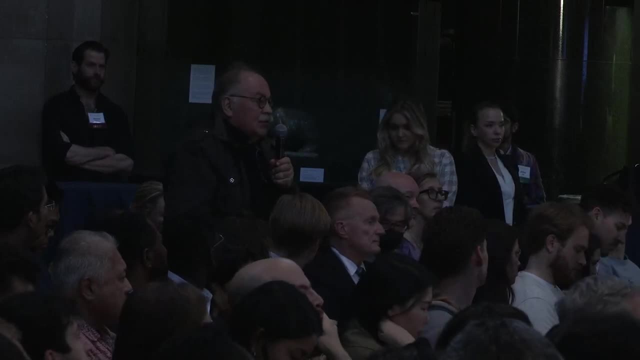 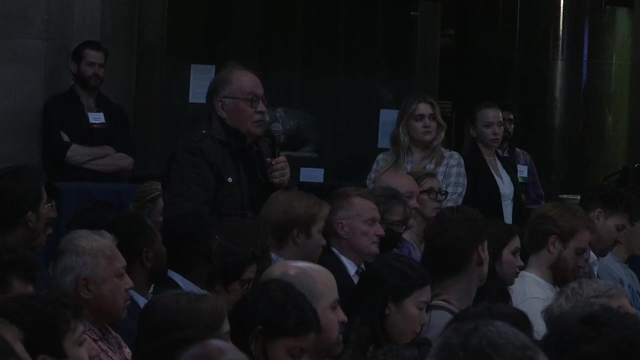 but import them secondhand. And of course, the electric car is great, but you have to ask yourself where does the electricity to run it come from? If it comes from a coal-fired factory, there's a self-delusion. So how do you address in the timeframe possible? 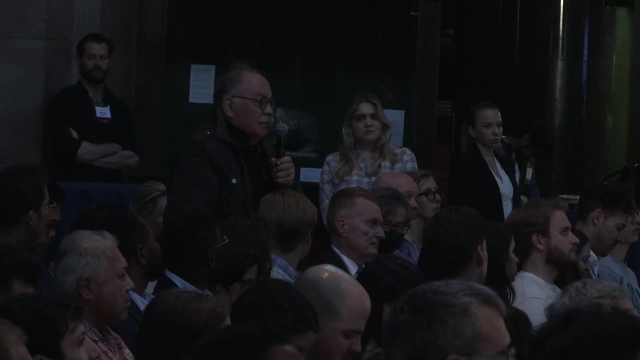 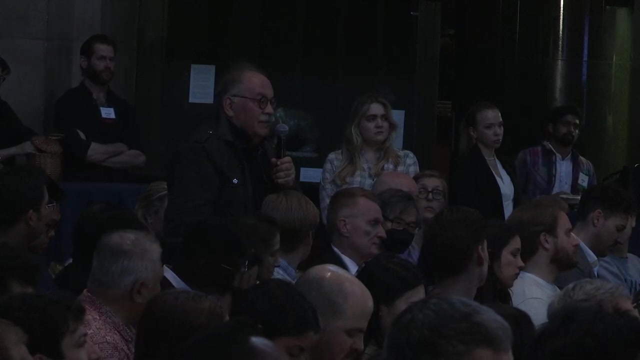 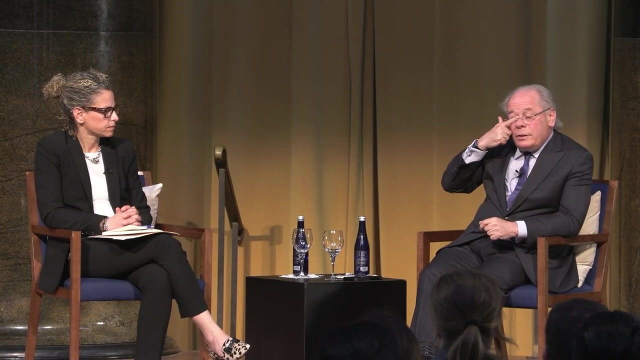 the replacement of those several billion petroleum-based vehicles without transforming them, Because obviously they can't be replaced by electric cars within the timeframe that we're talking about, which is 10 years or less. Well, that's why the goal of 10 years is probably unrealistic. 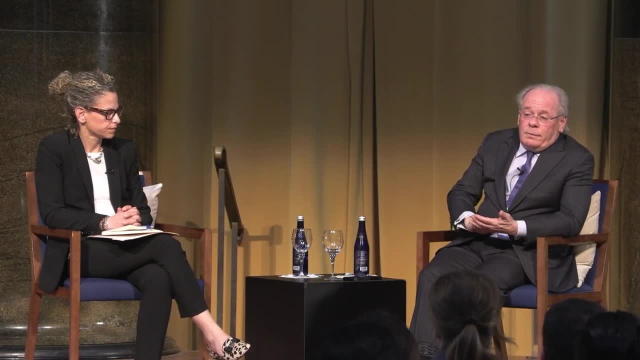 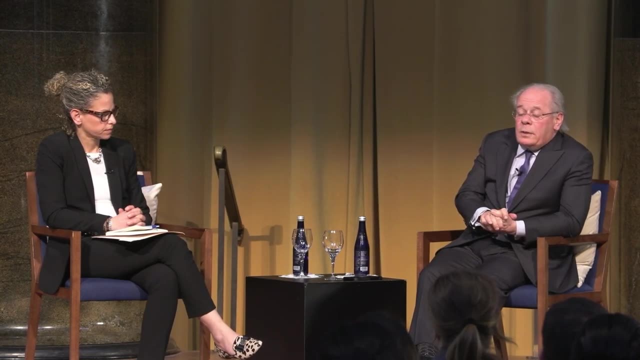 We're talking about a generation-long change And we're going to have internal combustion engine vehicles for a long time. The question is what's going to be the mix And also, as you said, how many of those electric vehicles will be powered on solar energy versus fossil fuels? 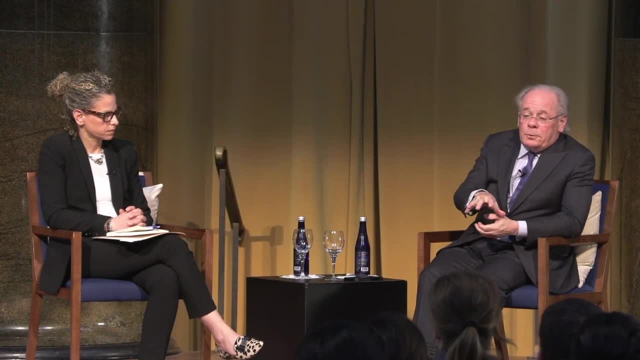 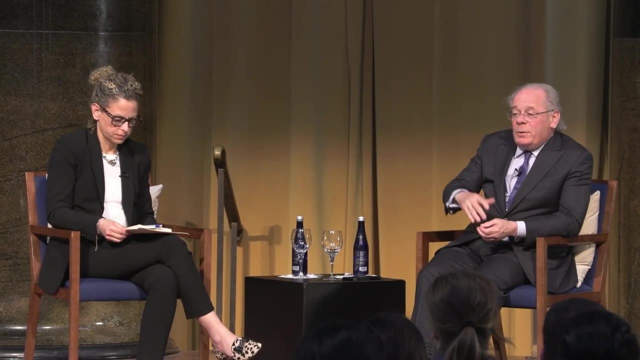 So I think in order for us to get off of the fossil fuels in transportation, we have to get to the electric vehicle. In order for that transition to be helpful to the environment, we have to get to renewable energy. So these are two separate transitions. 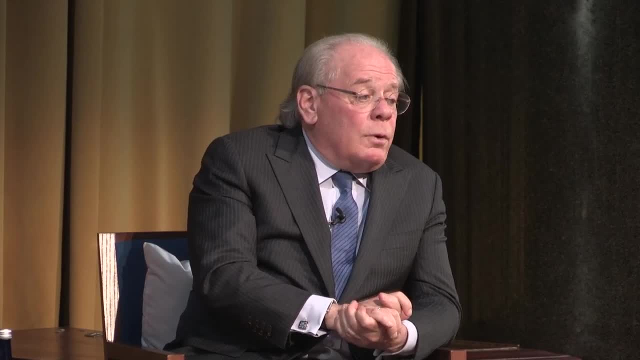 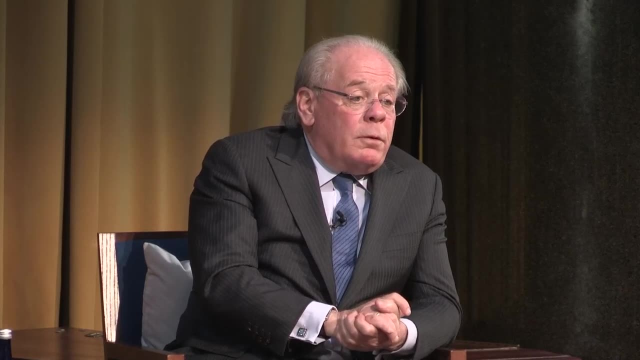 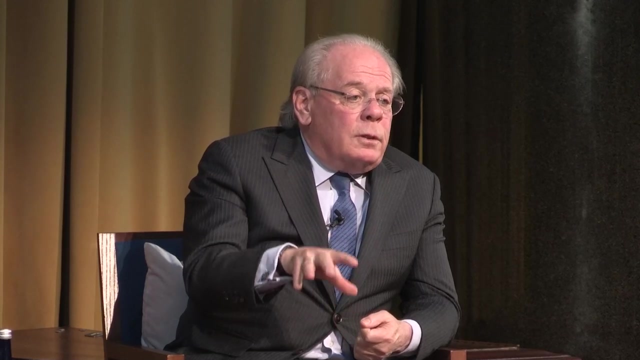 that have to take place simultaneously, And sure all of the old cars that nobody here is going to use will go to other markets, And it's going to take a long time before all of this goes away. I think part of the transition is when solar energy. 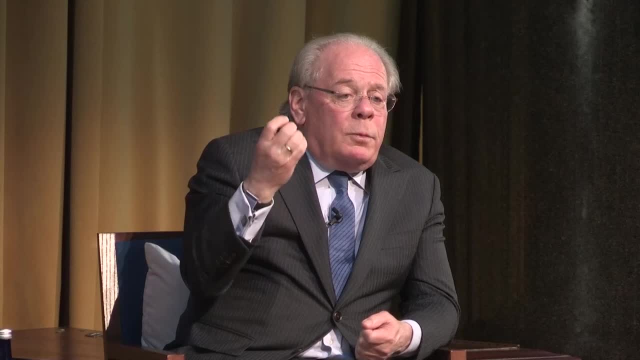 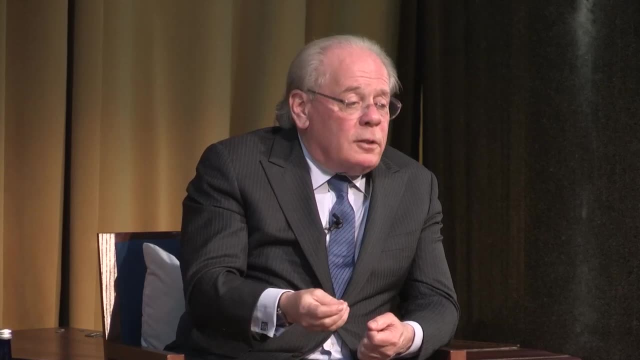 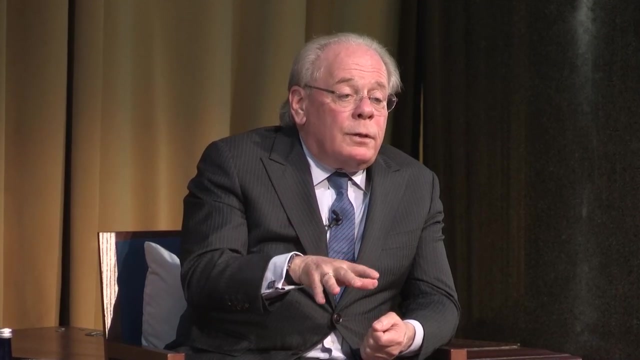 and the batteries that store it become so inexpensive and so technologically superior that it's literally so much less expensive than fossil fuels that your old internal combustion engine vehicle is really not worth maintaining, Because the electric vehicle is cheaper and better, And this is not an instant transition. 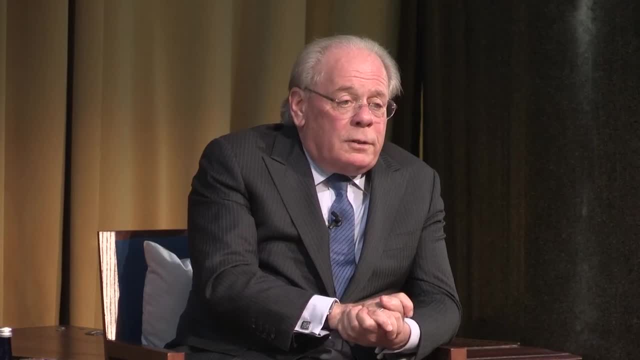 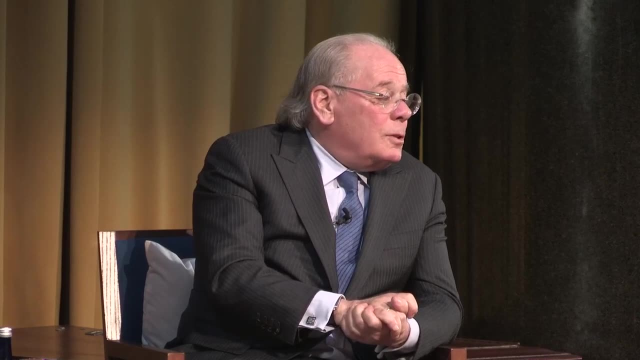 Electric vehicles now are expensive, Charging is inconvenient And a lot of the electricity is coming from fossil fuels. But you've got to make all these changes And you have to start somewhere, And I think one of the biggest and most difficult transitions is going to be the vehicles themselves. 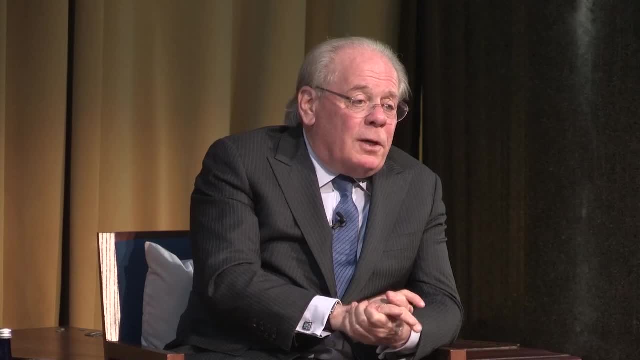 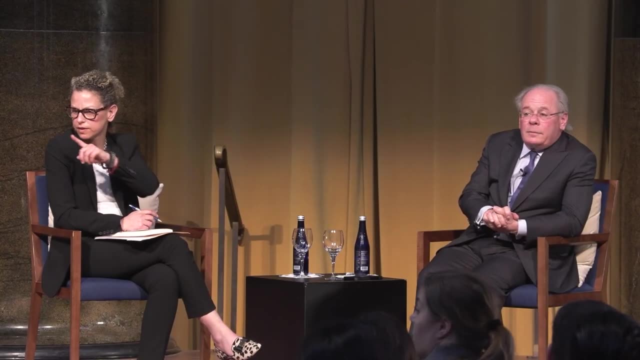 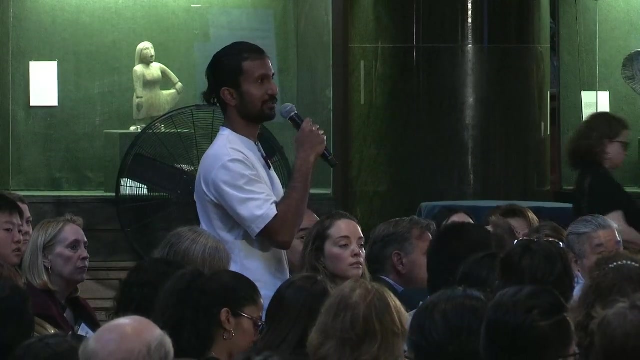 But there's other forms of greenhouse gases, by the way, besides carbon dioxide, And we have to work on those too. Thank you, We have time for another question And this will be the last one. Thank you, Hi. You mentioned that there will be more CSO roles in organizations. 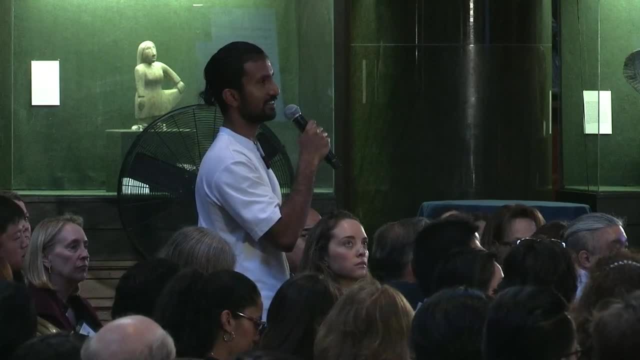 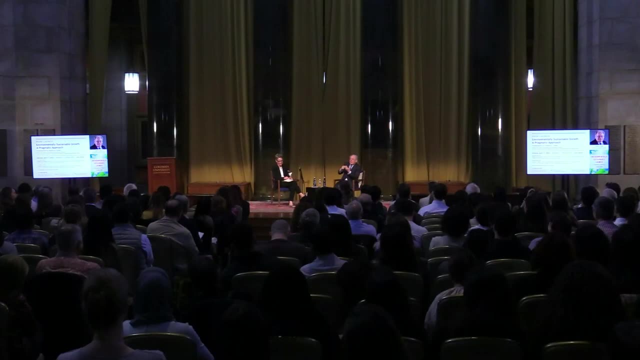 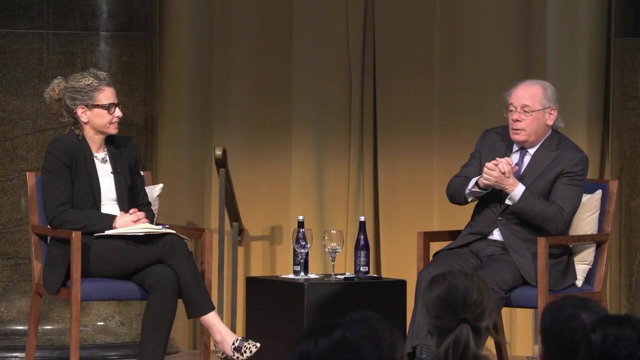 What would the skill set of a great CSO look like? Well, you either get the Masters in Sustainability Management, the Masters of Sustainability Science, or the MPA in Environmental Science and Policy. You could do the MA in Climate and Society if you weren't that analytically oriented. 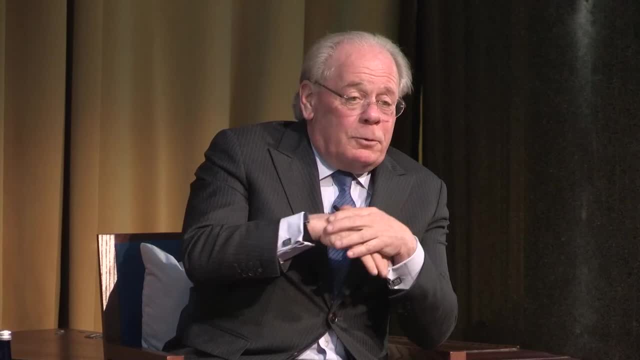 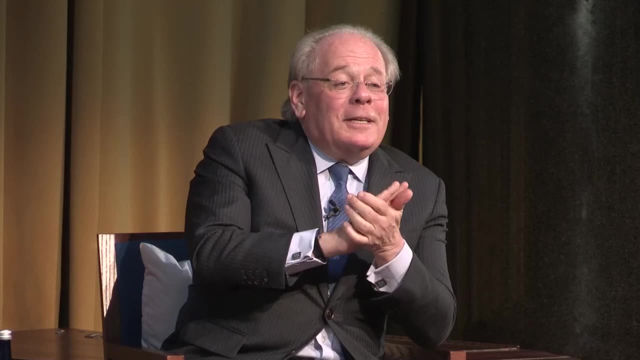 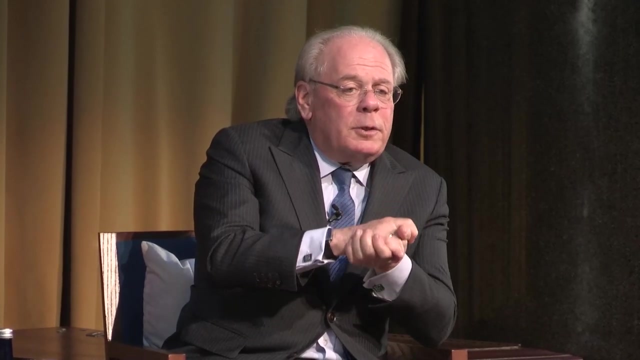 or management oriented. That would help too. Columbia offers a vast array of degrees, most of which I spent most of my academic year trying to sell, So I think we have some of those, But I think that a lot of today's sustainability professionals 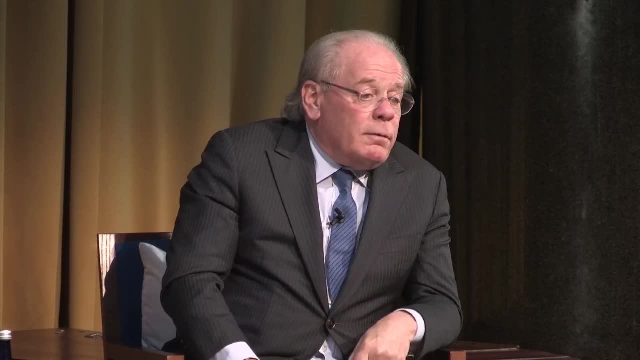 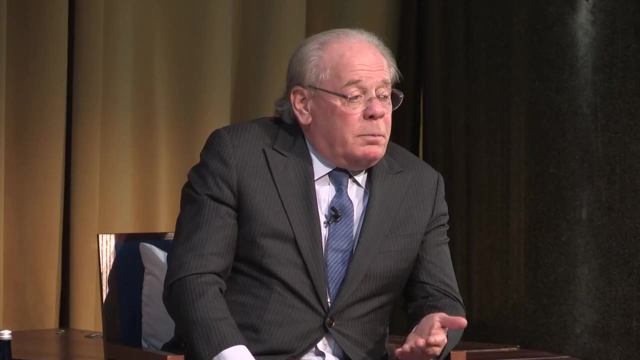 had to retool themselves. They didn't have the formal education that we offer here, And they've made an incredible start in getting this underway. In fact, many of those same people teach for us as practitioners because they have so much to offer. 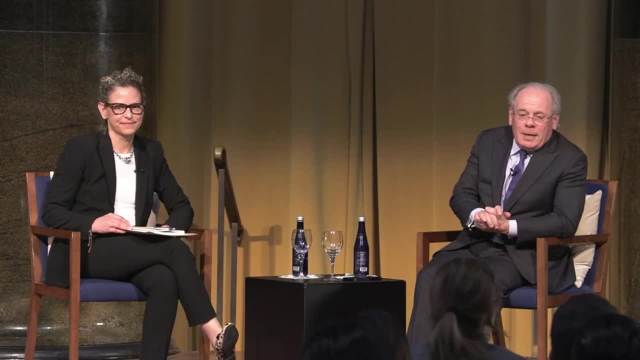 So those would be the skill sets. Anyway, thank you all for coming out tonight. Thank you, Steve.